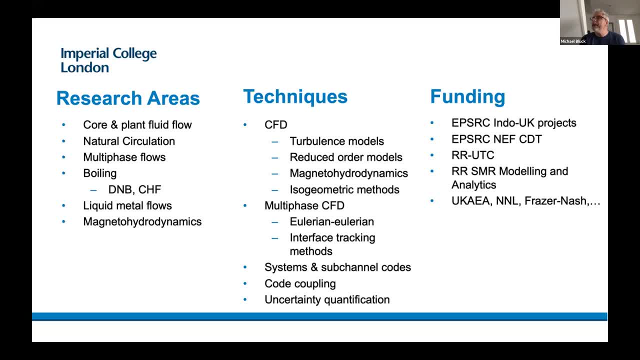 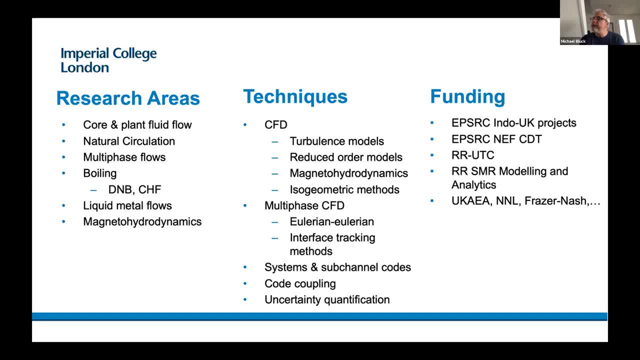 we're looking at a range of techniques. we've been doing that for a while now. we're also looking at a range of techniques- we've been doing that for a while now- approaches and interface tracking methods, systems and sub-channel codes. so 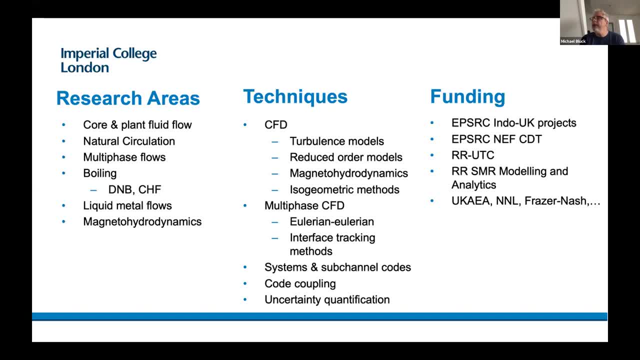 sort of 1D type approach for entire plant and core analysis, code coupling, particularly between CFD and systems and sub-channel codes and across all of that, really uncertainty. quantification plays an important role And we're funded through a number of mechanisms. 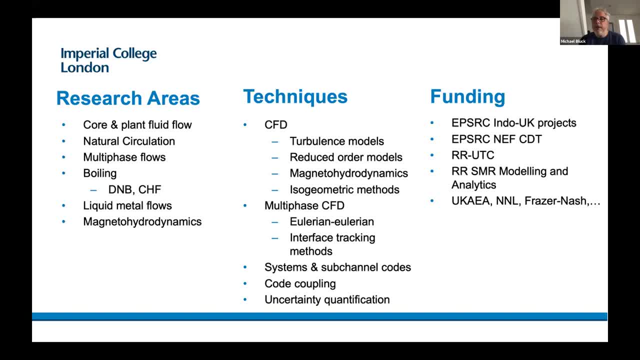 not in any particular order, but we're heavily involved, as others on this call are, with the EPSLC Indo-UK activities. We're also involved in the CDTs. We host the Rolls-Royce Nuclear UTC, the Imperial College, under that anyway. 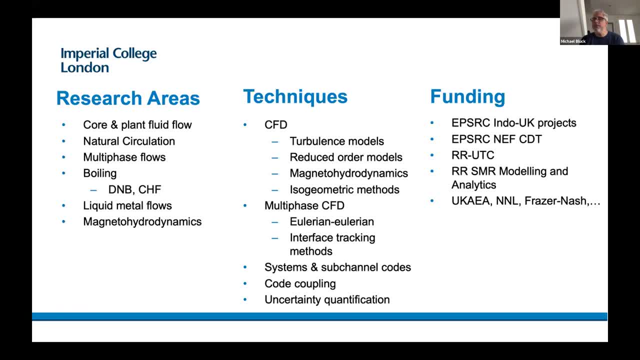 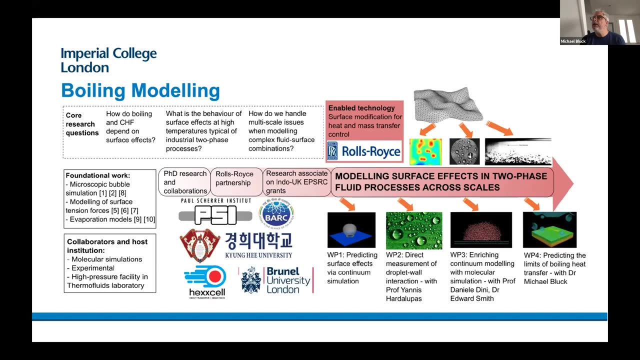 We have activities in the SMR program for Rolls and we also have activities and funding through a few others mentioned there: UKAA, NNL, Fraser National and a few others. So just a couple of very brief words. I don't wanna go over. 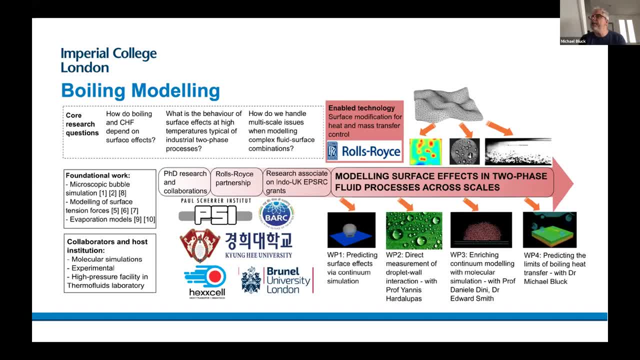 Boiling modeling- this is some of the work that I mentioned. Giovanni Giustini, involved in This, is really looking at very detailed modeling and boiling from inception through to growth and development And attachment, and that's an activity that we're coupling with molecular simulations. 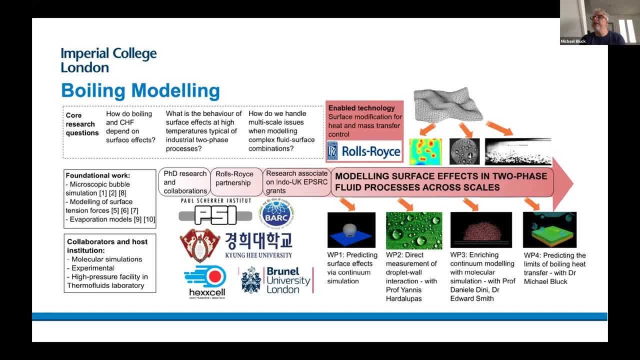 of the processes near the surface through to the continuum level and really looking at the effects of surfaces on that. So we're really coupling the materials almost with the fluid processes. So that's a bigger and growing area that builds on a lot of our boiling work. 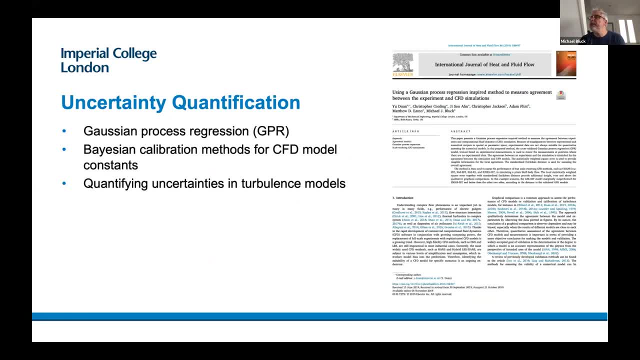 that we've done over many years: UQ, Uncertainty Quantification. that's another big activity that covers quite a lot of what we're doing now and it's growing. Gaussian Process, Regression Methods, Basing Calibration for determining constants- whatever we're doing, certainly unless we're doing DNS- 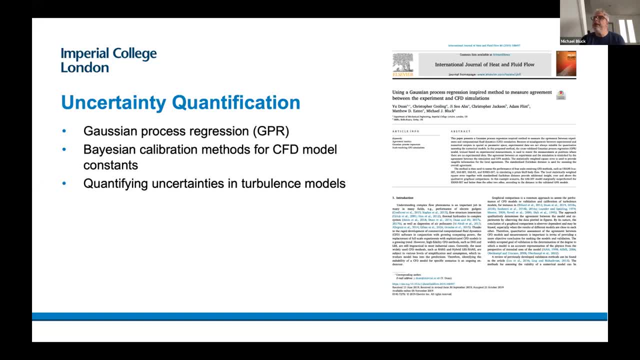 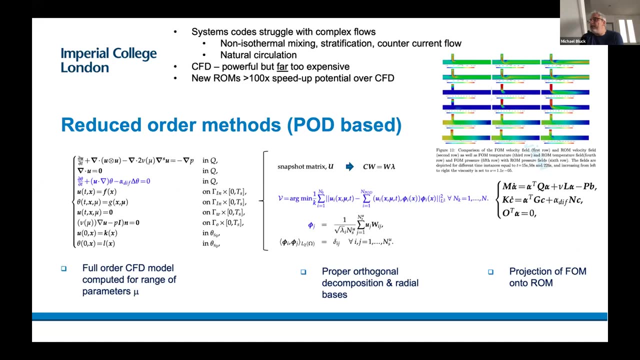 then constants are involved. So determining those and quantifying uncertainties in turbulence models and a whole host of work involved UQ. I'm only picking one or two of the things. I'm not going to go through a whole list. Reduced order methods again. 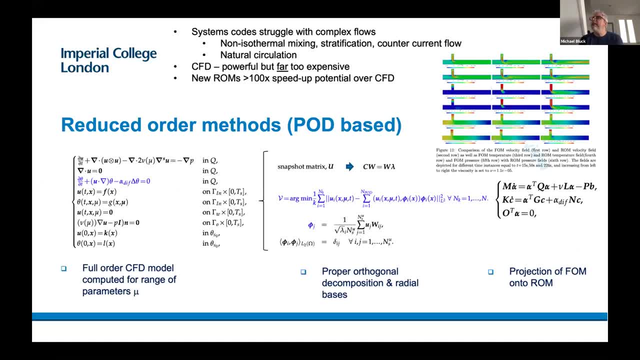 we haven't got vast supercomputing resources, then the requirement- our approach, if you like this side of the pond is at least- is looking at reduced order methods, particularly pod-based methods, where we take full order models and we do a proper orthogonal decomposition to reduce order. 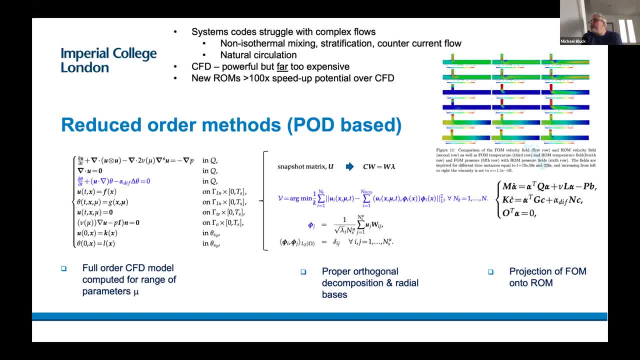 So that's one of the things we're looking at. The other thing is we're looking at how to reduce the cost, at some limitations, obviously, and we've done a lot of work on that in collaboration with a group in Italy, TRIES. 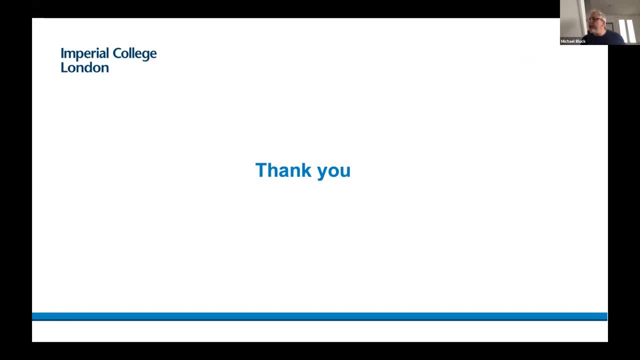 And I think I'll end it there. There are obviously others, but I think five minutes. I think that'll do, if that's okay. I don't know if I'm good. Thank you, Mike. Yeah, you can stop sharing, then the next one can share. 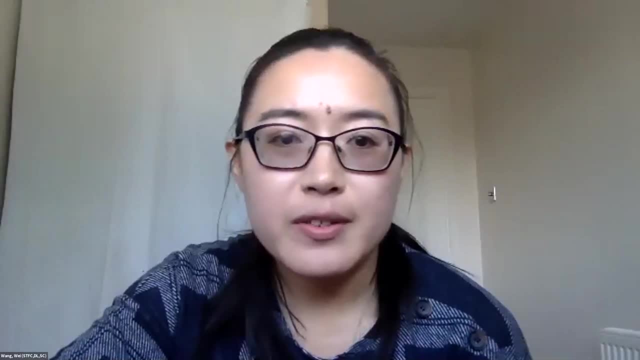 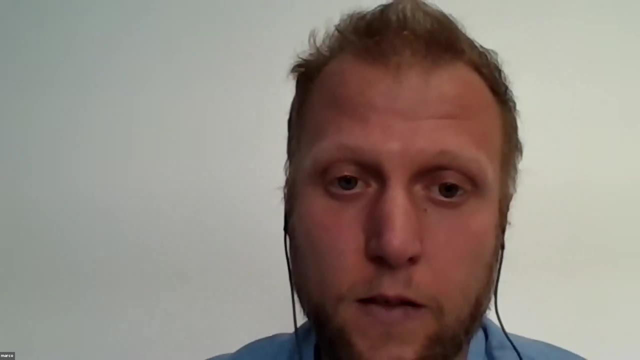 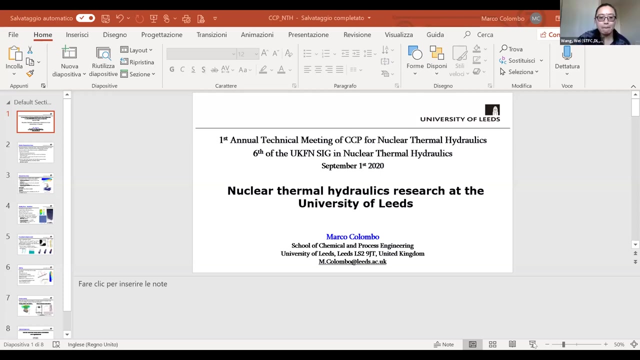 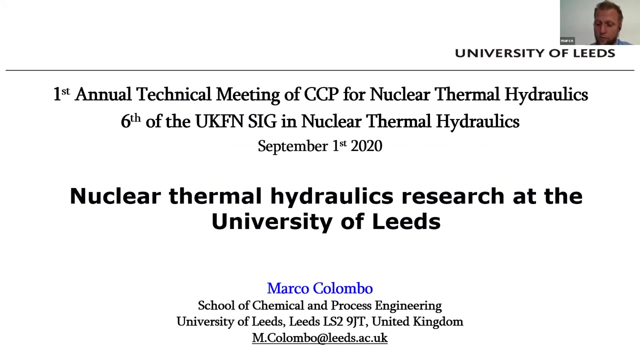 The next one is Marco from Leeds University. Okay, good morning everyone. Let me share my screen. Can you see it? Yeah, Okay. So yeah, we'll try to go on a brief overview of the thermonadolics activity at the University of Leeds. 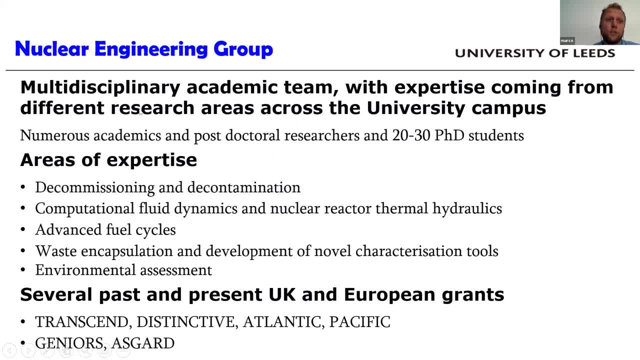 First of all, that is part of the nuclear engineering group, which is based in the School of Chemical and Process Engineering, but is a really multidisciplinary team that has expertise, other than in thermonadolics, also in decommissioning, decontamination, waste management. 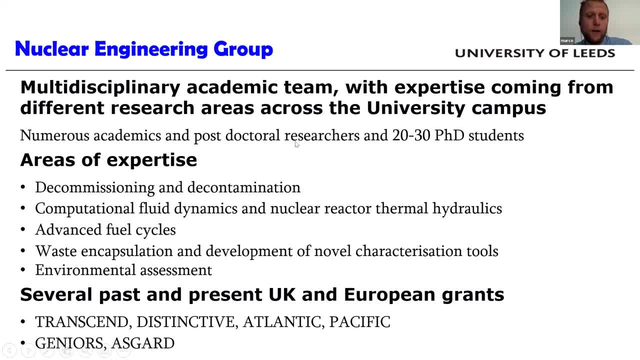 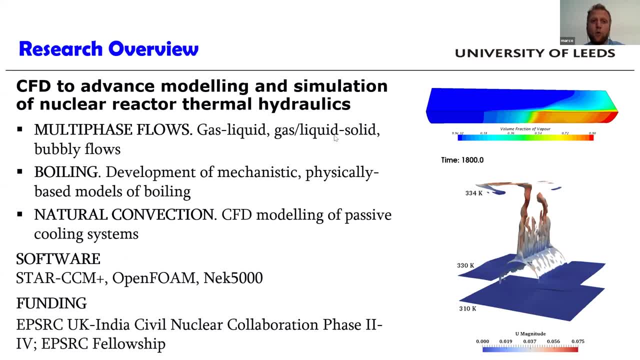 and in advanced fluid cycles, and has been funded with several grants from the UK and also Europe, present and past. So with regards to the thermonadolics activity, yeah, First, we use computational fluid dynamics to advance our modeling capabilities in different aspects of nuclear thermonadolics. 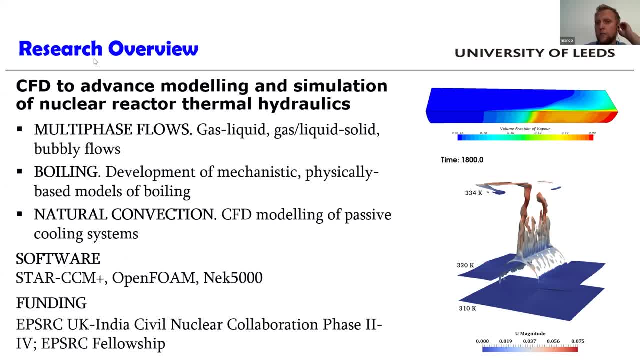 and our main expertise are in multi-phase flows, in particular gas liquid, but also gas or liquid with solids, and specifically also on bubbly flows, And I will show some results on those And then the deodorant and multi-phase flows. 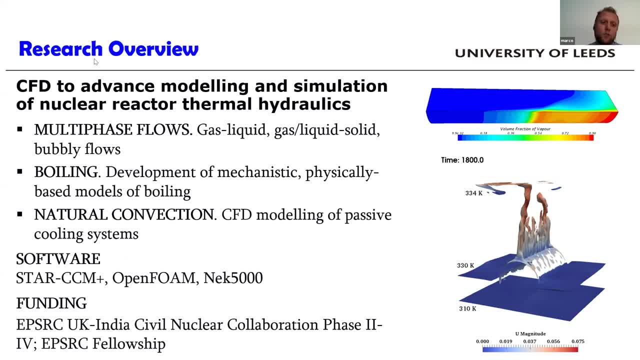 where we really focused on in boiling, and also we apply CFD to natural convection and passive safety systems in the context of nuclear thermonadolics. The software we use are mainly StarCCM Plus OpenFOAM and EC5000. 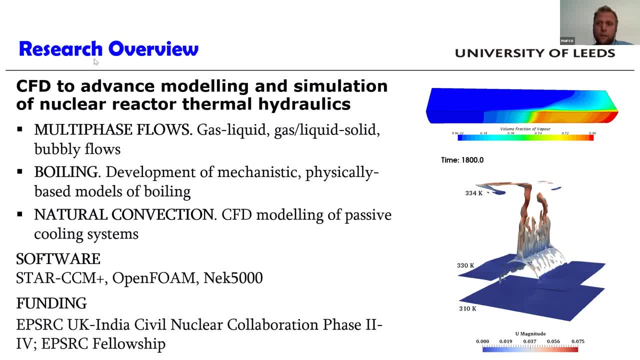 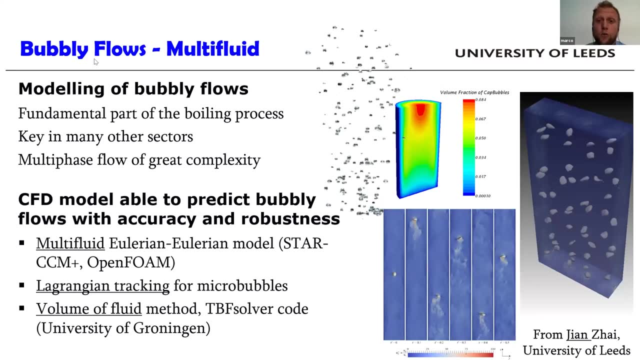 Those are the software we are experienced on and the activities have been funded through different EPSRC grants, mainly on the UK-India-CV nuclear collaboration and also the fellowship that I currently hold. So, with regards to bubbly flow, we are interested in modeling those. 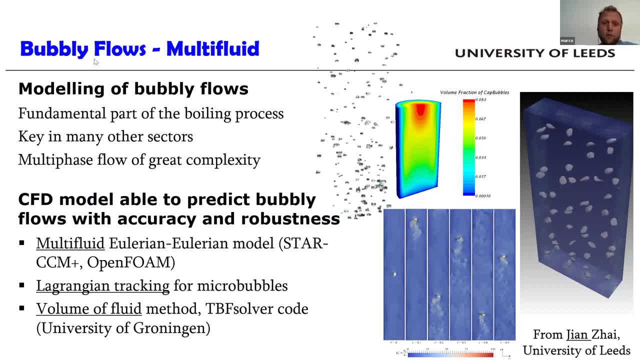 in the context of nuclear, because they are a fundamental part of the boiling process, but also because they are relevant in many other sectors where we require mixing, And that is also a fundamental part of some reprocessing techniques. We use different techniques to model bubbly flows. 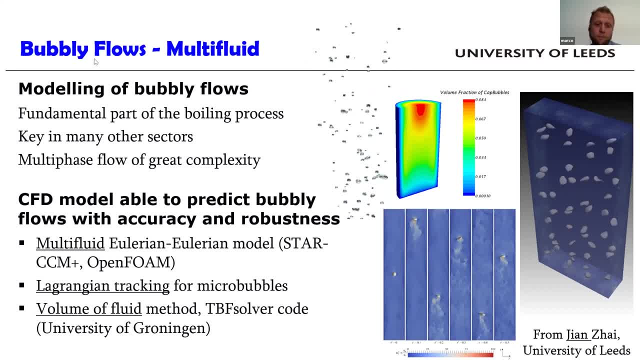 We have multi-phase capabilities with multi-fluid models, So you learn your models mainly using StarCCM Plus and OpenFOAM, but also we use Lagrangian tracking and this has been done mainly for micro-bubbles And we are developing also capabilities. 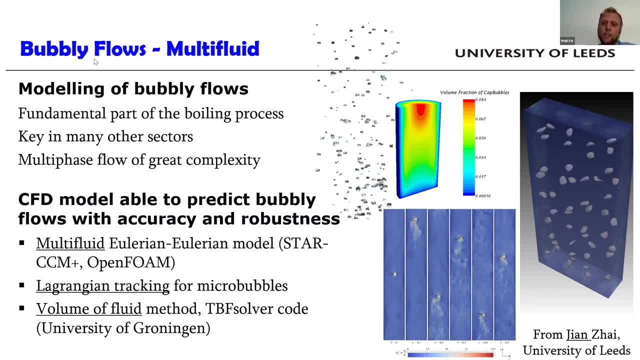 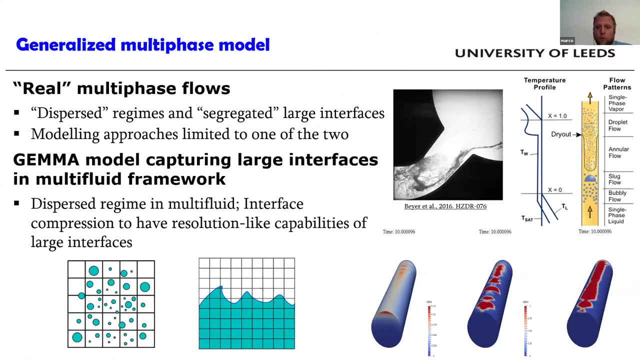 in using interface resolving methods such as the volume of fluid, And you can see some example on the right of a single bubble rising in a channel and also of some multiple bubbles: simulation. This is one of the recent developments, so the development of us. 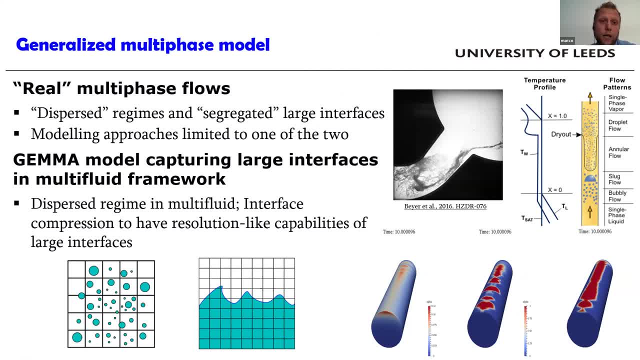 also in the era of multi-phase gas-liquid flows, the development of our generalized multi-phase model that is called GEMMA. that's tied to go beyond the fact that in gas-liquid flows we have multiple flow regimes and most of the time 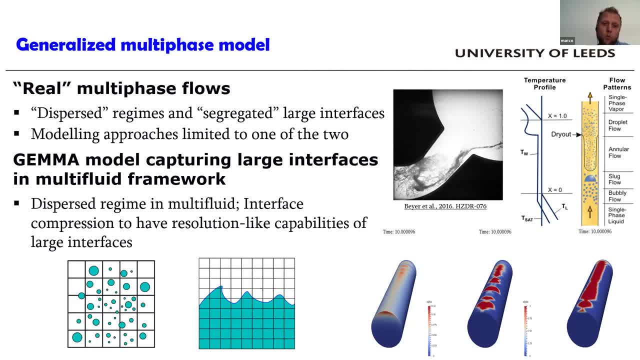 the models at the present time are limited to some of those. So what we are trying to do is maintain the resolution of dispersed bubble or droplets with average methods such as the multi-fluid. so it's a multi-fluid framework And on top of those, 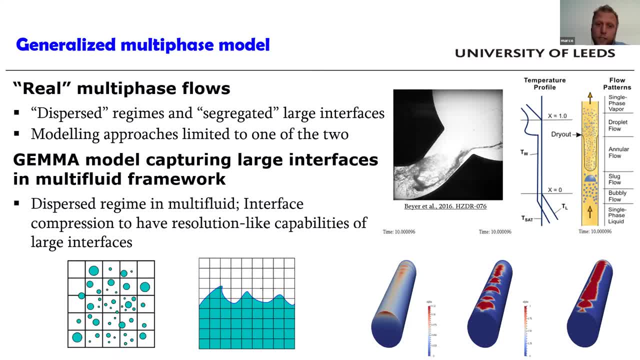 we have the resolution of the large interfaces, only more than resolution, let's say keeping the interface sharp and trying to apply the right close relation. And on the bottom right there is an example of the simulation of a horizontal pipe. So on the left the flow is dispersed, with many bubbles. 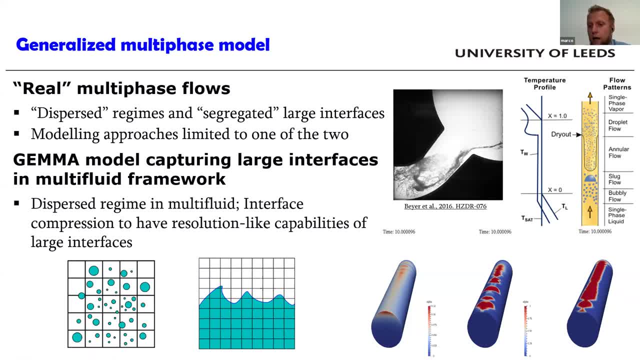 and then the void fraction gets higher on the right and the model starts to detect large gas structures and it becomes a plug And then a slug flow. The shape is a bit strange, but that's because the pipe is scaled in the flow direction. 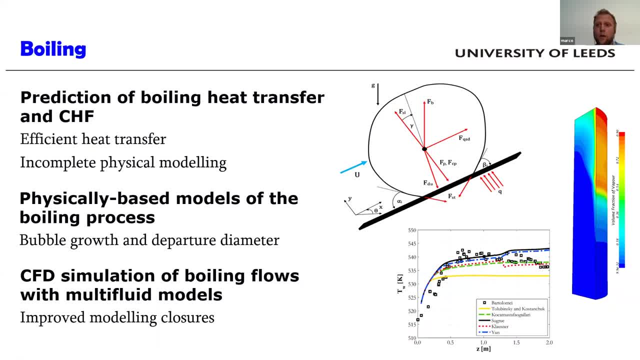 so it's much longer than how it appears. Other than that, we had many activity in boiling. Again, the interest is, of course, the prediction of boiling, heat transfer and the CHF in the reactors. What we do is we try to develop. 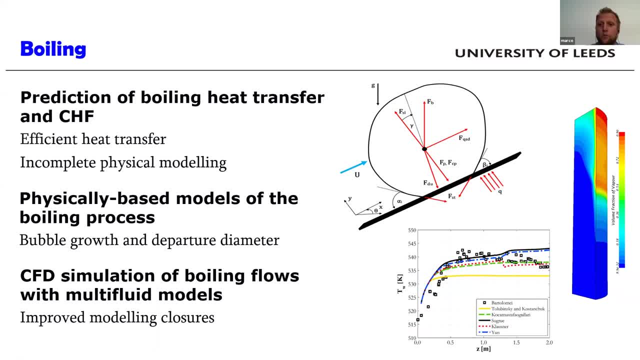 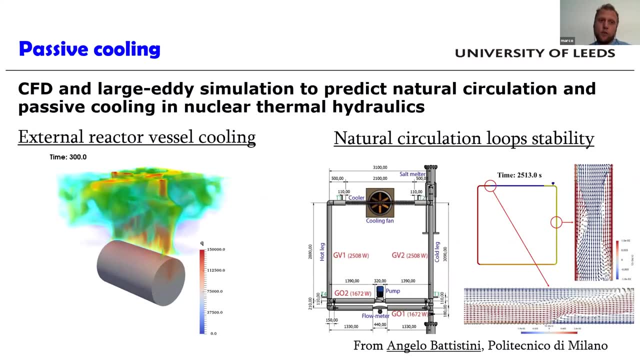 more physically-based model of the boiling process, in particular for the growth of the bubble and the departure, and implement those in CFD and add simulation of boiling flows in nuclear thermal hydraulics. Some of those are in natural circulation and this is the other area we are active on. 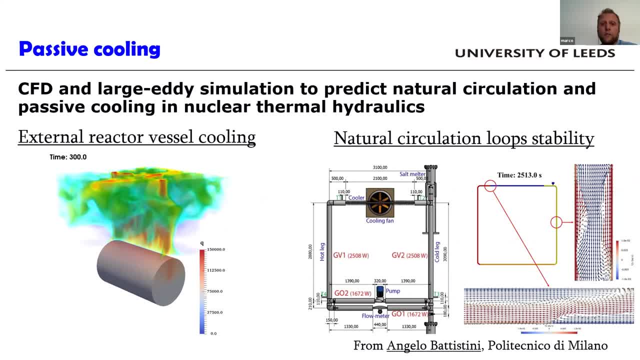 is the passive cooling. So the use of CFD, mainly coupled with large-head simulation, to predict passive cooling and the effectiveness of passive cooling in nuclear reactor. You see two example here: the cooling of the outside of a cylindrical vessel in a water pool. 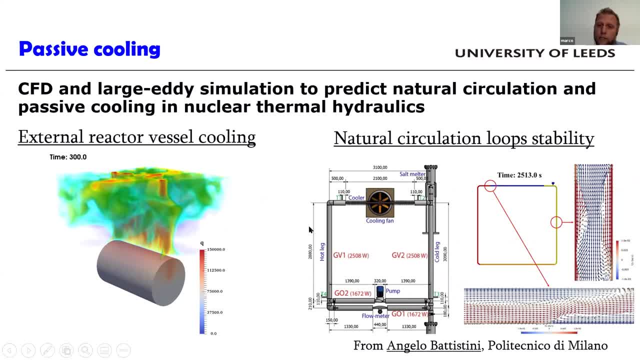 in case of core melting, and also, on the right, the simulation of a natural circulation loop with distributed heat generation. So here the focus is the molten salt reactor, again done with large-head dissimulation. This is on the right single phase. 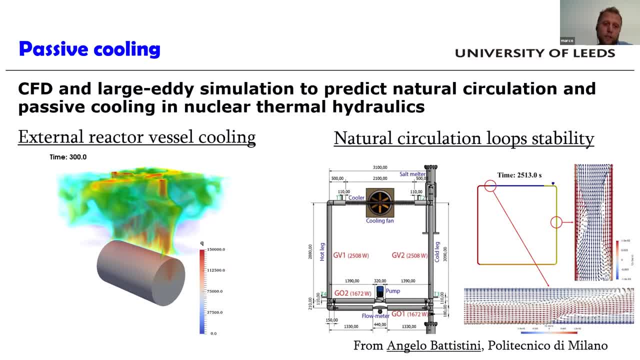 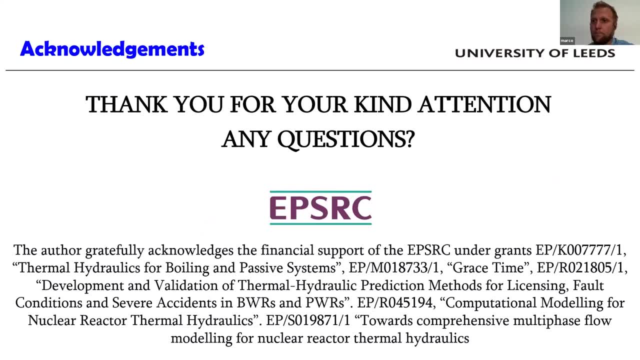 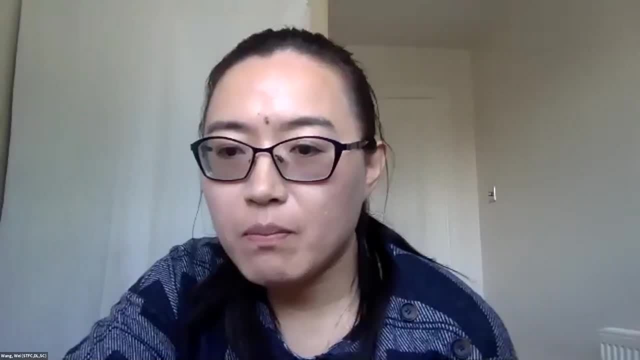 Instead on the left in the external reactor vessel, we also had some boiling on the outside surface. Thank you very much. That was my presentation. Thank you, Marco. The next one is Marcus from Bangor University. Yeah, good morning all. 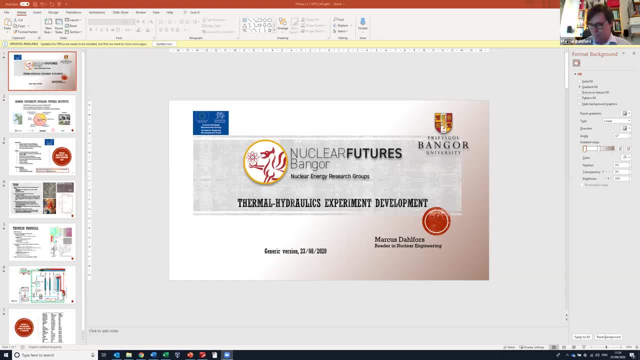 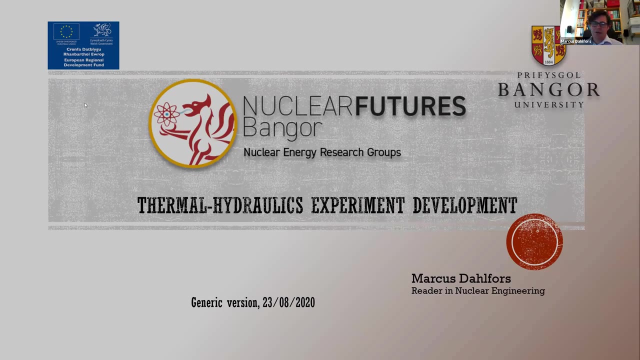 I'll try to share here. Let's see. can you see my screen? Yeah, yes, Get it started as a proper slideshow as well. Yes, okay, Yeah, So I'm Marcus Dalfors, representing the Nuclear Futures Institute. 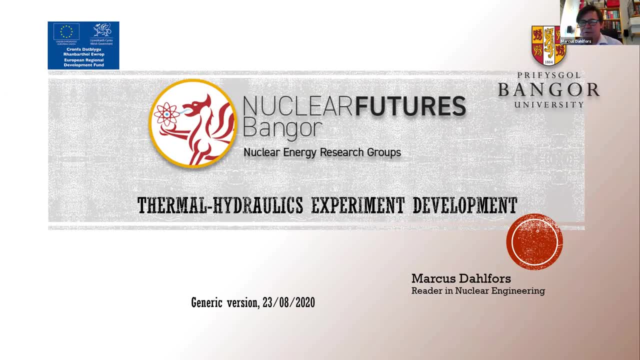 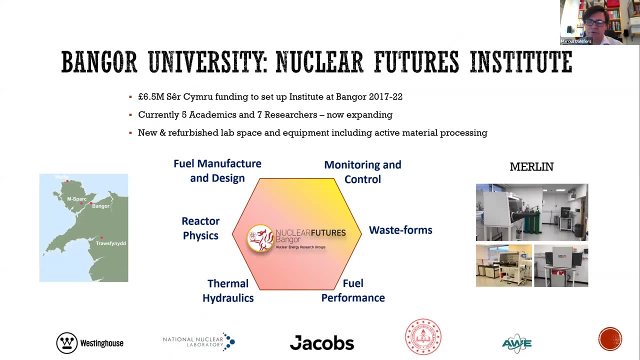 of Bangor University. We're pretty fresh on the arena here in nuclear thermal hydraulics And I want to present to you the background roughly how our institute has reprofiled itself lately. So currently, or let's say we have a fairly solid base. 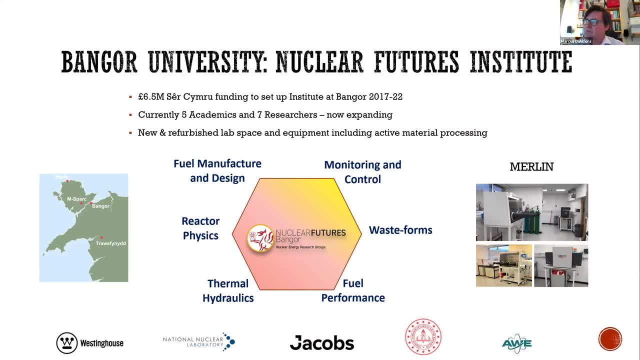 within materials, waste forms, fuel manufacture and design and fuel performance. What I'm bringing to the group is reactor physics and thermal hydraulics and, yeah, probably a little bit of dabbling into the areas of fuel performance and monitoring and control as well. 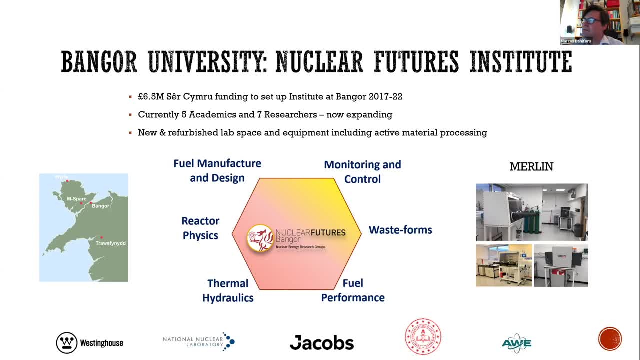 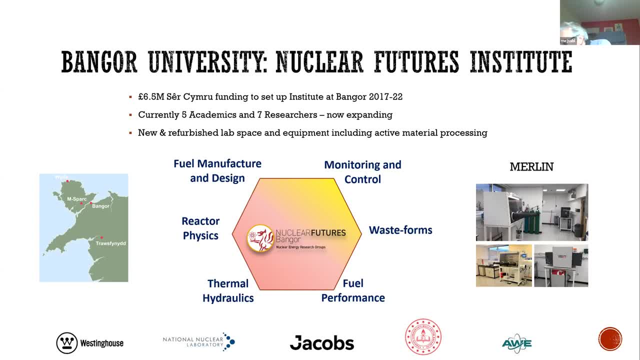 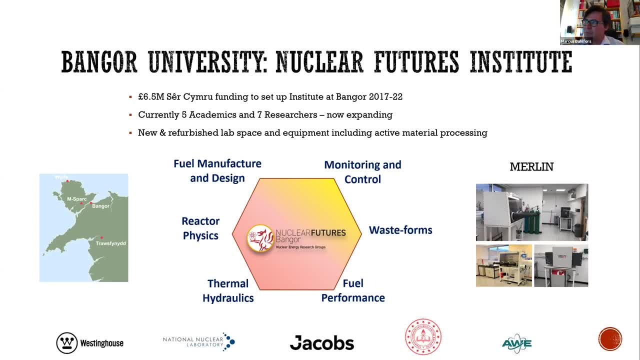 where we are. you see a small map there which points out Bangor and some of the sites for nuclear development that we have in the area. We're funded by a 6.5 million pound CEREC-CUMRI grant And this is running actually now. 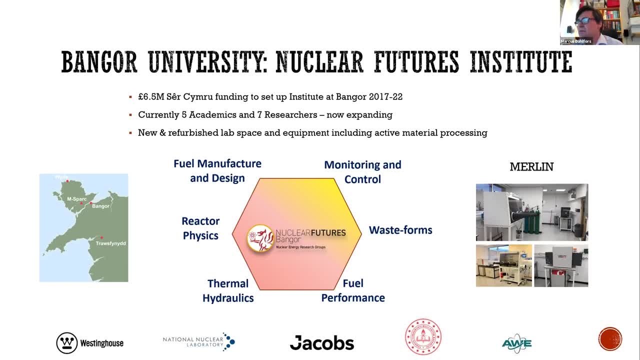 after a re-profile of the funding. It's running until 2023.. We're right now five academics and seven researchers, but we'll be expanding quite significantly, as I will show you on the next page. We have some new and refurbished lab space. 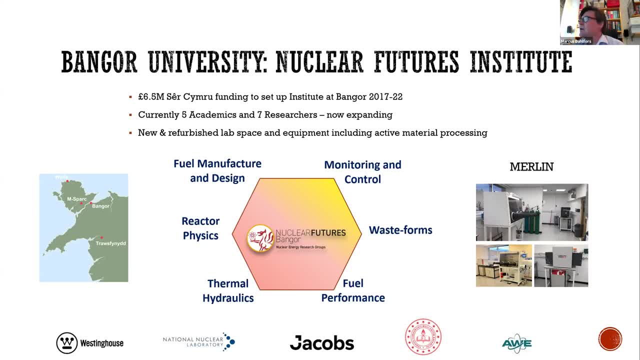 What concerns thermal hydraulics, I'll show you. And then we have quite significant materials, laboratories and actually more proposals in the making on that side as well. The one that we have right now is Merlin, which is a refurbished, quite sizable lab. 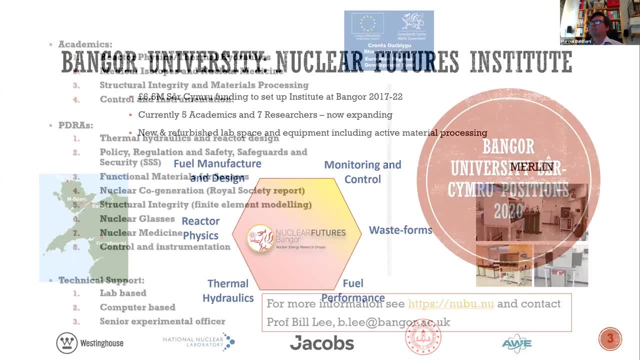 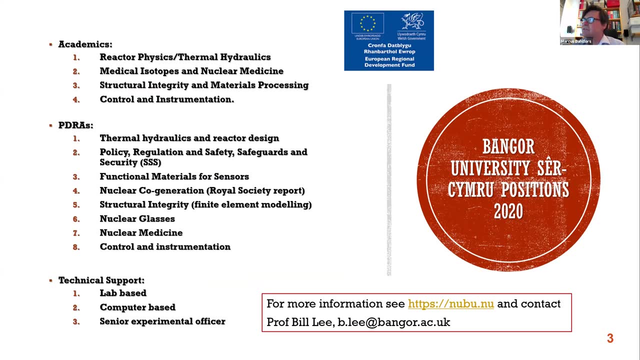 where we can even handle active materials. The recruitment way that we are initiating right now is fairly significant. There will be more information if you. The recruitment way that we are initiating right now is fairly significant. There will be more information if you. 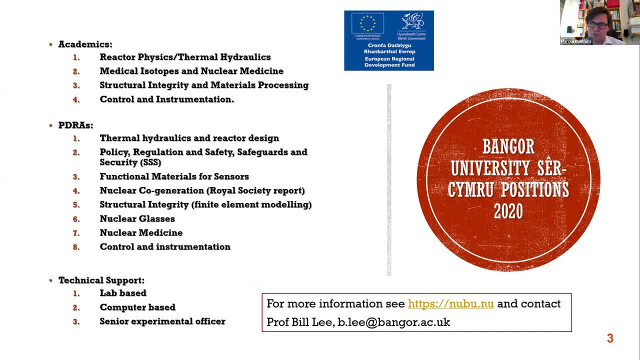 go to our webpage. I'm quite aware of the time limitation, So I will just tell you what will affect the area that I'm active in myself. So I'm looking towards engaging one to two lecturers in reactive physics and thermal hydraulics. 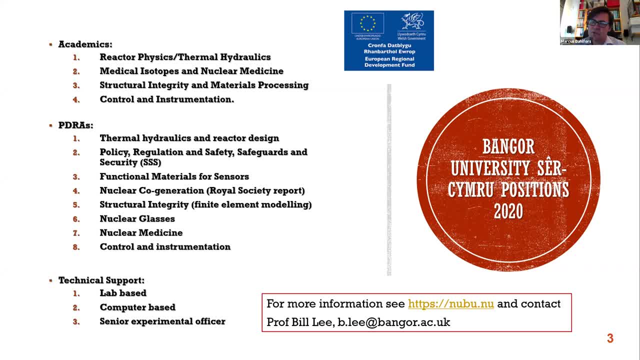 and also control and instrumentation, which will be relevant to the field of thermal hydraulics experimentation. That's where I think our group is fairly complementary to many other groups in the UK, although I know there are others who are active in experimental TH, but we are quite 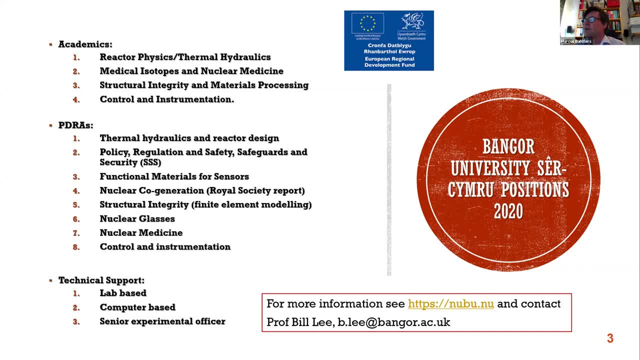 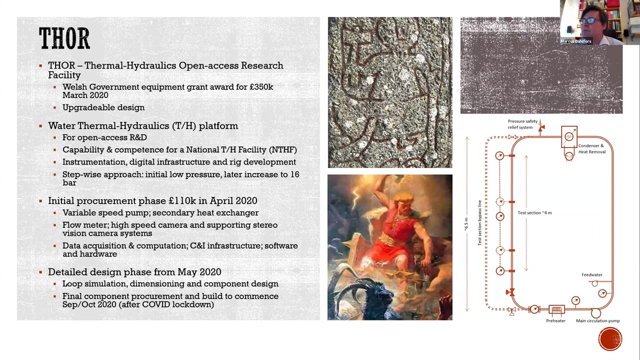 focused on that part of thermal hydraulics. Then we're also looking to engage at least three postdoctoral research associates in these areas as well. Quite importantly, we're getting a couple of technicians in as well, which will be quite significant for the current thermal hydraulics experiment project that we have going. It's 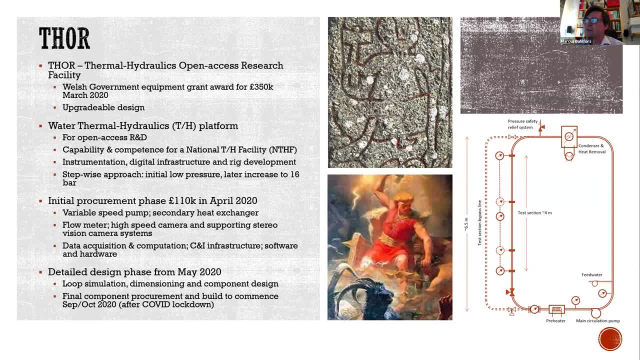 the THOR facility Thermal Hydraulics Open Access Research Facility. We would very much welcome anyone who wants to come and design experiments and carry out on our rigs. I would refer to said web address and please don't hesitate to get in touch if you have ideas. 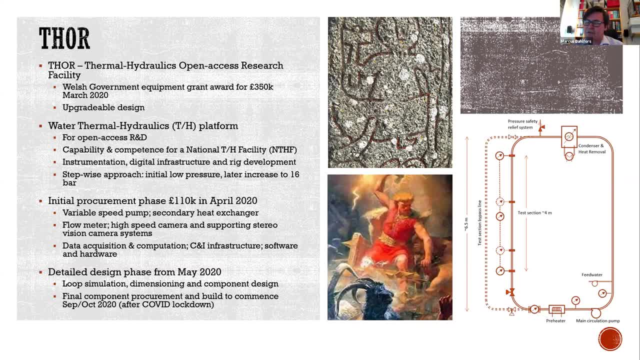 This rig has a very simplified diagram to the right showing what it's roughly about. There are a few things missing there, but it is right now in detailed design and construction is to begin next month. We have done some initial procurement and are well on our way. 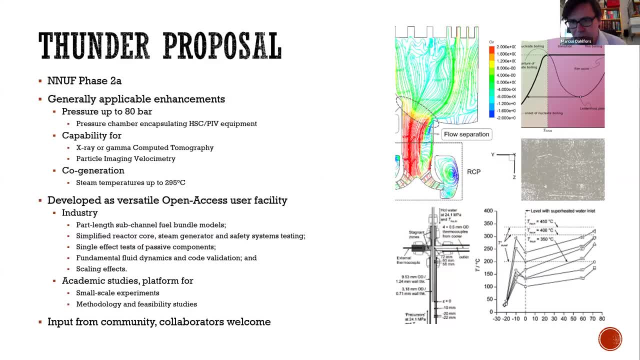 But I want to turn my focus to actually a proposal. due to the recent national nuclear user facility, call the phase 2A of it- We have developed actually an upgrade proposal, so THUNDER, which is the thermohydraulics upgraded and enhanced research facility. 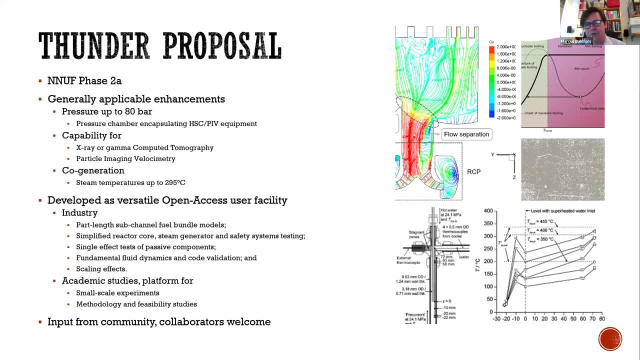 And this would basically build on a similar concept, but where we would take up pressure to 80 bar with a very low pressure, And this would be a special feature of a pressure chamber that can accommodate large window access to thermohydraulics experiments inside of it. 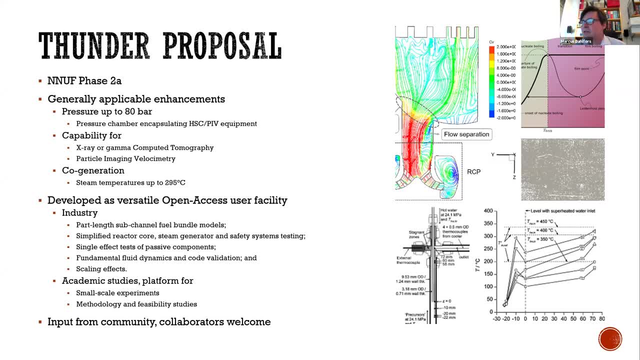 For geometries of quite significant extent. we are looking to maybe a 2.5 meter high and 1.2 meter pressure vessel where we would have pressure recognition. Maybe we can just go for a medium diameter maybe, but if we could do that, 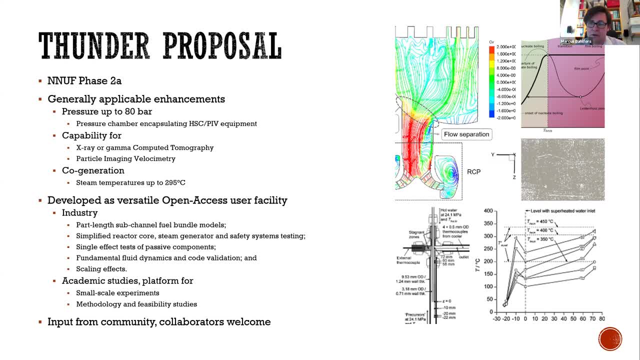 we could have a helping of about 5 to 10 meters and would be able to have the double-walled temperature. So this would be, I would say, a very, very high pressure system. We would get an 8 to 9 meter pressure system which we can use for cylinder. 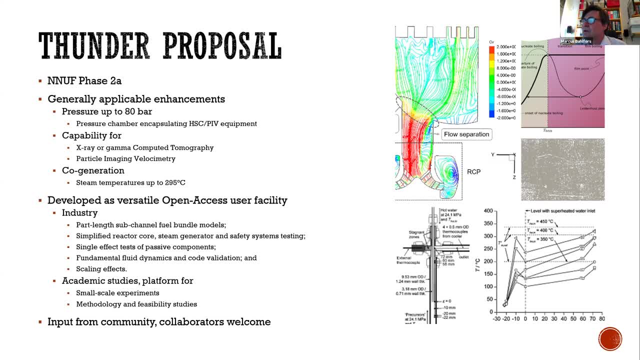 but at the same time, this would allow, as a second, Curtin, which is an interesting thing because it is not a problem. If you are trying to use a water pressure system, you can have a medium pressure system and then, at the same time, you have a lower pressure system. 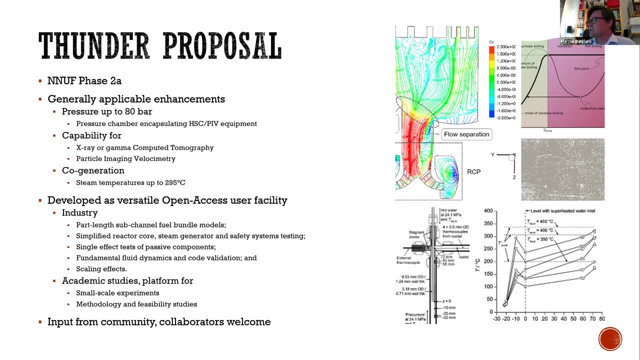 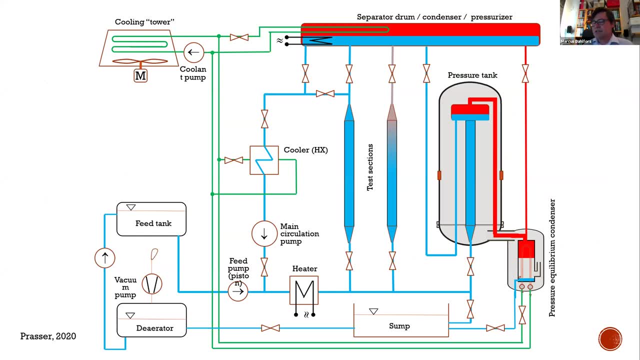 which would get the temperature to a 5 to 10 meter pressure, same as you do with a sure temperature system. That's a very good answer. This is the basic scheme of the loop that we are proposing, and especially the system here with the pressure tank and the pressure equilibrium condenser is quite bespoke to this and it requires an inert atmosphere of nitrogen to be run. 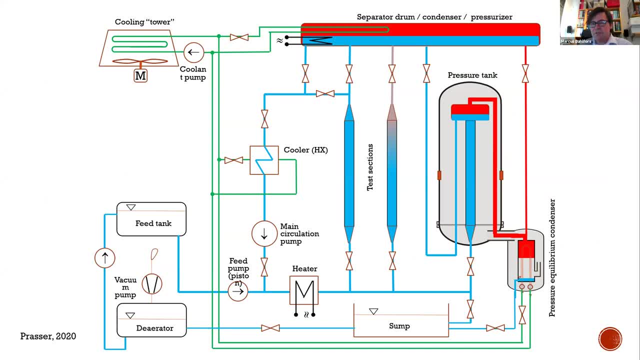 It has generated a bit of interest and actually I've spoken to some people within the UK NTH SIG network and who are also interested. There are also other complementary concepts out there for this call and many things look interesting, but this is now ours. If we are successful, we would obviously look for collaborators. 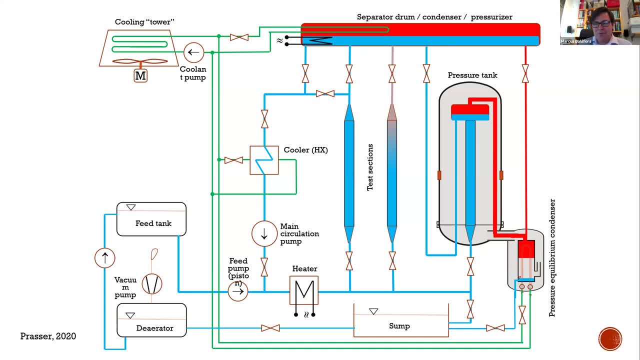 Thank you, And people with suitable problems to test in this kind of facility. How are we doing for time? Thank you, I'm happy with that, So if you have questions, don't hesitate to contact me later. Thank you. The next one is David Emerson from STFC. 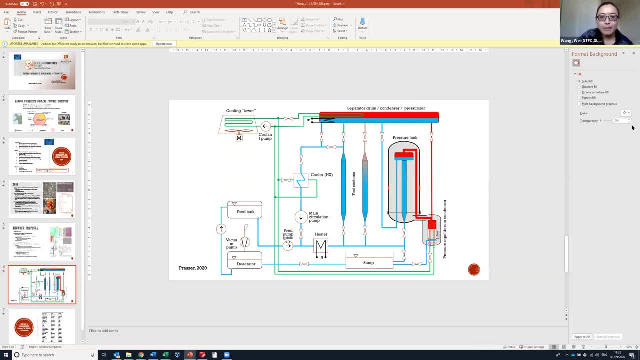 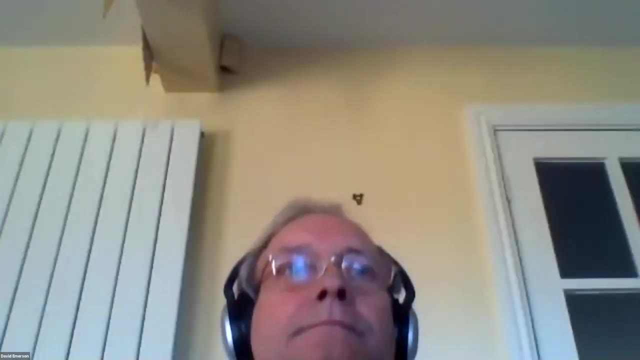 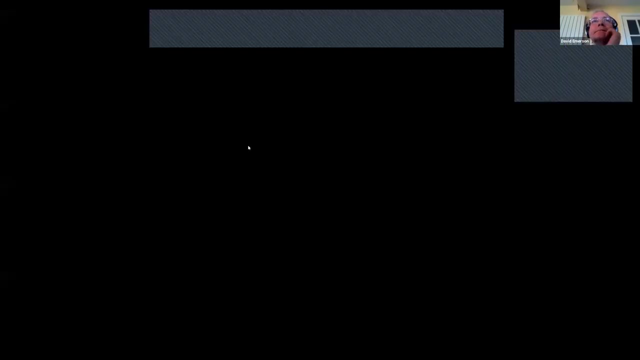 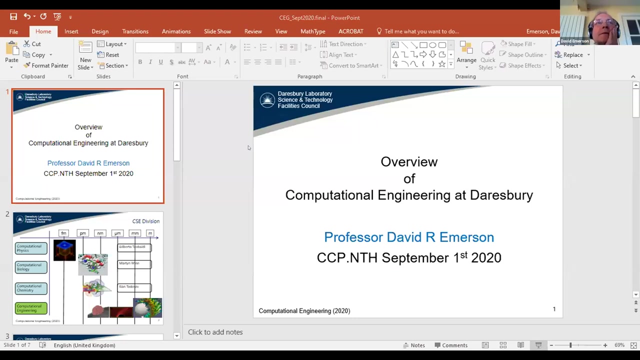 That's brilliant. We are using the product of RT. Can you stop sharing? Just on my screen it disappeared. There we go. Thank you, That's fine. Hopefully everybody can see that. Yes, Right. So I'm going to just give a brief overview of the group. I mean, you've already heard. 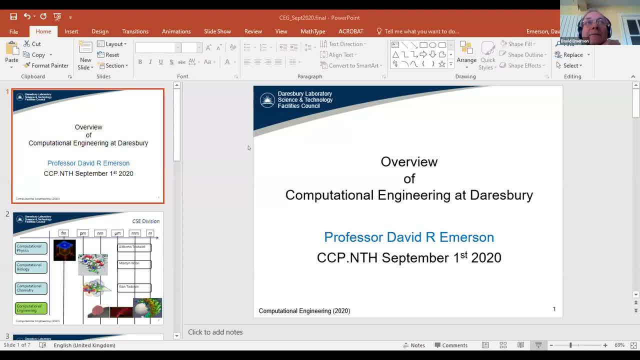 from Wei about the CCP and some of the activities we're doing there around the nuclear. So this is a little bit broader around the department and some of the other work going on. So we're part of the department and it's computational science and engineering division within the 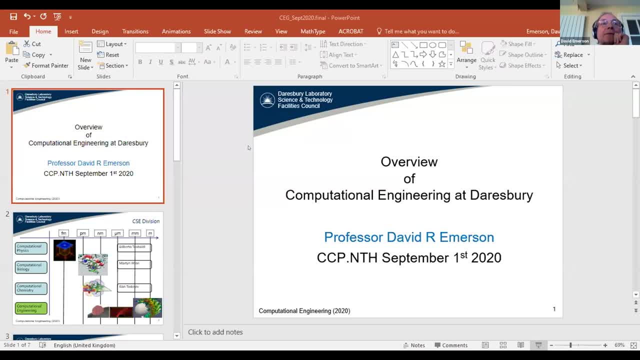 scientific computing department And within ours we have four branches. We look after the engineering, but we also have physics, biology and chemistry. All of these have a long history in CCP activity from different areas. but it gives a kind of indication of the range of 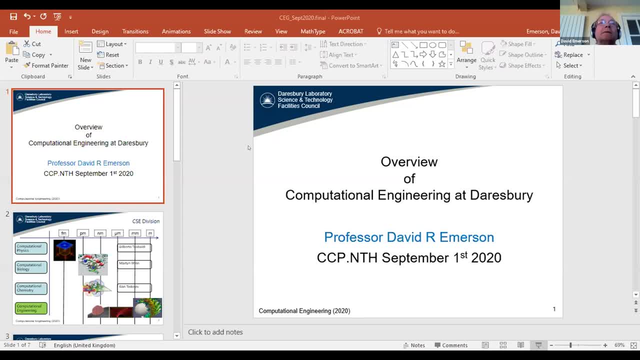 length scales that we cover from electronic structure of matter looked at in the computational physics, Lots of computational biology work that Wei has mentioned with the GBSRC and MRC and a very strong computational chemistry activity as well, which has included looking at materials for nuclear storage and looking at damage to nuclear vessels using 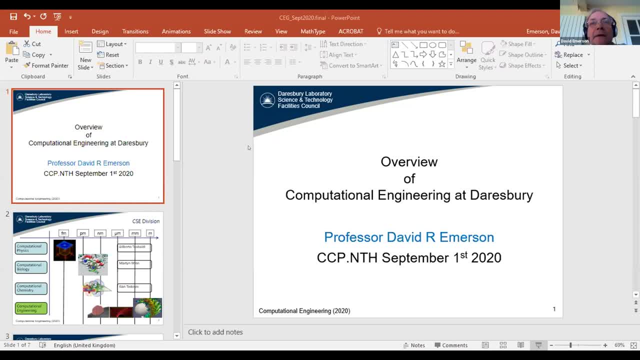 molecular dynamics. We've just started a little in-house project. It's a short project with us using molecular dynamics to investigate some of the properties of molten salt reactors, to try and understand some of the terms in there. The research topics that we cover are quite wide ranging over the years. Some of these 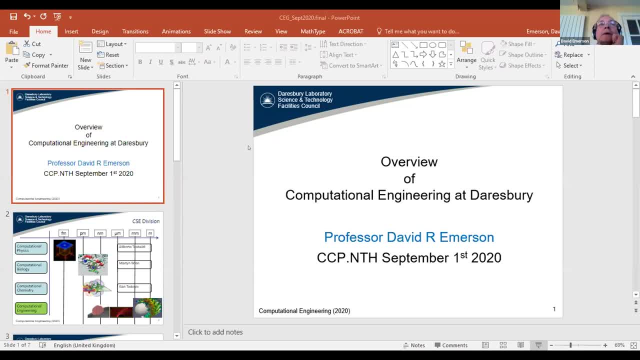 are active at the moment. Some are a bit quieter, but everything- through turbulence, combustion, free surface flows, aerodynamics, environmental flow modeling, micro- and nano-fluidics, rarified gases, energy- Of particular interest at the moment that we're looking at is the role of solar energy in the environment. We're looking at the role of solar energy in the environment and we're also looking at the role of solar energy in the environment as well as the role of solar energy in the environment, And this is, as I said, in terms of the energy generation. 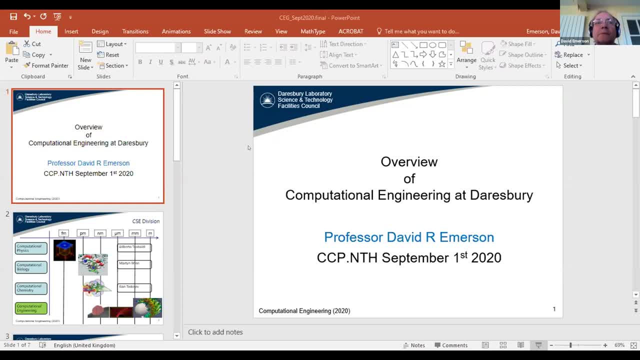 at is the Petra and Exacell software development. We have a number of projects around that and in multi-physics and multi-scale simulation, which includes quite a bit on coupling, which is one of the big challenges. So this is just one example of some of the activities going on. 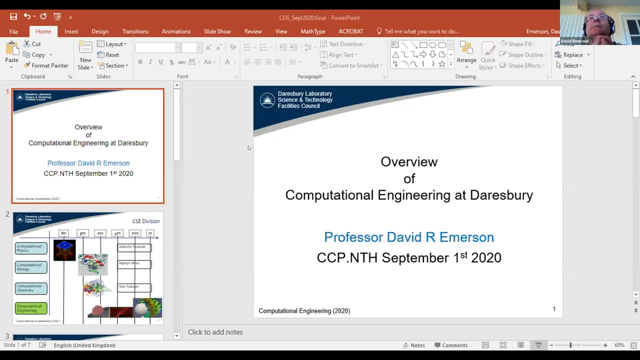 So the blood pump that you can see was an FDA challenge looking at how they could look at the hemocrit in the blood as the blood leaves the pump. I think your presentation is. you can just full screen your presentation. It's on full screen with mine. 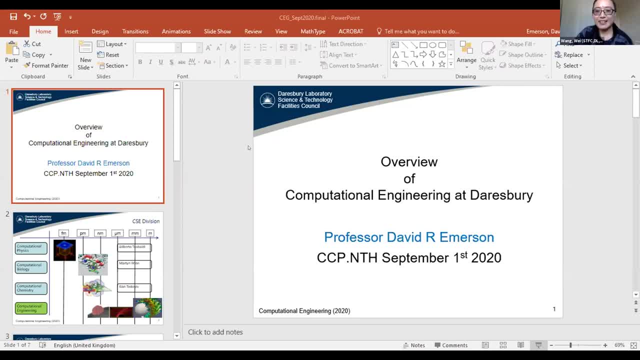 Now it only shows the first page. Oh, Okay, I have no idea why that is. It's showing as full screen on mine. Okay, Maybe you have dual monitor. Yeah, I can unplug the other monitor to see if that causes an issue. 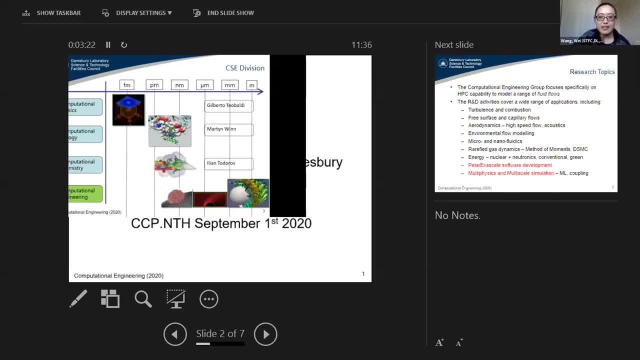 Can you see the second one? Yeah, Okay, That's never happened before. Okay, Well, okay, Just very quickly. that's just showing the various different activities. It's actually not showing very well on my screen now, which is interesting. I can only see a bit of my slide, but you can see all of it. 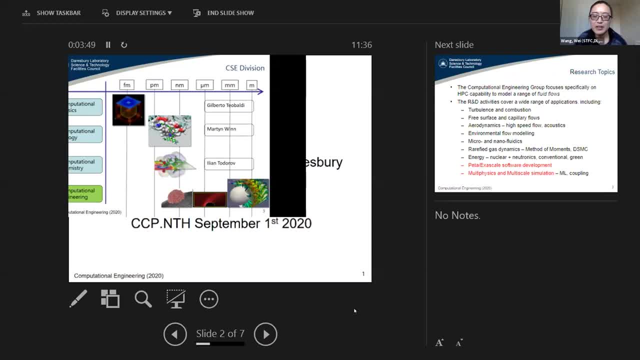 Yeah, we can show your current slide and your next one, Okay, Okay, Let me. what I'm going to do is just end it and start again, because I think it's got screwed up in a classic windows way, Okay, So. 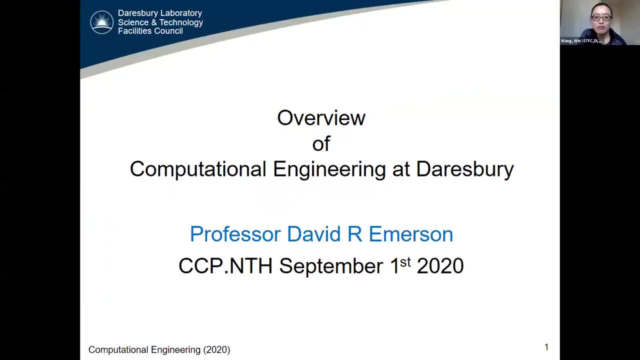 can you see? can you see it now? Yeah, that's the first page. Yeah, Yeah, Great. I don't know what happened there. He's never done that before in all the times I've used it, So anyway, so 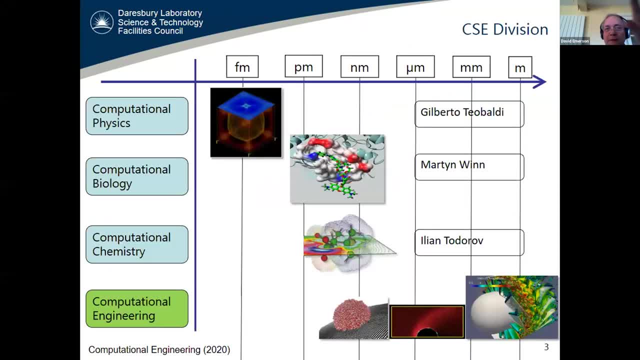 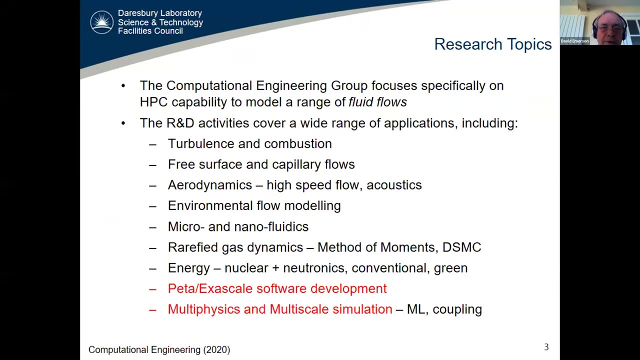 Great, Thank you, Thank you, So okay. so this is briefly going over again, just showing the length and time scales that we're operating over from lettering structure, Various sections. These are the research topics that we're looking at, But the main thing to focus on it, the ones in red, which are the areas that we're working on. 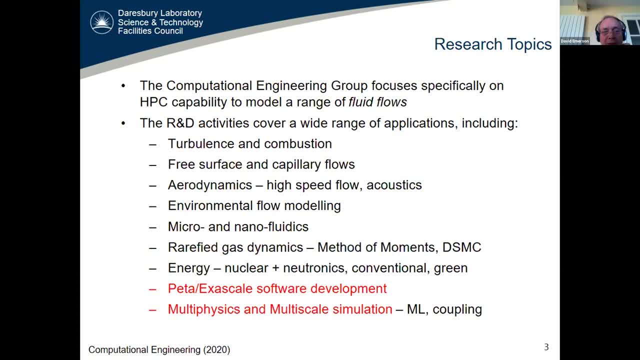 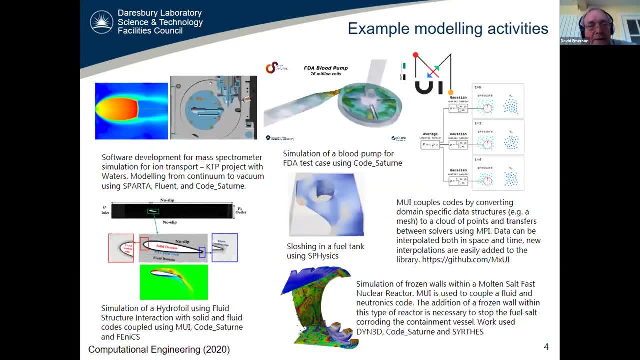 Quite extensively at the moment, which is on the Petron X scale in the multi physics and multi scale, And and this is just some of the examples of what we're doing, of projects. So at the bottom right is Project that we had looking at: salt fast reactor. 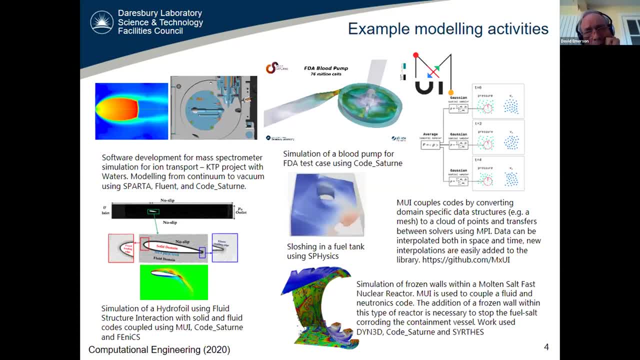 The top right is looking at coupling and in the coupling we've been developing the milk scale user interface, which is a collaboration with Brown University in the US, and This is an open source package for coupling Which is based around the MPI directive, So it's very portable and easy to add to codes. 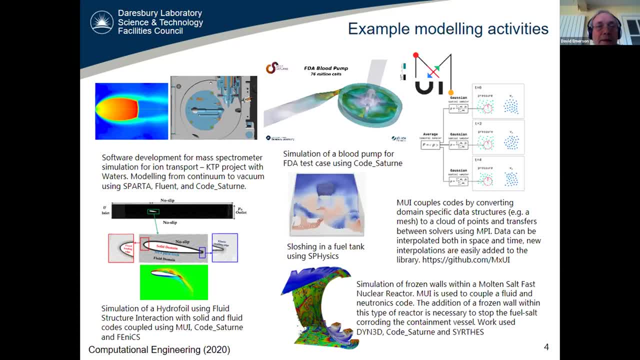 There's still a lot of work to do on developing That coupling, but our intention is to use this coupling so we can use The best code that we want for doing a particular application and then target that and couple them together. Given time is now a bit tight, I'll move on. the top left one is a mass spectrometer that we were working with. 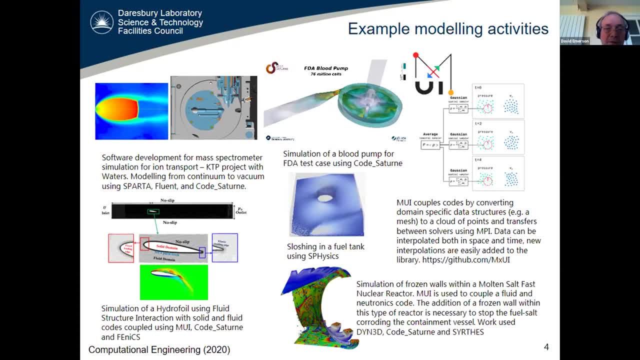 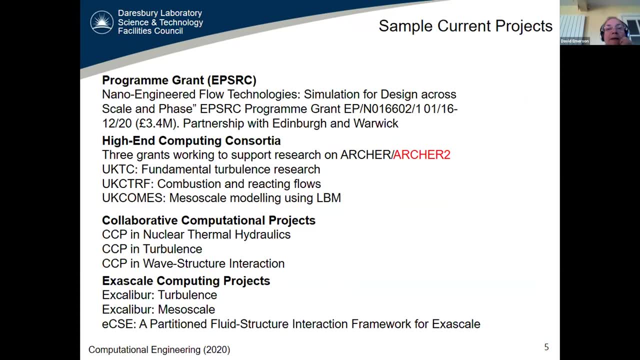 Which is a form of project that way worked on and So we need some talk about sort of fluid structure interaction, which is a project Just happened. So sample projects: We have a program grant is currently running looking. This is looking at Nanoscale and micro scale activities with 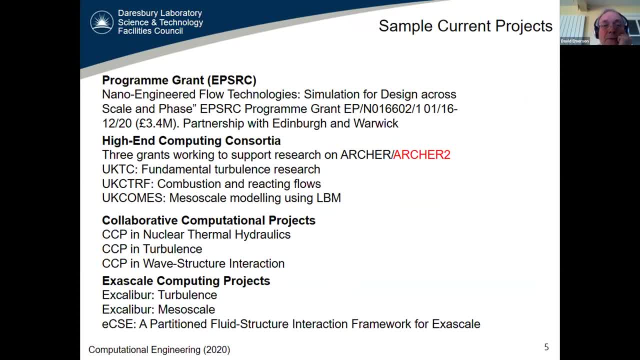 Warwick. There are three high-end computing consortia Which are quite relevant to what We're doing here. There's the UK turbulence consortium- We get a lot of our compute time within the consortium from UK TC. there's another one on turbulent reacting flows and there's no one looking at Lisa scale modeling and 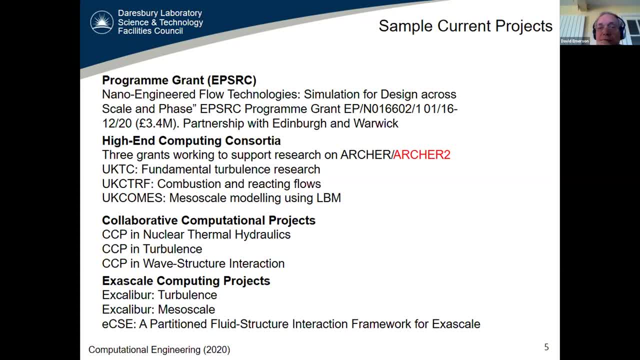 highlighted in red is the Next machine, which is not you too, And I'll just briefly touch on that in the next slide. just to say what we're targeting, There are three ccps of relevance at the moment. There's the nuclear thermal hydraulics, as we're meeting today. 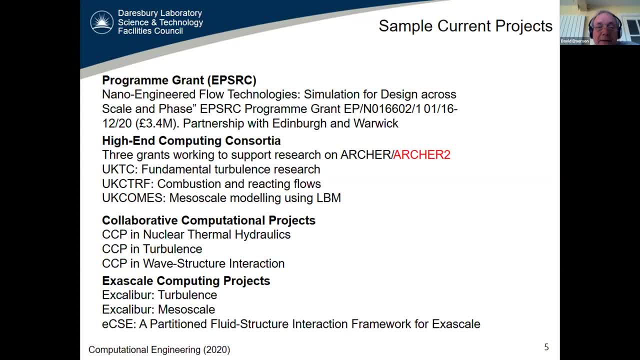 There's also a CCP in turbulence is looking at fundamental DNS, And there's a CCP in wave structure interaction and part of the target there is to look at large-scale FSI type of projects. in terms of exascale, We are nowhere near as active in the UK as they are in the US. 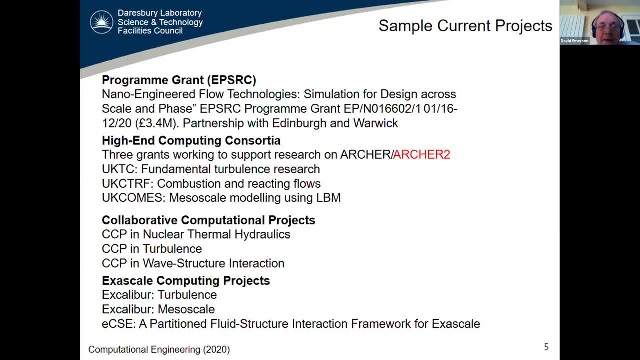 So we do have one called Excalibur, which is looking at trying to Coordinate the activities, and there's a couple that are currently running which is looking at turbulence, and one looking at Mesa scale modeling, and one of our team, Alex Cullen and Charles Moulinac, have just had a project funded. now on 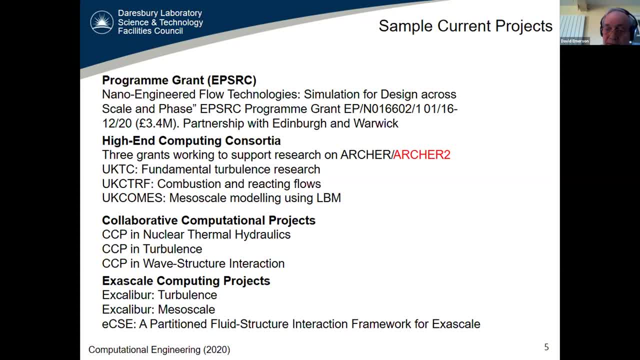 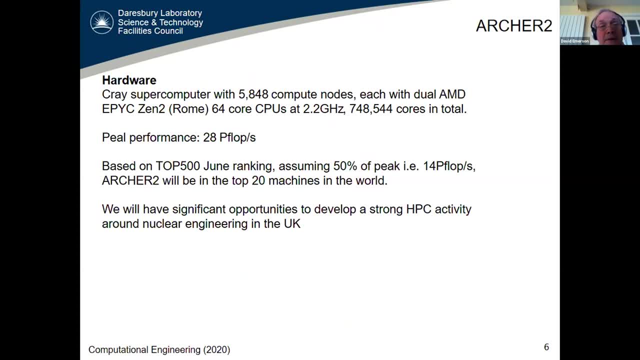 Looking at fluid structure interaction framework for exascale. so the machine that we've just had installed, although there's only Four cabinets at the moment, The rest is So on its way- It's a crazy supercomputer with five thousand eight hundred compute nodes. Each of these have the AMD epic Rome. 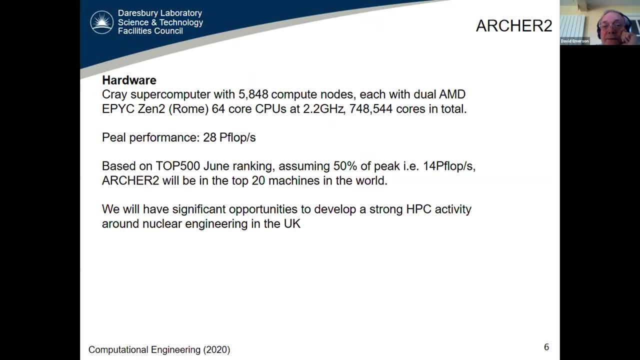 but you So 700, just under seven and fifty thousand cores in total. the peak but the peak performance is 28 petaflops and based on the June ranking from 25 vendored. and so over the next year we will continue to have a number of four cabinets with a number of five thousand compute nodes, and here this is actually four cabinets at the moment. the rest is sort of a way it's a crazy super computer with 5800 compute nodes. each of these have the AMD epic Rome CPU, so just under 750,000 cores in total. the peak but peak performance is 28 petaflops and based on the June ranking from 2500, and based on the June ranking from 2500ʹ. 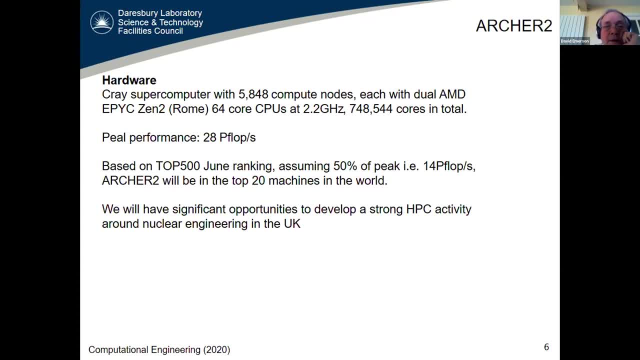 top 500 D, Assuming we've got 50% of the peak, we'd be around about 14 petaflops, which would put Archer 2 in the top 20 of the machines, somewhere around about number 15 or 16,. I 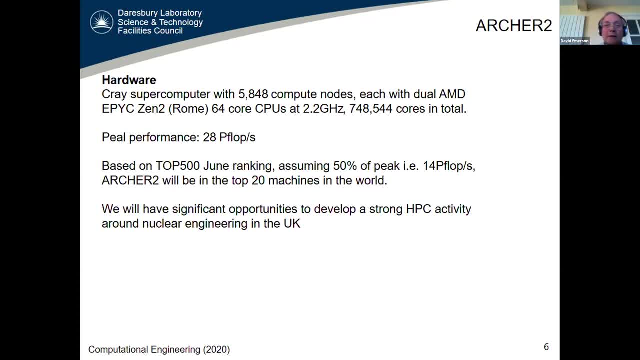 anticipate, And we're already planning to have a substantial activity on Archer 2.. So that's it. Sorry for overrunning slightly with the mess up on the screen. Yeah, Thank you, Dave. Can we just stop sharing? The next one is Shui-Sheng from University of Sheffield. 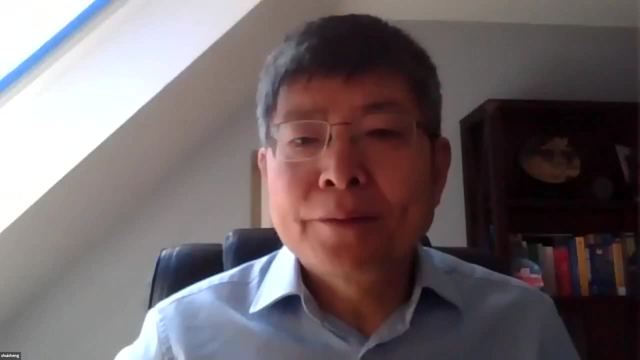 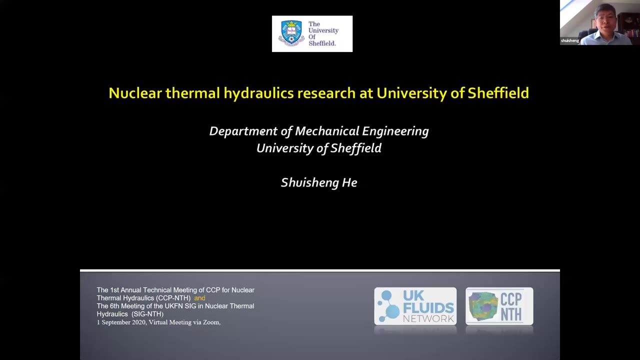 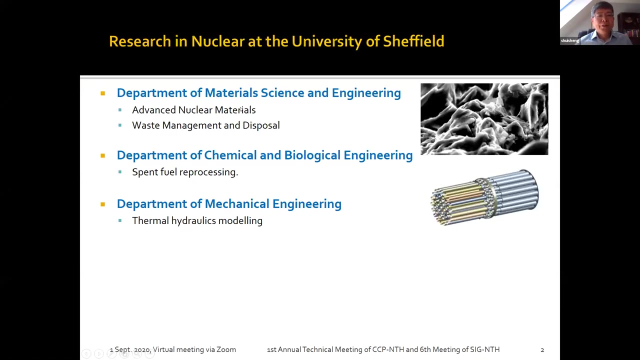 Okay, All right, Let me find the right screen to share, Is it? Yeah, Okay, Excellent, All right, Okay. So at University of Sheffield, nuclear research mostly includes research on advanced nuclear materials and waste management, And this is largely within the Department of Materials Science and Engineering. 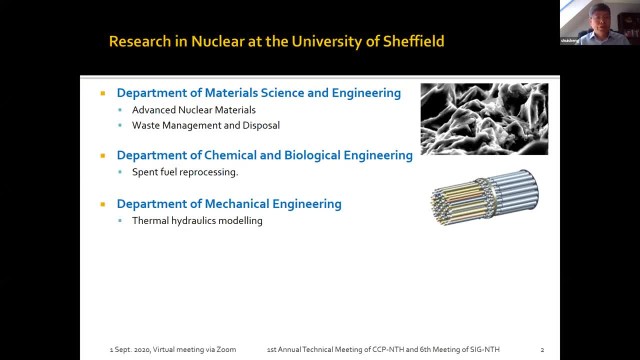 And then in the Department of Chemical and Biological Engineering, they are working on spent fuel reprocessing, And here in the Department of Mechanical Engineering we focus on thermohydraulics, which is something I'm going to talk about, But before that, obviously, 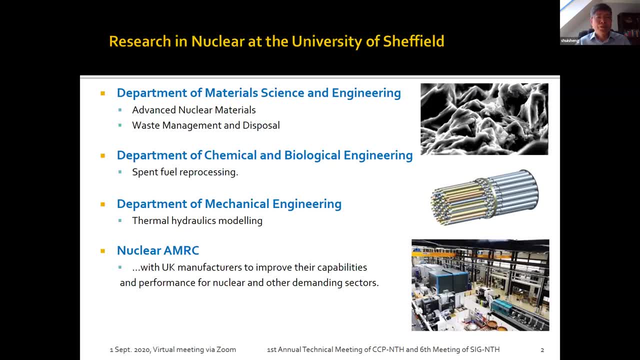 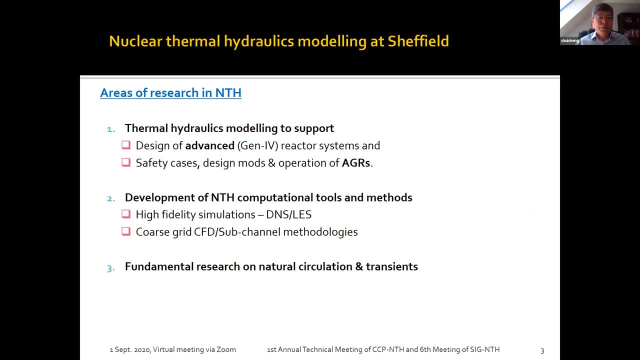 I need to mention nuclear AMRC, which is focusing on manufacturing. And now, in terms of nuclear thermohydraulics, we focus on three things, And the first one is very much like a general modeling to support the design of advanced at generation four reactor. 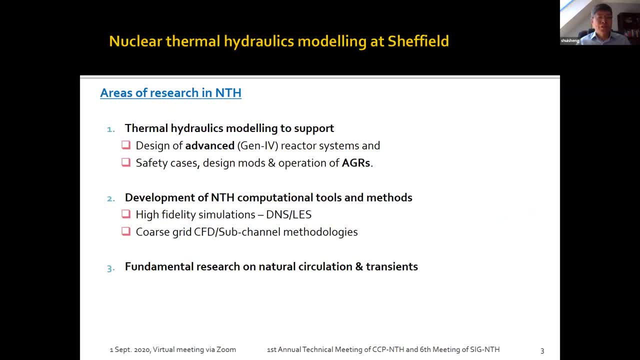 systems And also to support the safety case design, modifications and operation of AGRs. And following that, we also work on the general computational tools and methodology development, including both high fidelity simulations and cross-grid CFD. And finally, number three, 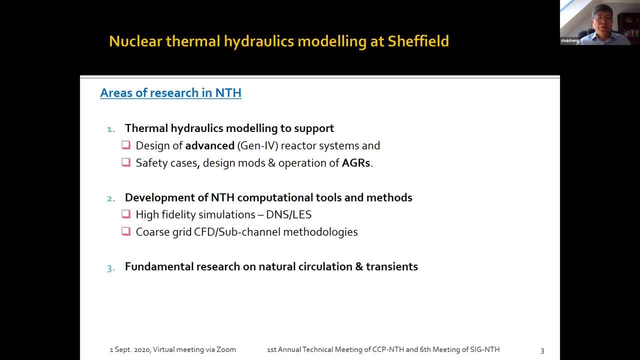 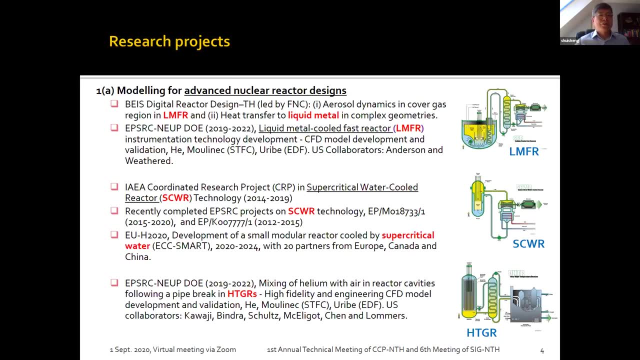 we're working on some fundamental research on natural circulation and transits process project. So next, I just gave you just some examples of research projects currently happening within the research group in the department. Now, the first one is on the modeling of advanced nuclear reactor designs, who are involved in three types of reactors. that's liquid metal. 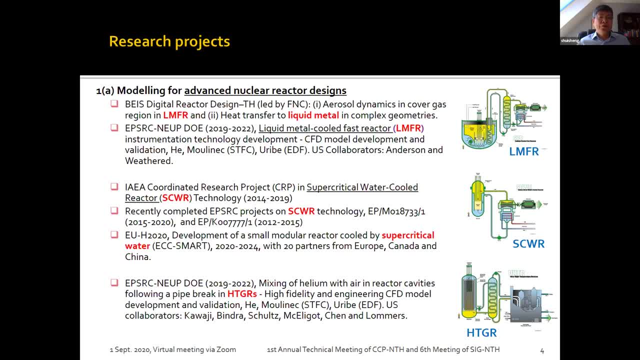 fast reactors and ICWR, super critical water-cooled reactors and more recently on high temperature gas-cooled reactor, And within the first group, were involved in the base digital reactor design, some analytics led by Fraser Natch consultant, And here we worked, been working on aerosol dynamics. 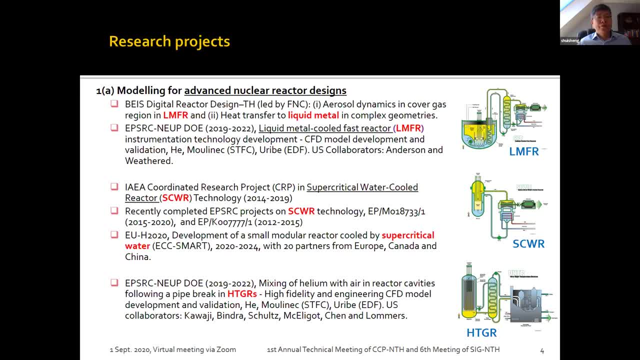 in the carbon gas region In liquid metal fast reactor And more recently we focused on heat transfer to liquid metal in complex geometries And that will be discussed later on by Xiaoxue Huang. And in the framework of EPSRC and DOE project. we are working together with SDFC and EDF energy on the 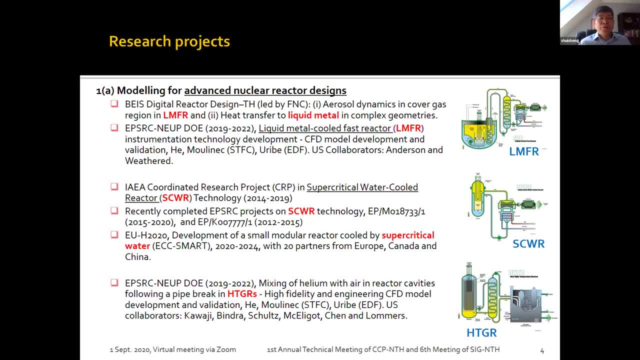 safety model development and validation in the area of liquid metal fast reactor to support the activities in instrumentation technology development in the US. And in terms of the second topic, ICWR, we've been working on this for quite a while now, over 10 years. Those were supported by 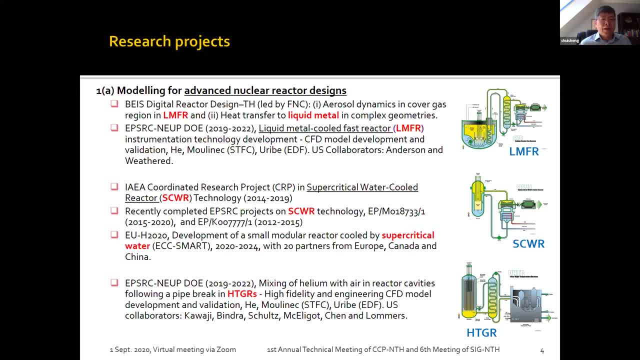 mostly EPSRC project, but also IAEA, CRPs. Now, more recently, we are involved in EU project. So in all those projects we look at the physics and modeling and this is also some of the the basis which leads to the development of numerical methods, which I'll talk on the next slide. And the last one is: 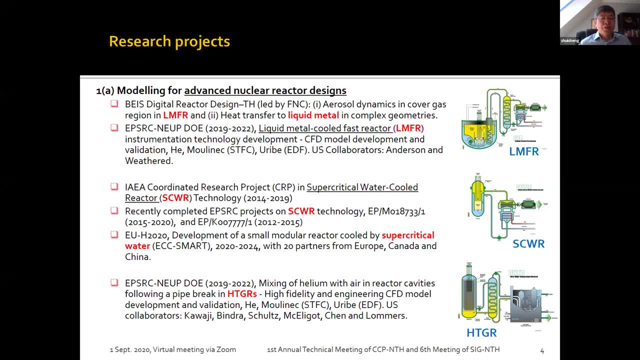 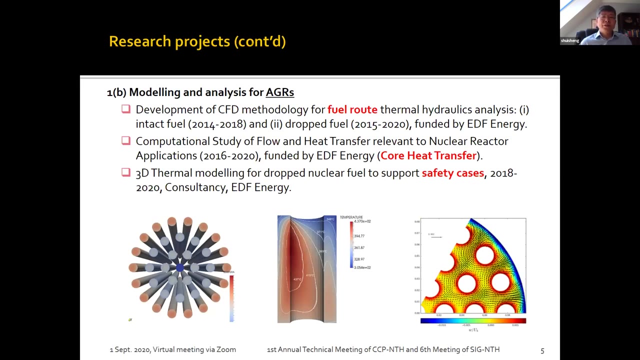 PSTGR. Again, this is part of the EPSRC, DOE, collaborating with a different group of US colleagues, And again on the UK side it's from SDFC and EDF Now in the AGRs. so we've been working in like few route modeling. There are a couple of PSTGRs. 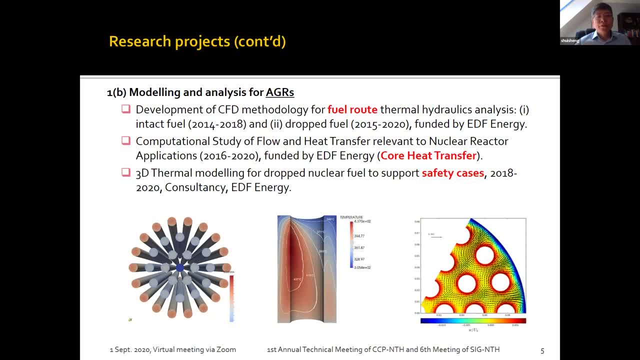 scholarships, which enable us to develop something quite interesting. And then, in terms of the core reactor, core heat transfer is something I start with, So we've been probably working with that group for over 10 years. And then, and the last one, we talk about safety case, And this particular one is a recent safety case which we have. 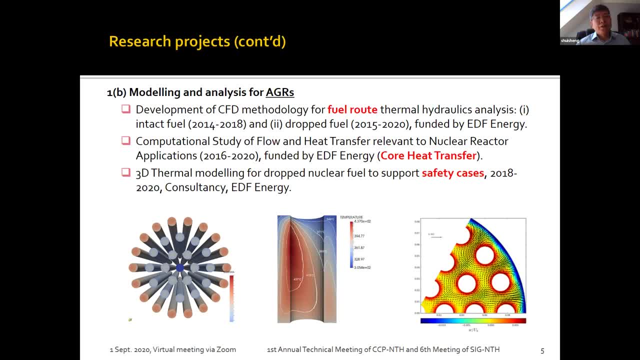 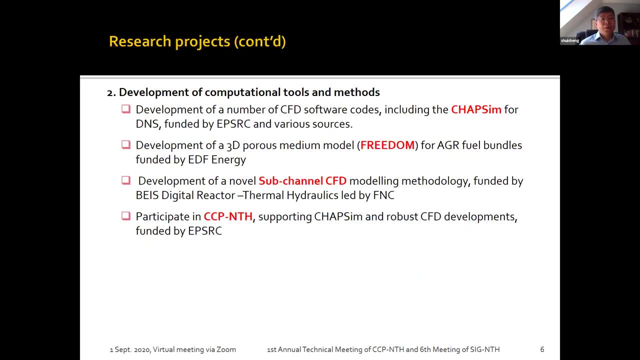 done, And we have done a bit of work to support this in an area of 3D thermal modeling, But in the past we supported various safety case development. Now, in the area of computational tools and methodology development, as a group we have developed a number of safety software codes and probably with this Let's 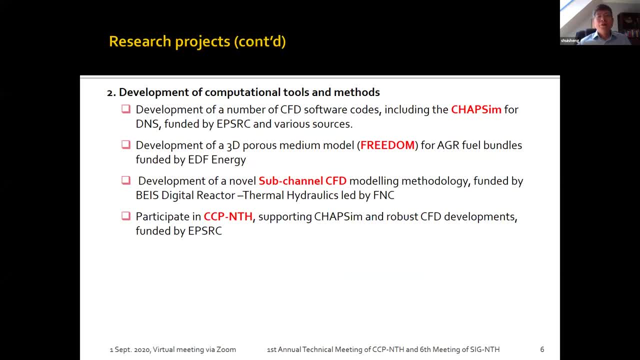 focus on that. That's what we want to do, But that also includes CHAPSIM for DNS, And obviously the main developers are Mehdi Siddiqui, who is currently at Liverpool General Motors University, And also Dr Wei Wang, currently at SDFC. And in the second item, we actually developed a 3D porous medium model. 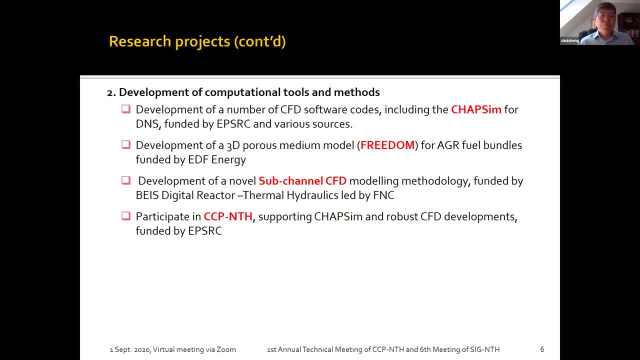 And in the second item we actually developed a 3D porous medium model. And in the second item we actually developed a 3D porous medium model called FrZen for AGR fuel bundles. called FrZen for AGR fuel bundles. This is something we hope to use to support. 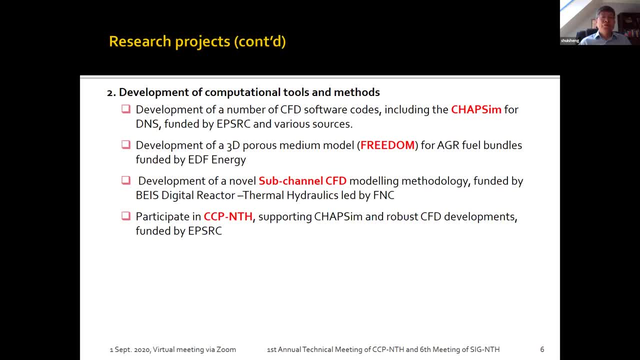 all the safety cases related to natural circulation, both in terms of intact fuel and drop fuel scenarios. And the third item on this is a development of a novel CFD modeling methodology. This is funded by Bayes Digital Reactor Thermodynamics, again led by Fraser Natch, And again this will be discussed by Dr Bo Liu in the afternoon. 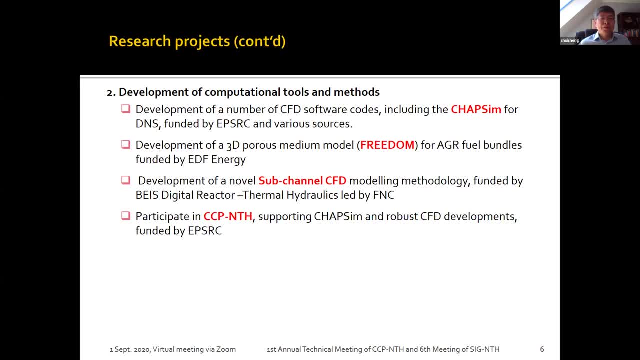 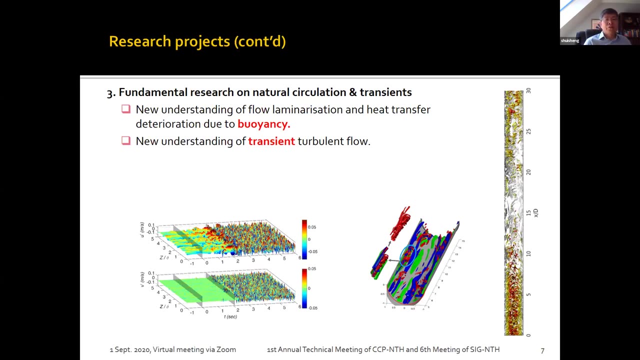 And, lastly, we participate in the CCP, hopefully to support and benefit from the development of Chapsim and robust CFD. And what is this? This is natural circulation and transient flow research, which are relevant to various kind of scenarios in nuclear sector. you know, both in terms of the 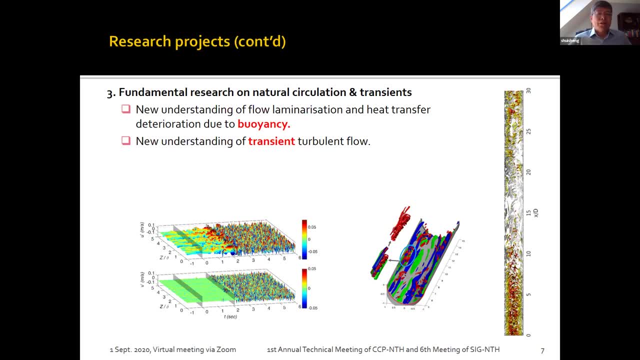 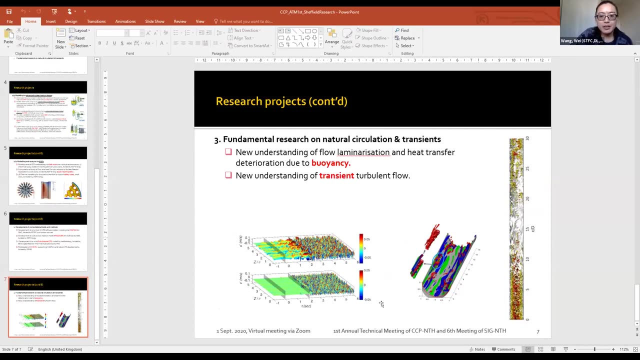 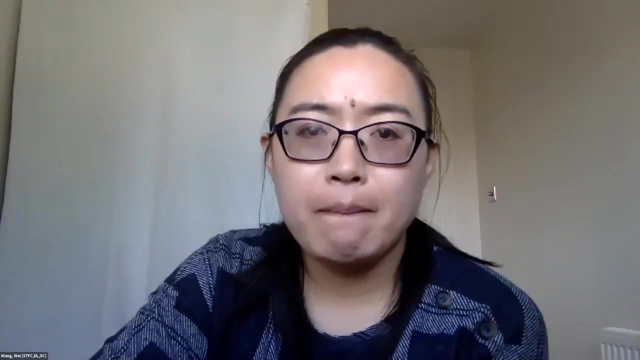 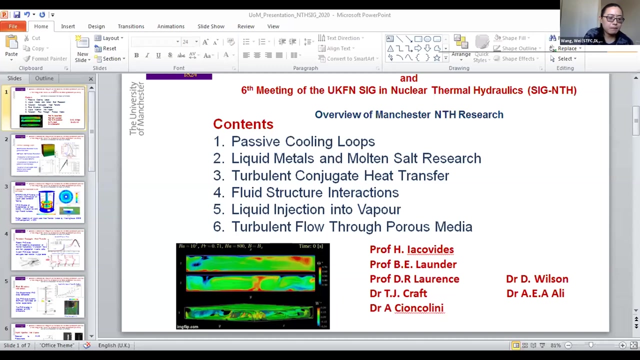 transient flow, startup or shutdown, but also in terms of passive cooling or points-driven flow. I think that's everything. Yeah, Thank you, Xuesheng. The next one is Hector from University of Manchester. Okay, Okay, Can everyone see the full screen? 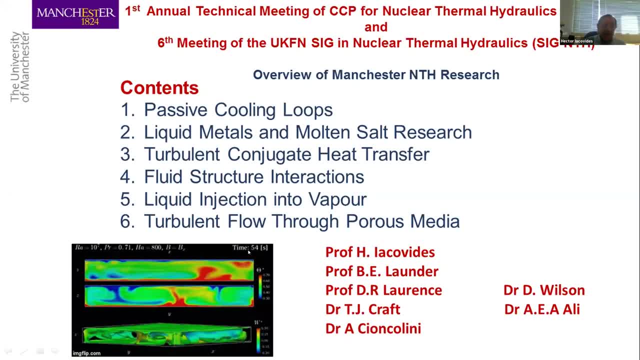 Yes, Okay, Thank, Hello again. Over the next few minutes I'll try and give an overview of some of the current and also recently completed research in the area of thermohydraulics within our group. Down here I have the names of the academics and PDS. 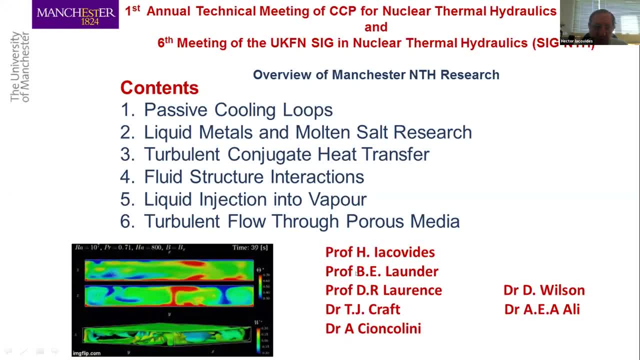 There's a very interesting group already that currently works in this area within the group. I should perhaps also add that at Manchester we also have the Modelling and Simulation Center, set up by a DEF Energy and now been joined by other external collaborators. 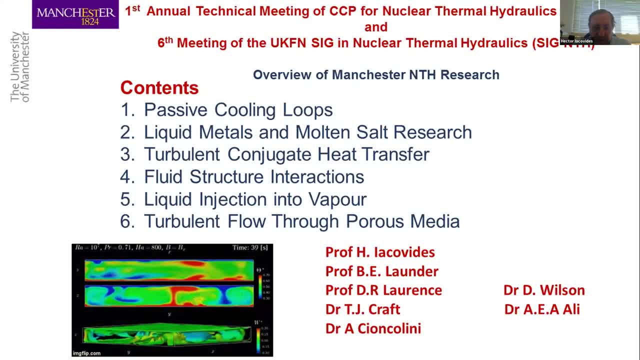 We also have the Dalton Nuclear Institute, which provides and supports nuclear research right across the different disciplines. So in common jointly with Imperial College, we are a Rolls-Royce nuclear research center Here. I'll just quickly go through some of this list of items. 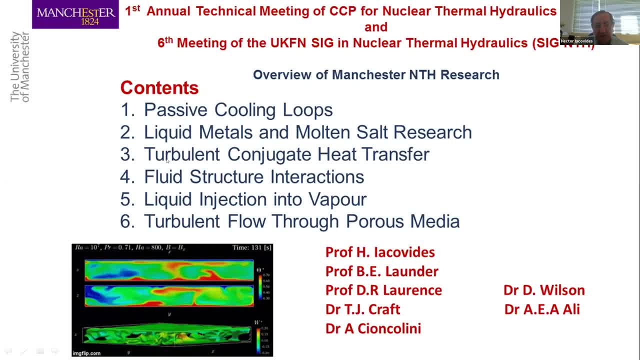 It is actually by no means exhaustive. I just realized, for example, that I left some of the experimental research that my colleague Andrea Chiocolini has underway on boiling, But it will give you a flavor of what we are up to. 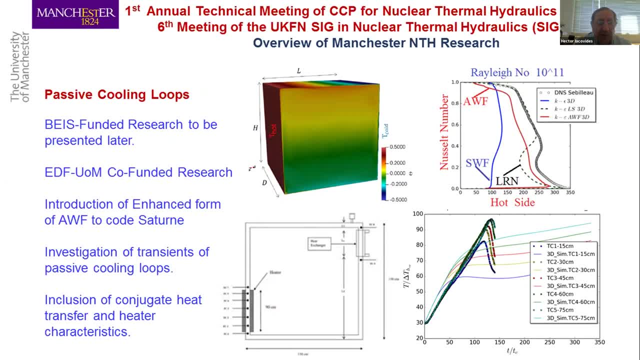 Passing cooling loops is an area we are quite active. We have funding from BASE through the BASE Friends in Asia project, which Dr Wilson will be discussing further later on. We also have another PhD studentship co-funded by EDF and the University of Manchester. 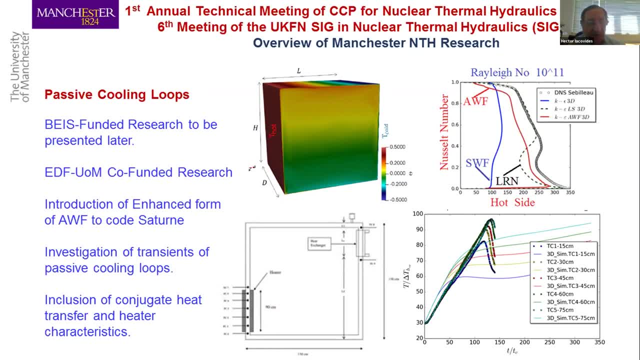 We look at more fundamental aspects, starting with more fundamental natural convection flows, where the student introduced the analytical world function into code Saturn which, as you can see here, it has quite a big impact on the accuracy, And he's also now looking at some of these natural convection. 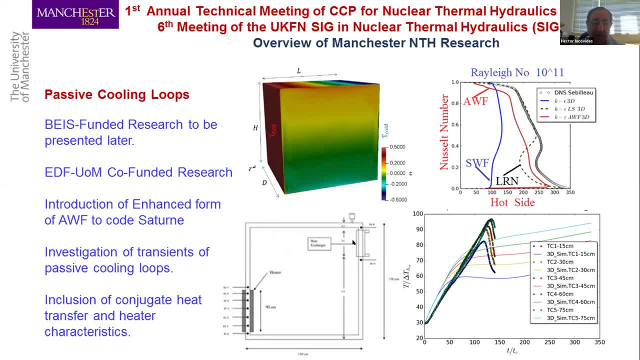 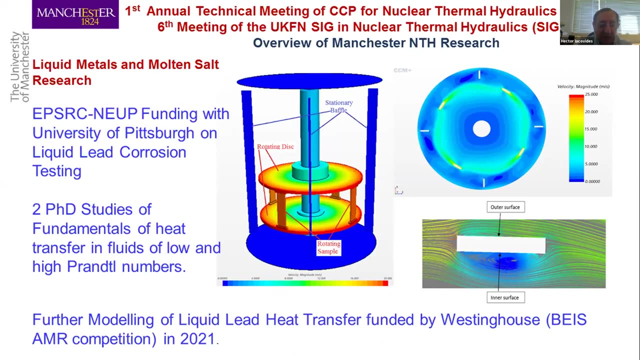 loops and, in particular, focusing on the transients and how that can be improved by including conjugate heat transfer and also the characteristics of the heater. Another area that we started working a lot recently is liquid metals and molten salt. research Funding is mainly provided by the joint EPSRC and EUP grant. 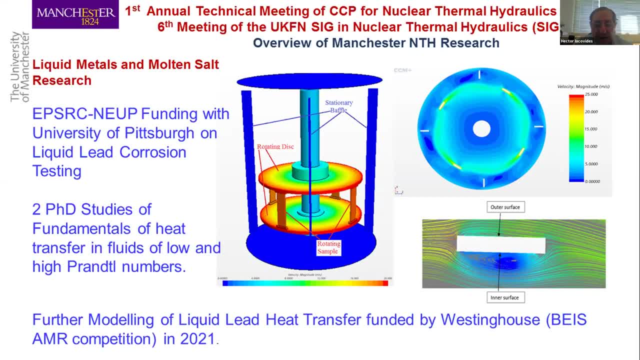 jointly with the University of Pittsburgh. Here are some examples of some of the initial work we're doing to provide some information to our Pittsburgh colleagues on how to design a molten lead corrosion experimental rig. Then we'll go on to produce some high fidelity simulations. 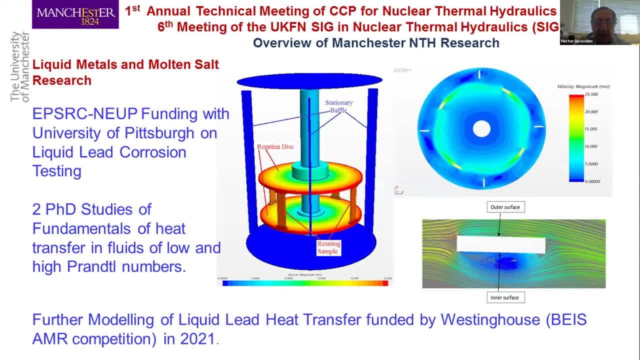 of this in order to compare with their experimental data. In parallel to that, we also have two PhD studies looking at fundamental aspects of low plant and high plant number heat transfer. And later on into 2021, we will start another project funded by Westinghouse through the base AMR competition. 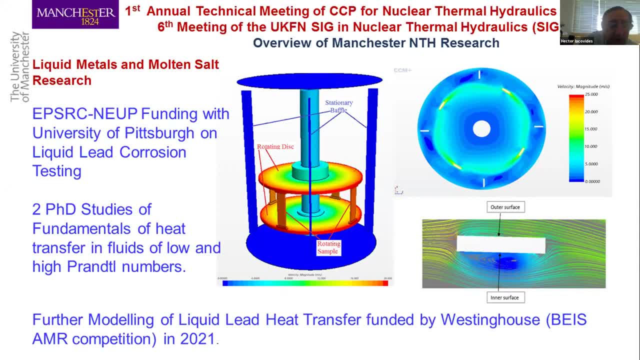 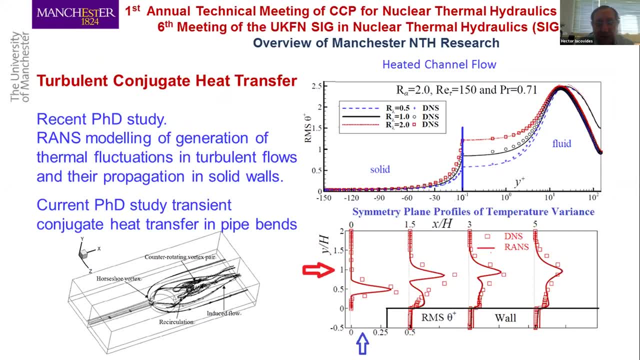 on liquid lead heat transfer as well. Another area is that of conjugate heat transfer. We recently had a PhD study completed in which we've been looking at the generation of thermal fluctuations due to turbulence within the flow and how they propagate into solid wall. 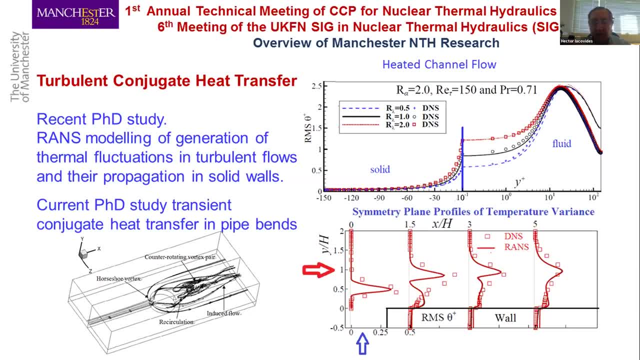 Initially looking at simple channel flows and comparing with DNS data. Having developed the model more recently, we applied that to these more complex 3D case, for which there is also DNS data, And as you can see here, it seems to be providing pretty close agreement with the DNS. 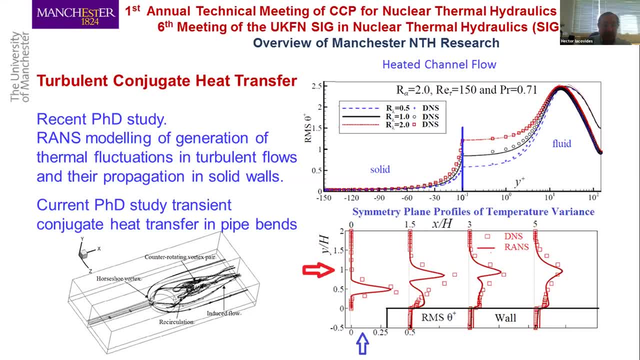 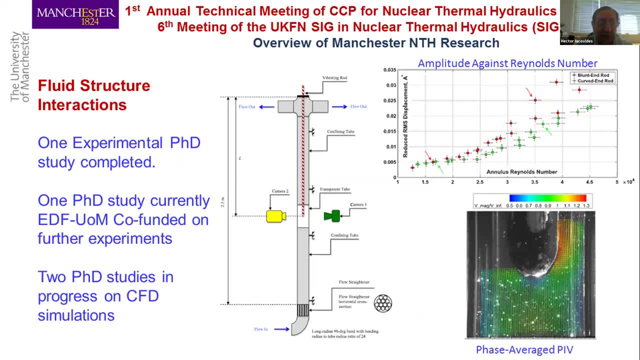 More recently, we started another PhD study looking at transient conjugate heat transfer through pipe bends. Now we are really looking at thehare Gleich закublic Ab leg ad And what we want to offer an international source study to say that aân other area is the fluid structure interactions. 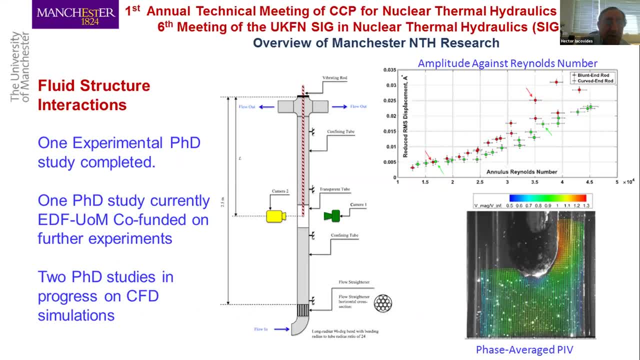 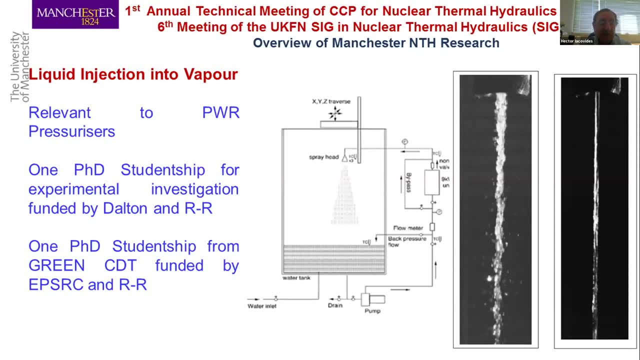 relevant to PWR fuel passages. Another area that we started recently as part of our collaboration with Rolls-Royce is liquid injection into vapor, which is relevant to the pressurizers in PWRs. We have an experimental PhD investigation and this is the leak we developed in some of the 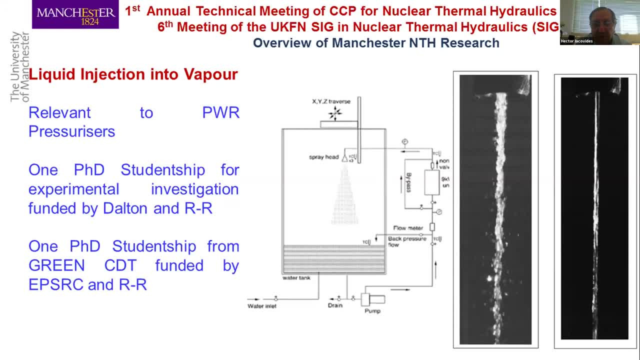 initial videos, the images that we produce for these injections. That was funded jointly by Dalton and Rolls-Royce, and we also have another PhD studentship from the GreenCDT, again co-founded by EPSRC and Rolls-Royce, looking to develop CFD models for these cases and use experiments for 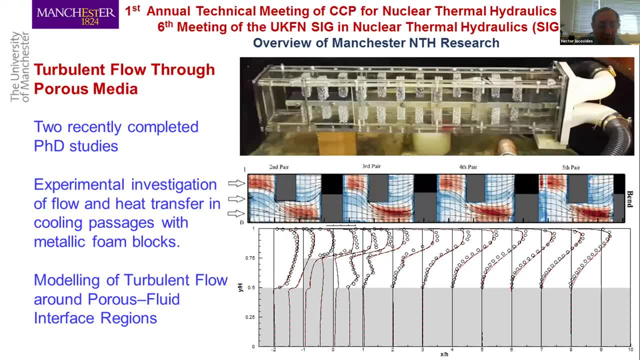 validation. I would like to thank all of you for joining us today. Thank you very much, Thank you, Thank you. Another area that we recently completed is that of turbulent flow through porous media. We had one PhD study that looked at, collected a lot of experimental data for flow and heat transfer. 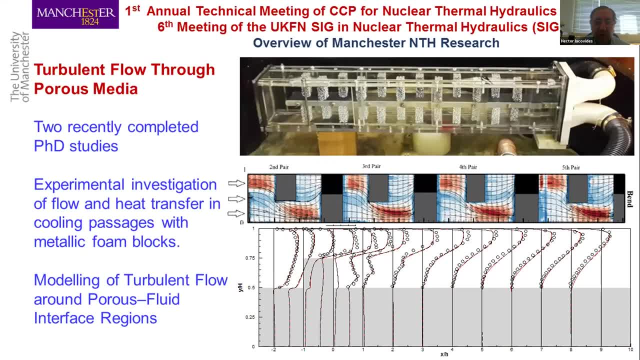 through passages which include metallic porous foams to enhance heat transfer. Here are some of the PIV data that we collected. In parallel to that we had another PhD study looking at the turbulence modeling of some of the PIV data that we collected. In parallel to that we had another 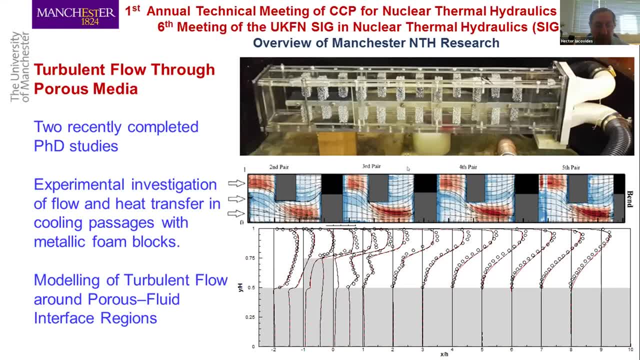 recent study looking at what are some of the interestingly interesting pieces that lead to such flows, and especially at improving and developing models that handle turbulence around the interface between the fluid and the porous regions. I suspect that's my last one, So hopefully I managed to give you a quick overview within a reasonable time. Clearly, there's a lot more to be said about those, but that's perhaps for another day. Thank you, Ericyorsun, enough time to be sad for another day. Thank you everyone. Thank you, Thank, Thank you, Thank you, And I hope that this topic lesson will take effect. correct clothing was for many of them, but we will talk about it later. 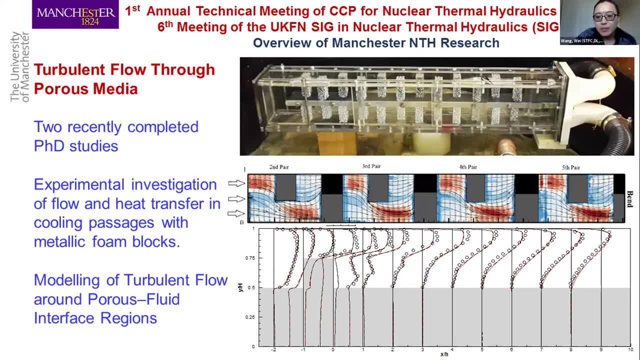 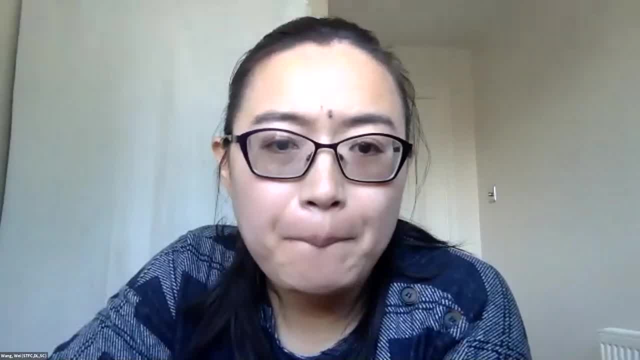 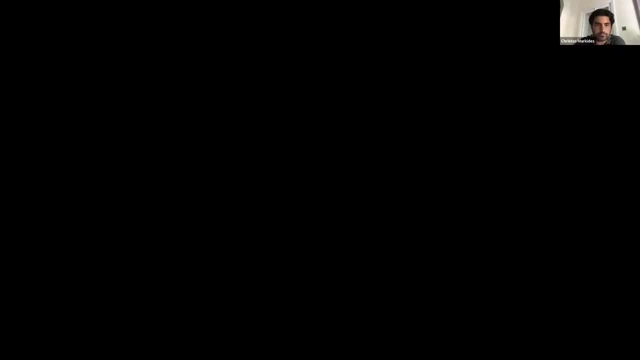 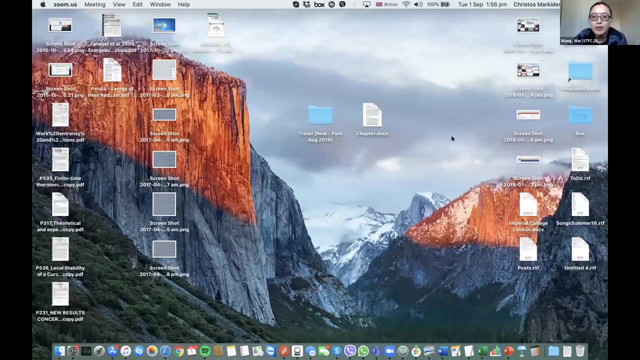 Thank you, Hector. The next one is Christos from Imperial College London. Hi, so it says I can't share the screen. Let me try again. Okay, Does that look okay now? I think you need to. yeah, Now it's okay. 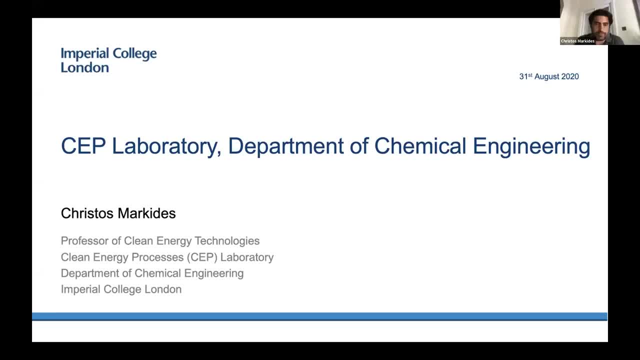 Okay, So thanks very much. I think we had a presentation which mentioned the work in the Department of Mechanical Engineering- the first one- and also some mention of other colleagues in other departments, So I'm going to focus on the Department of Chemical Engineering. There were three main academics in our department working in related areas. 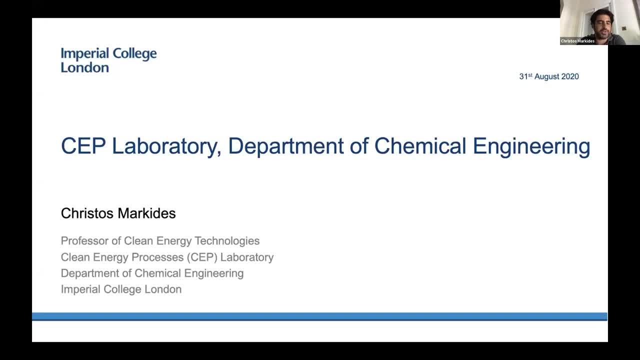 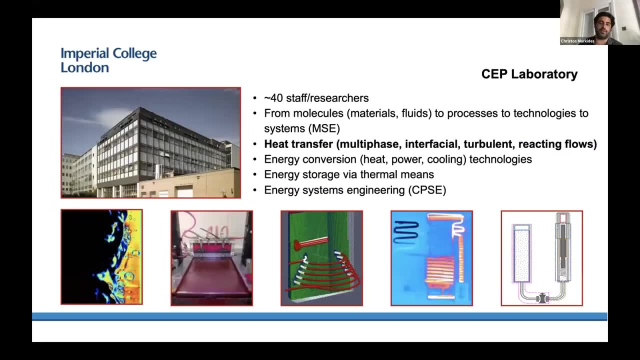 Unfortunately Geoff Hewitt passed away, so it's really down to myself and a colleague, A colleague of mine, called Marcos Milan. In our group we have- you know, this is the size of the group- and we tend to do work that goes from all the way, from sort of processes, and I mean sort of heat transfer, mass transfer processes. 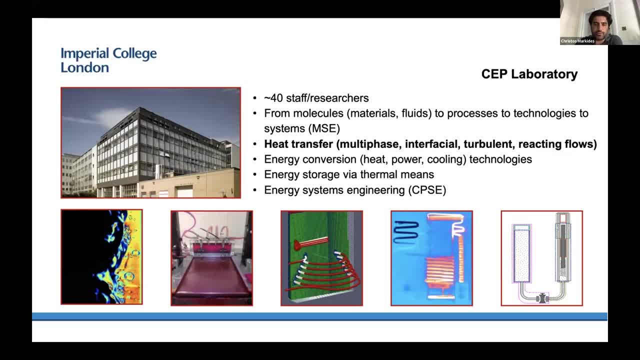 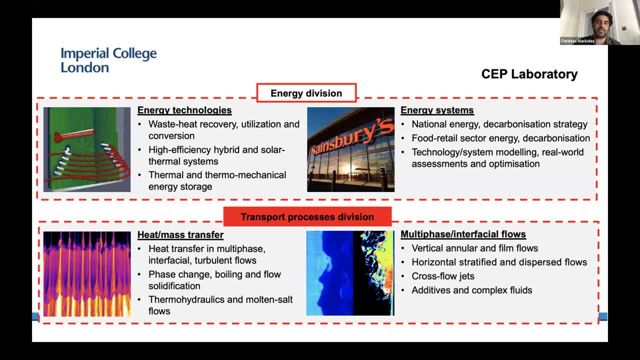 up to technology, devices and systems, And I won't really talk to you about everything, but I'm going to focus basically on the red bit for this particular presentation. Being experimentalists, I suspect that you know the most useful thing we could do for. 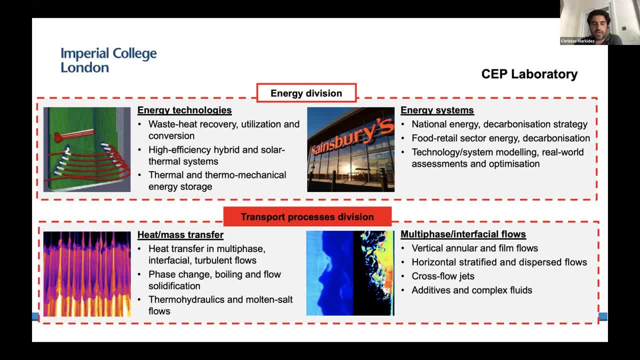 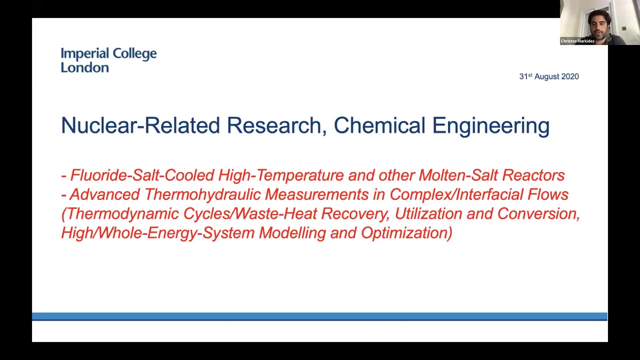 people who are on the call today is provide high quality experimental data for model development and validation. So I'm going to be focusing on the work we've done on the sort of bottom two, the bottom half of this slide. Okay, so we in our department- and I'm speaking also here on behalf of my colleague- we've done some work a few years back. 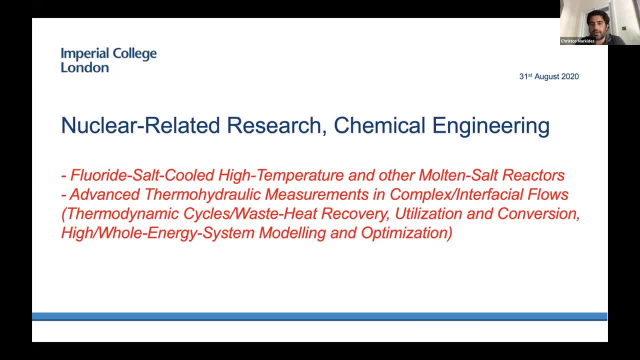 starting from fluoride salt-cooled, and also we developed an interest generally in sort of molten salts as heat transfer fluids for nuclear applications and nuclear reactors. This was an interest of Jeff Hewitt's and we had a number of a couple of PhD students. that were funded through the CNE, the Center for Nuclear Energy at Imperial College. 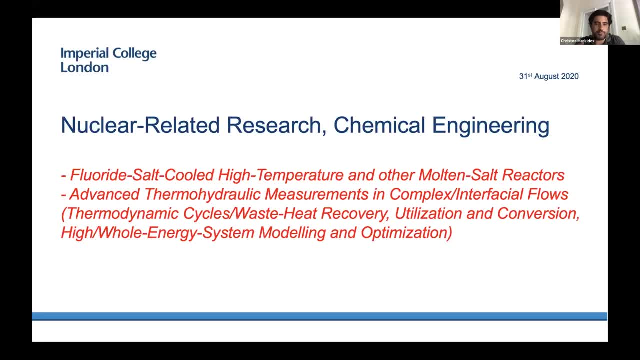 But I think, really, the core of what I'm going to speak about today is the second bullet point, although I will say a few things about the first one. I'm basically going to present to you some experimental capabilities which we're quite keen to apply to flows which will be, which are of relevance, I guess, for model development. 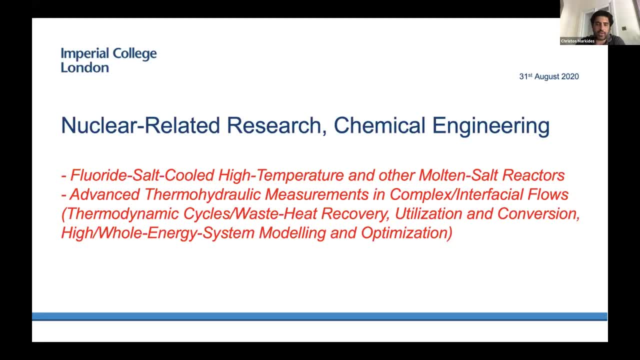 We do, then, a lot of work on, let's say, what happens to the heat-heat recovery, utilization, power cycles and sort of whole system analysis. It's out of scope of the discussion but I think it's. it's useful that the people on the call know that. you know there are some people that are sort of trying to include the role of nuclear energy in the UK in a more sort of high energy way. 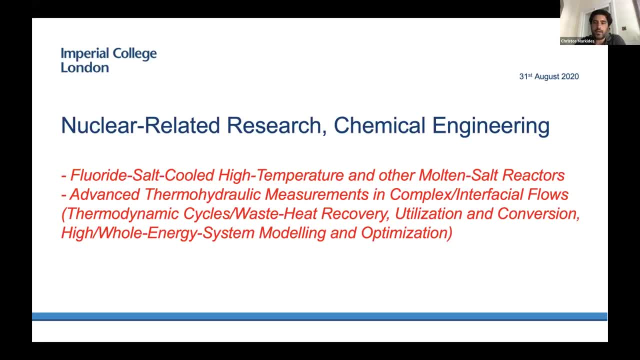 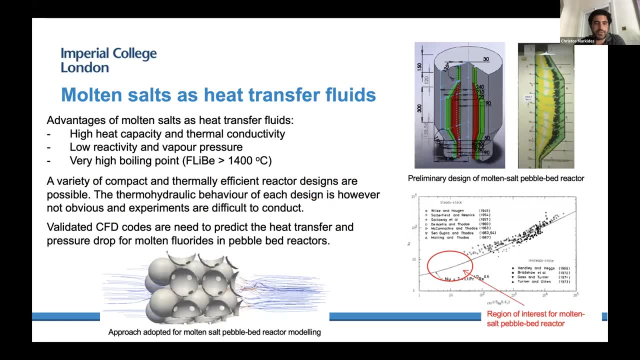 So, so, so. so system modeling sense. So I'll go quite quickly through a number of slides I mentioned. there was a. we do have an interest- that we did and we still do- in molten salts as heat transfer fluids and the design of different types of reactors. you're seeing here some work we did on pebble bed. 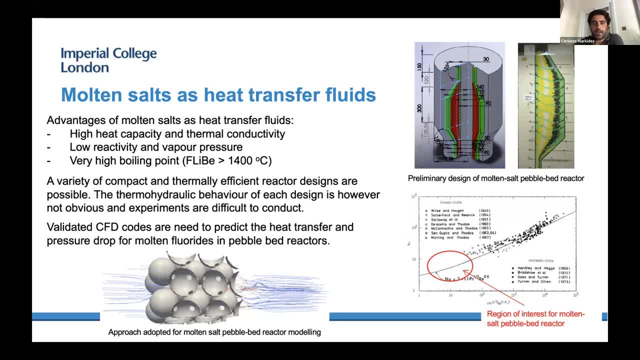 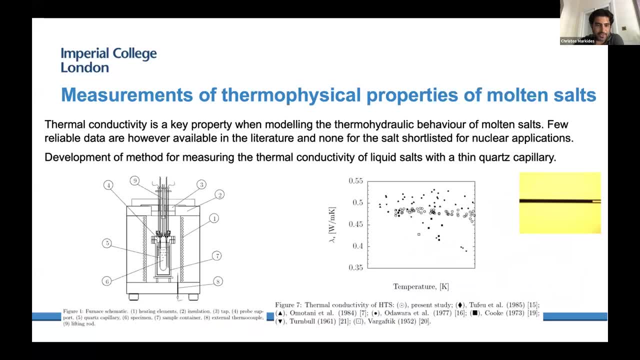 reactors with salt as a heat transfer fluid. We very quickly discovered that you know when you're doing cfd you're just entering thermal physical property values, which is a little bit of a black magic. So there was a a lot of work. a whole phd went into measuring thermal physical properties. 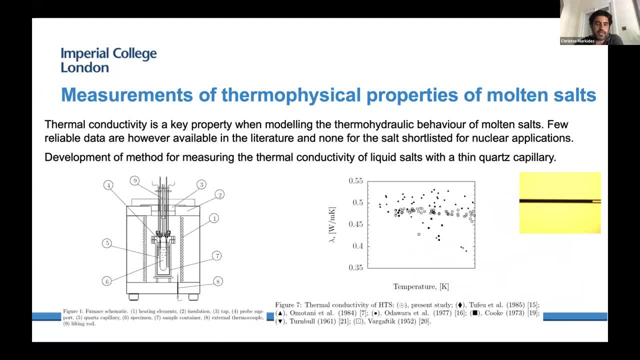 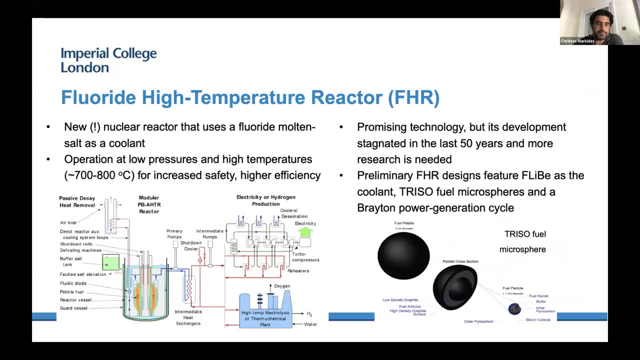 of molten salts outside of the ranges where actually data can be found in the literature. um, we then went up to the level of, you know, considering the reactor and the power cycle and and the whole plant, so trying to optimize the plant. there's an interest there and 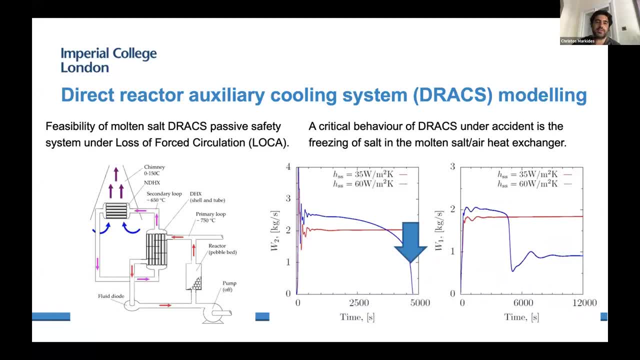 trying to answer those questions to you know, doing a burning DeadMyPan was important. I'm to design a drag system which is basically a passive cooling system for these types of and other types of reactors, and we found some interesting results. this is published. published data on um, how, in some cases, you can have freezing of the salts in these types of heat exchanges, which 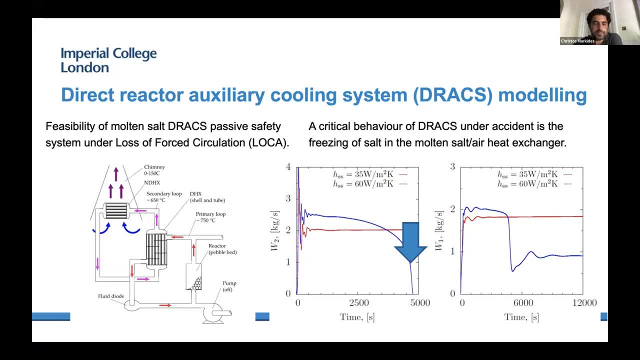 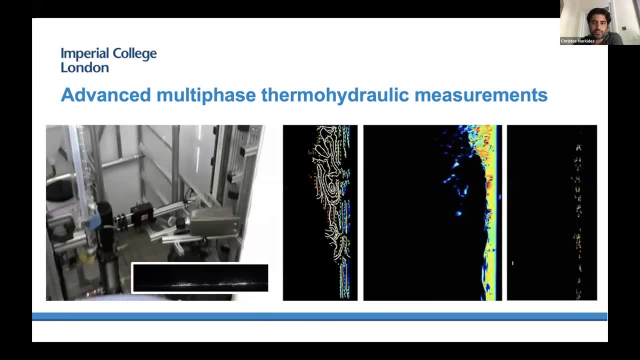 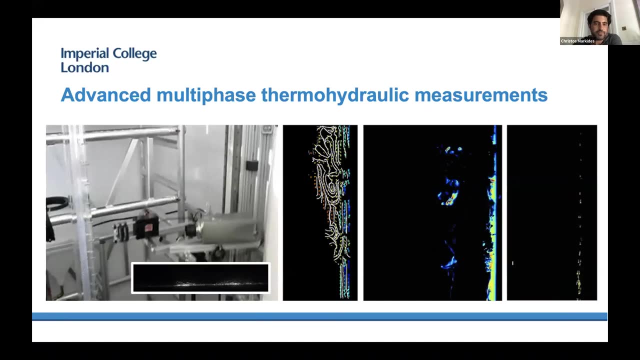 is basically a very bad news if you're trying to design something which is passively safe. okay, so let's go into the the sort of the main thrust, i guess, which would be of interest to the people here. um, in my group we specialize a lot on um, interfacial flows, two-phase flows, typically. 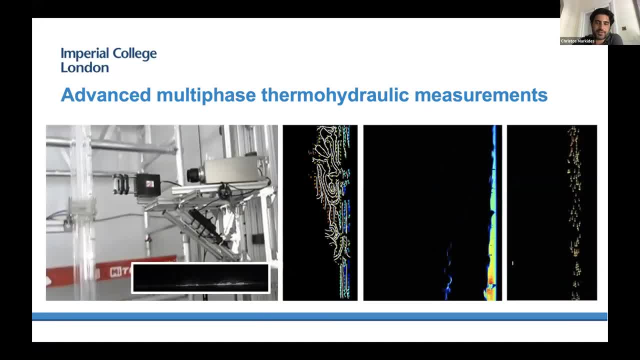 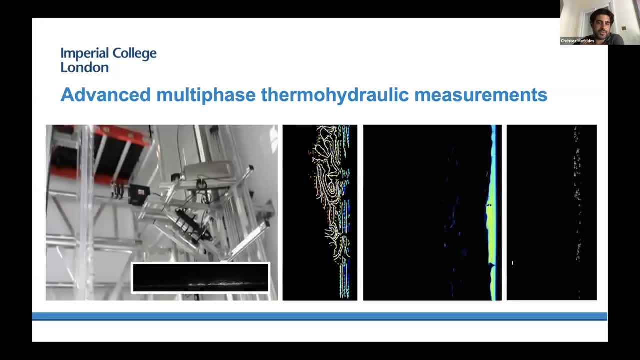 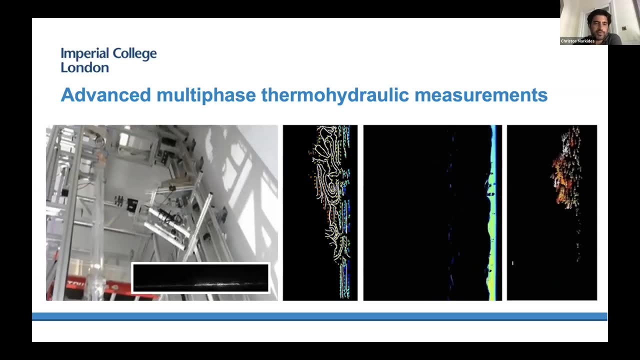 gas, liquid or liquid liquid, where there's a, you know where the two liquid phases are immiscible. also solid liquid, solid gas. most of the things i'll show are liquid gas, but there are other types of flows and we do a very wide range of measurements here. you can see um moving frame. 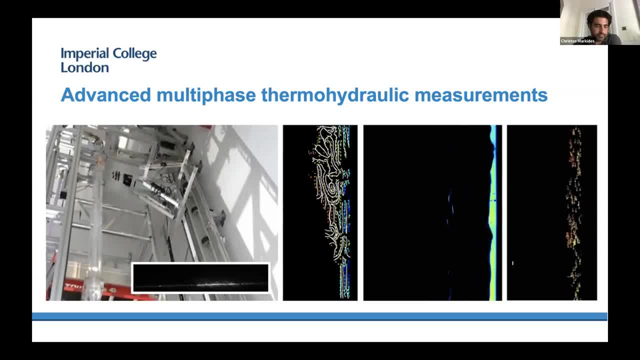 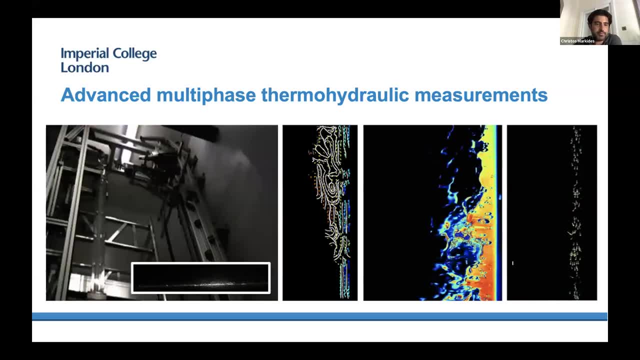 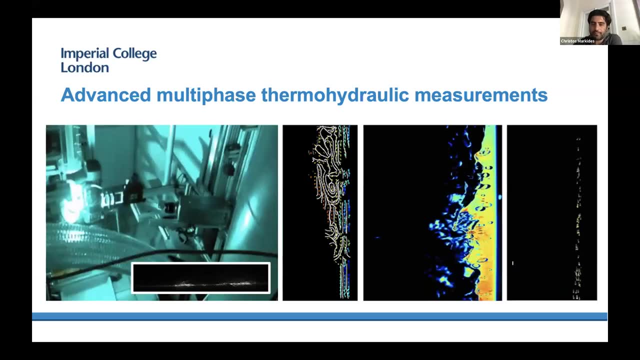 of reference measurements. on the left hand side we're in very relatively well for a lab scale, large-scale sort of experimental facilities. so we're talking about up to 40, 50 millimeters and seven to eight meter length. so i mean um, not not small scale, not bench scale, um, and the idea. 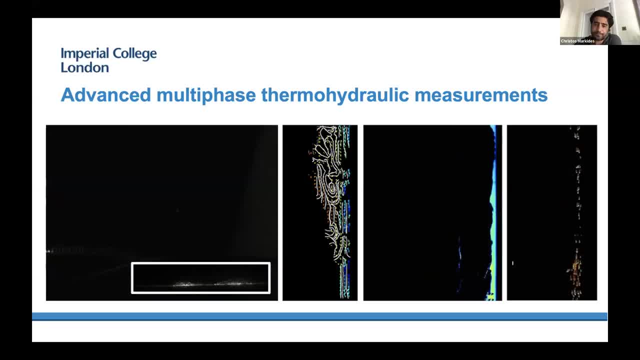 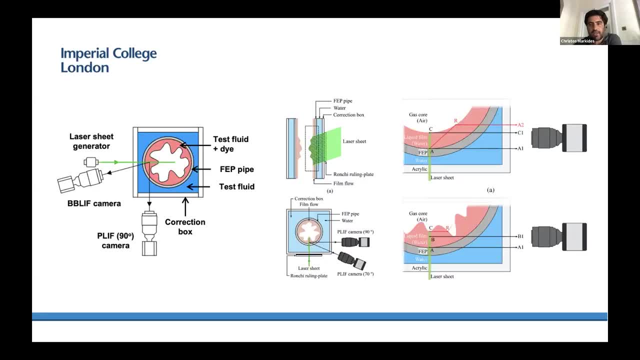 here is basically to to find out where the interface is and to provide velocity field information. um, if you have a um, a two-phase- here i'm showing the example of a liquid gas system- optical measurements, that which are required to perform things like piv in single phase flows, become 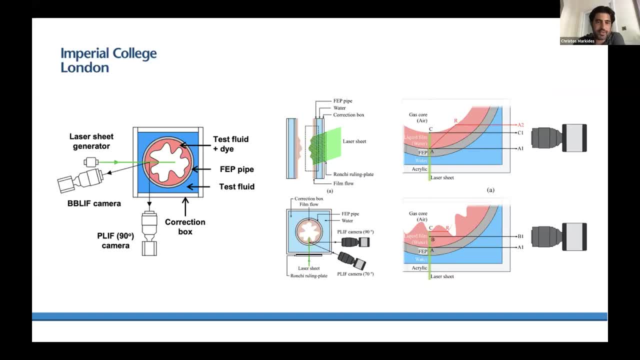 much, much more difficult because, of course, you have distortions wherever you have the interface. you have reflections, you have refraction of light and so on. uh, we've spent a good 10 years- 12 years, since i joined the department, basically developing techniques that allow you to do measurements in. 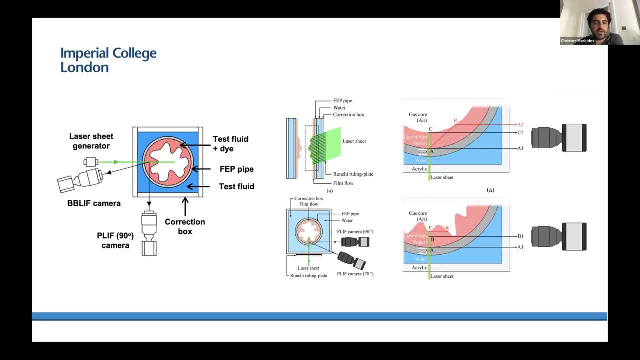 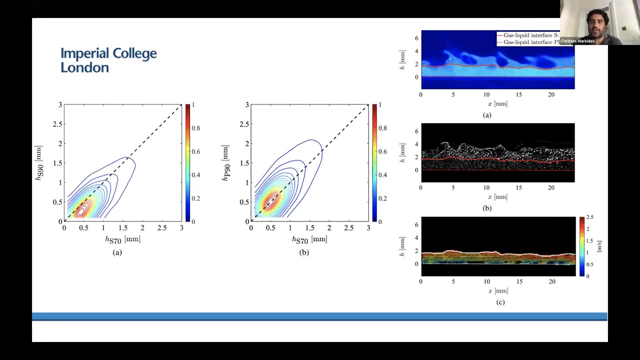 these types of flows and to measure velocities, uh, etc. and and interfacial locations, which gives you for the phase distribution in in uh, with different techniques and- and here i'm just showing one particular case where we're trying to measure the or identify the free surface of a film, where 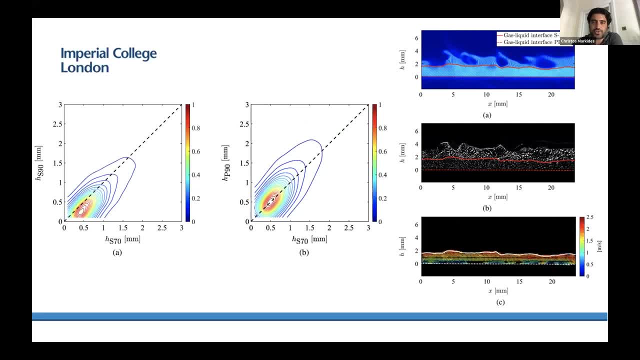 you can see that, um, the true surface of the film is actually hard to get. so we have techniques which allow you to find the real location of the film, everything else above this red line. i don't know if you can see my cursor, but basically this is called the false interface. 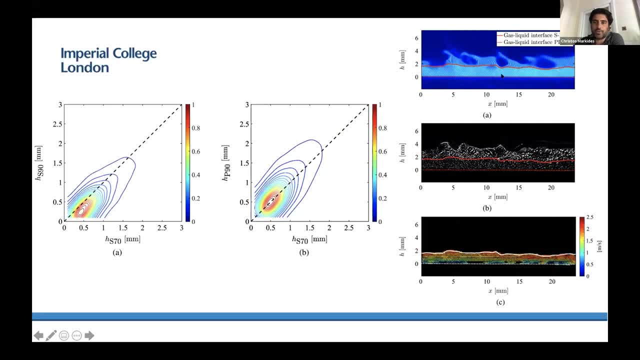 there's no real liquid phase over here. the liquid phase is only below the red line. uh, i think that really, the main point here is that when you're trying to do measurements in two-phase flows and in boiling flows- which i'm going to get to in a second- 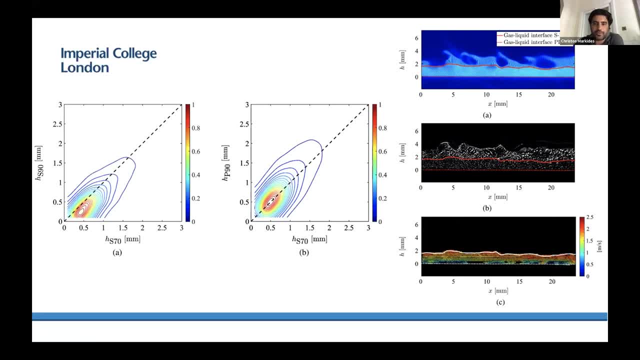 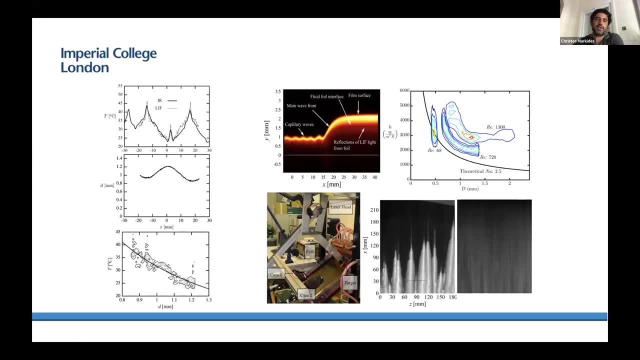 you need very dedicated experimental techniques, and we've trying to be trying to develop this for a number of years. um, so here's us basically going from just identifying interfaces and velocities to now starting to temperature measurements, and you'll have all sorts of techniques that allow you to do that, either based on laser methods, uh, so fluorescence, which is 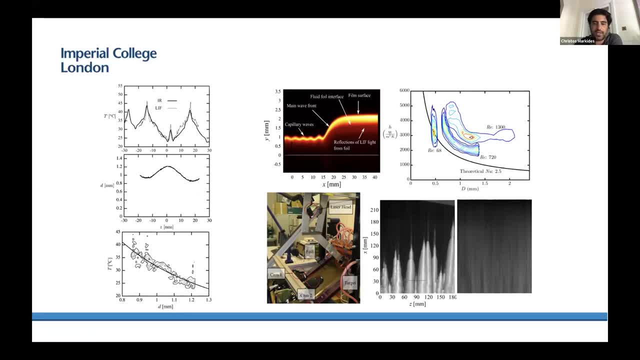 a dependent or infrared measurement techniques which we've been applying to different types of flows. here we have a film which we're trying to measure heat transfer coefficients in and i guess the interesting thing here for people who are on the call is the sort of space and time resolved. 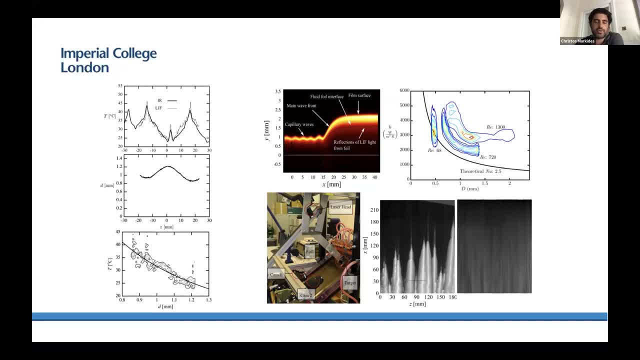 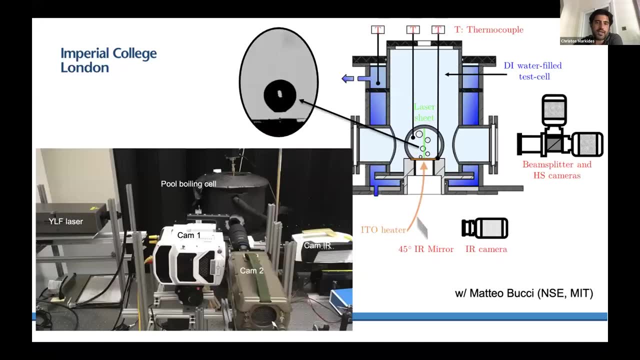 nature of these measurements right, so we can get a special distributed measurement of a heat transfer coefficient over some surface and time resolved, uh, and then effectively then taking these types of techniques and trying to look at uh, uh, a much more complicated flow. so this is, uh, boiling right, so pool boiling and this collaboration with matteo at mit. so this is. 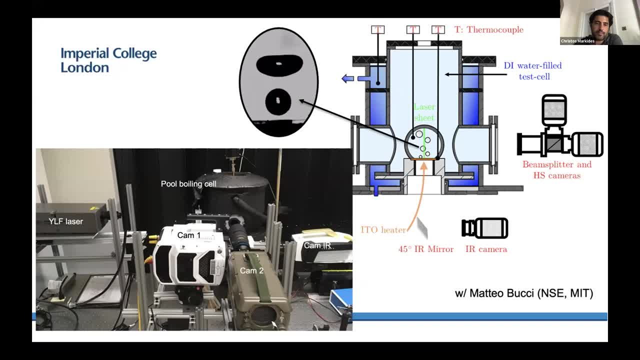 actually a work that was done at mit, um in the nuclear department there with, uh, some of the work in terms of applying techniques, that sort of we brought um and i'm going to show a few sort of typical- you know the type of information really that we're trying to get to with these measurements. 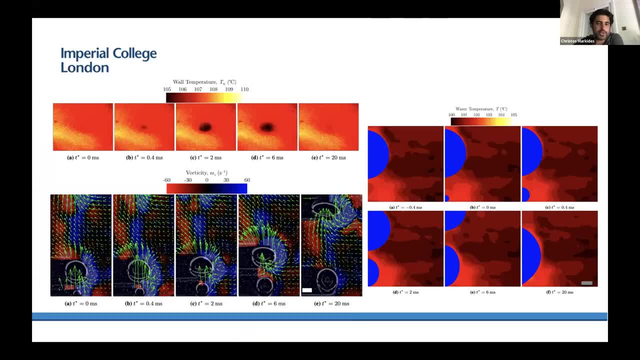 and so these are the other ips in in the emerging models of the front right and you can see that here. you see on top a bubble which grows and detaches from a surface. so you can see there that the wall temperature underneath the bubble uh is lower um. below that you see the velocity field around the bubble as this rises. so this is from a different camera angle. so the top image is looking down on the on the heated surface where the bubble rises and then detaches, and and the one below is looking at the flow field from the based. we can see the density in the bottom. so awards. 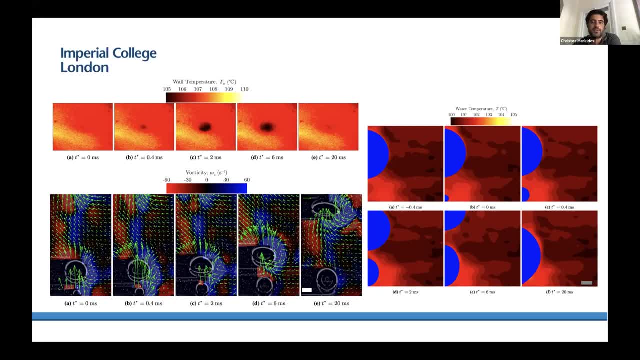 in the bottom we can see this dual sideotherapy. from the sideところ side you can see the temperature field around the bubble as this lifts off the surface. So this is to see things like temperature boundary layers and other sorts of effects behind the bubble as it. 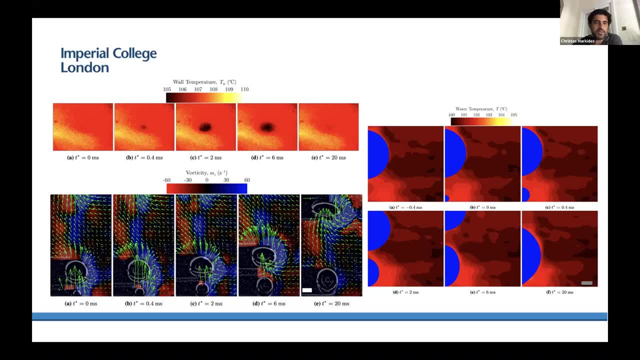 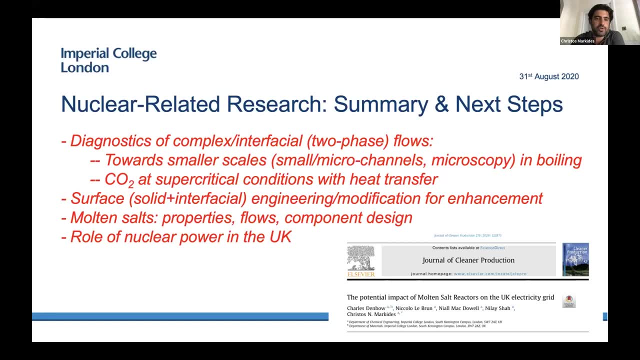 rises Okay. so I think that really summarizes what we've been trying to do and what are our next steps. We're trying to go. as I said, most of our experiments are sort of large-scale experiments. We're trying to go not just in terms of the size of the channel, but also potentially. 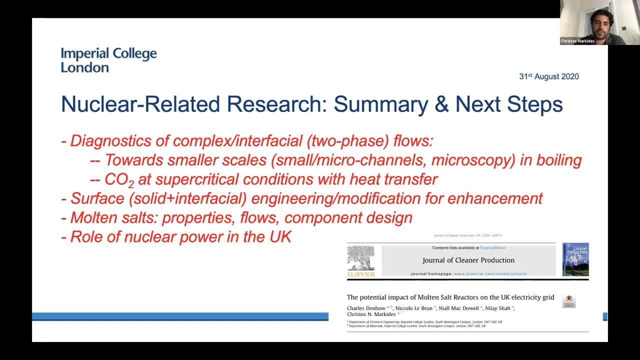 the measurement domain towards smaller domains. So we've got a microscopy system that we're building up at the moment and we have also an EPSRC funded grant on small channels that we want to kind of start applying these techniques to, and we're sticking with boiling. so we're talking. 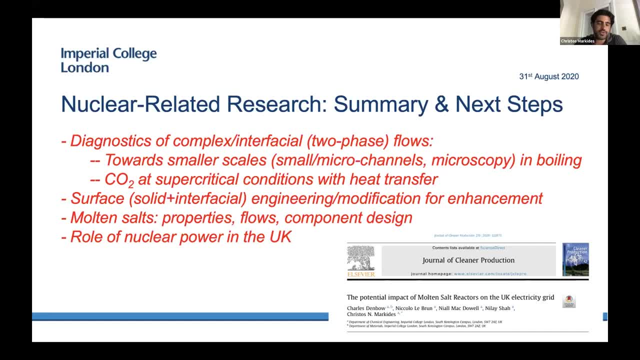 about two-phase flows. We also have an interest. we have a Marie Curie fellow who's arriving in October-November and doing measurements in basically in CO2 at supercritical conditions with heat transfer, and then you have buoyancy effects and a lot of difficulties again making 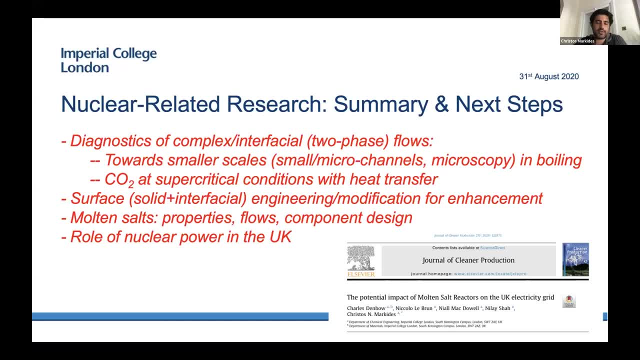 measurements We want to look at. this is basically work that Matteo does at MIT on surface engineering, nanoengineering, and to what extent you can affect things like heat transfer performance, let's say, at a very high level, through these types of modifying surfaces. 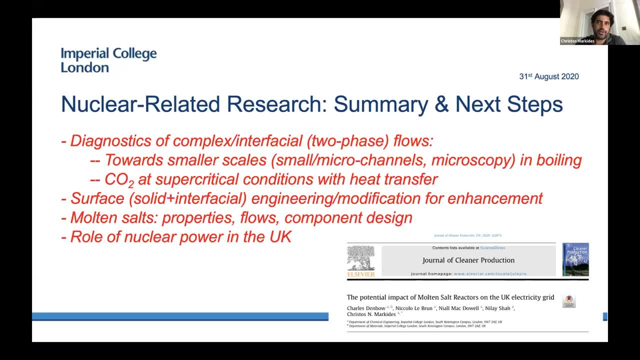 But also personally, I have an interest in the interface, so you know, whether through particles or other types of yes. Sorry, I have to interrupt you. I'm done. I'm done. this is my last slide. Okay, I think I'll finish it there. I'm done. Thank you very much. Thank you. thank you, The. 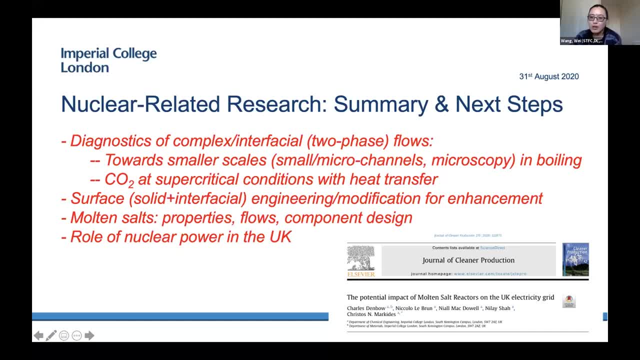 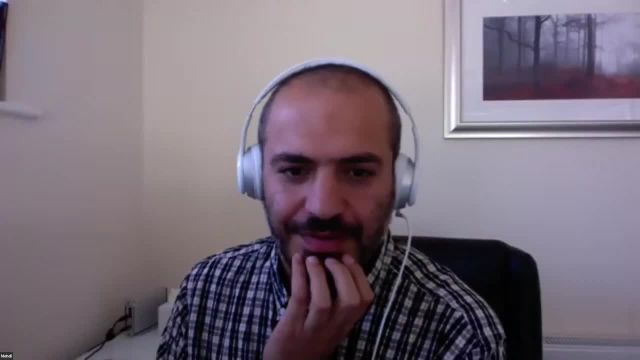 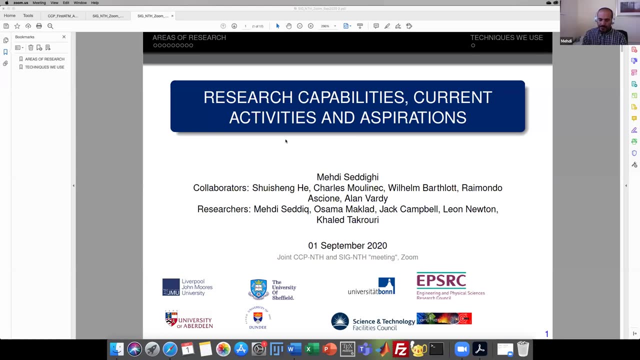 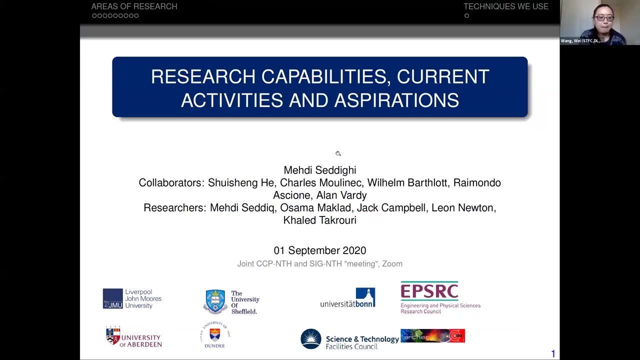 next one is Maddy from Liverpool, John Moore University. Right, let me see if I could share my screen. Is it all right? Can you see it? Yes, All right, brilliant, Thank you. thank you, Wei, And I think it's time to say good afternoon, I think. So, good afternoon everyone, and yeah, I'm going to briefly. 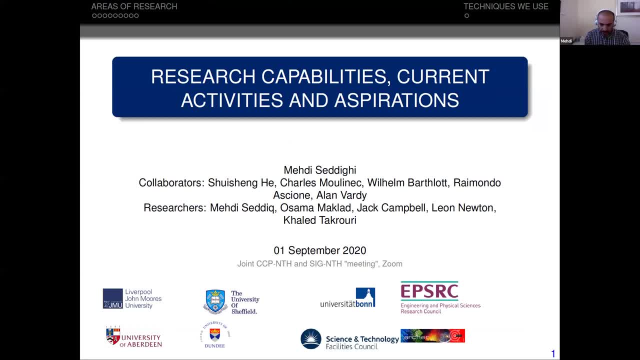 talk about. this is a very short summary of what we are doing and related to I mean thermal hot relics. This may be some recent and current fundamental research that we are doing and part of the work has been done. when I was working with Shushan Sheffield- working with him in some 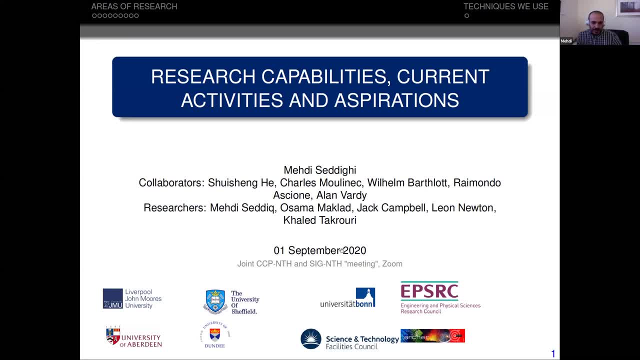 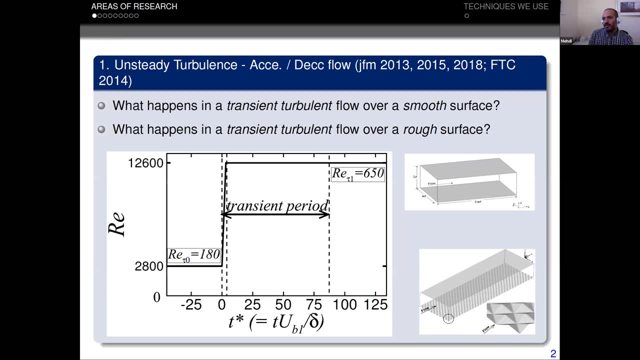 projects and some others with other collaborators, obviously a couple of researchers who are helping and doing research on this mainly. And yeah, the first topic is on the turbulence when we have non-periodic flow, So we have one turbulent state and at some point we accelerate this area to another. 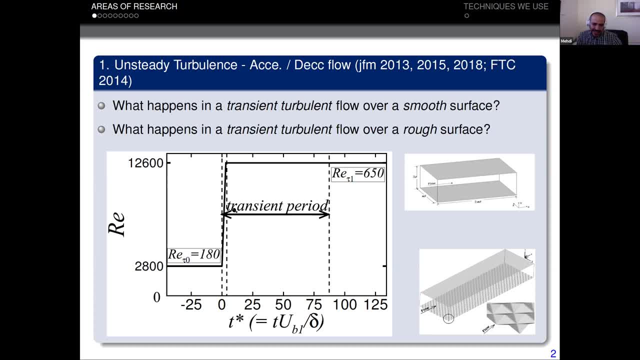 turbulent state and there is a time following that acceleration or deceleration chain that we call it transient period and during that period it I mean the flow will change to reach to the new turbulent stage. We have done research on smooth surface and rough surface. for this I mean type. 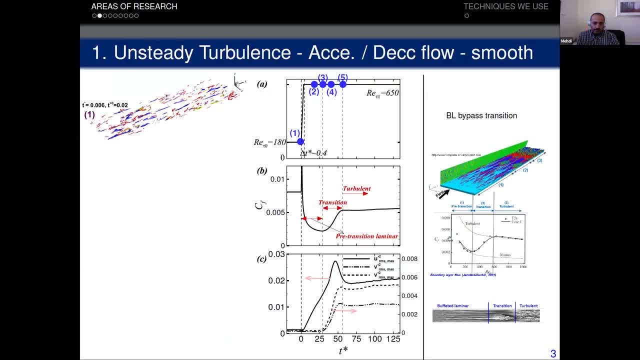 of flow and for the case of smooth surface there is. I mean, although despite the initial state is turbulent, the flow has shown a laminar to turbulent transition, a process which resembles there what we see in the bypass. So it is an event of an event of a transition. 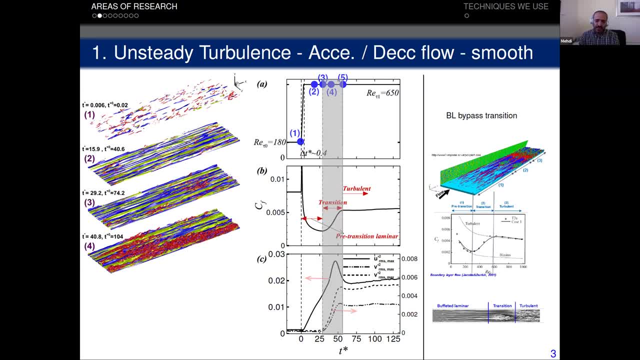 So there's lots of details on that. I have shown that three states of pre-transition, transition and turbulence states have have been shown by the flow following that acceleration. Again, this is this part, the fact that the initial stage of the flow is turbulent. 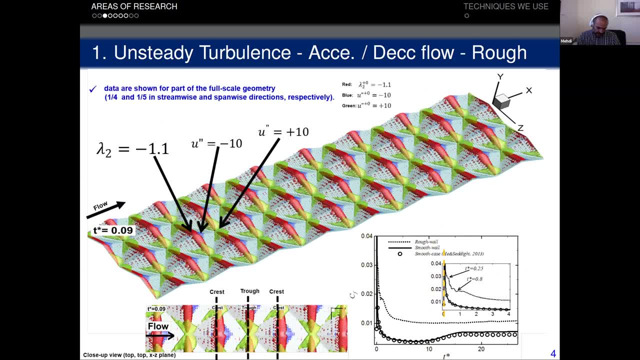 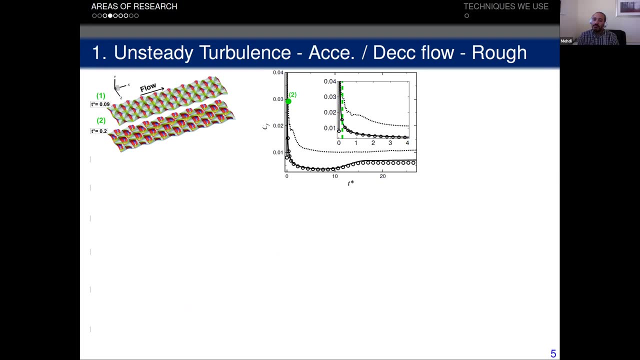 So we did also the- I mean the research on, on when we have a rough surface and the roughness is modeled using a simplistic- I mean pyramid roughness, and again the initial flow state was turbulent, although at I mean quite low in terms of I mean the roughness definition, that is, at low, I mean near the 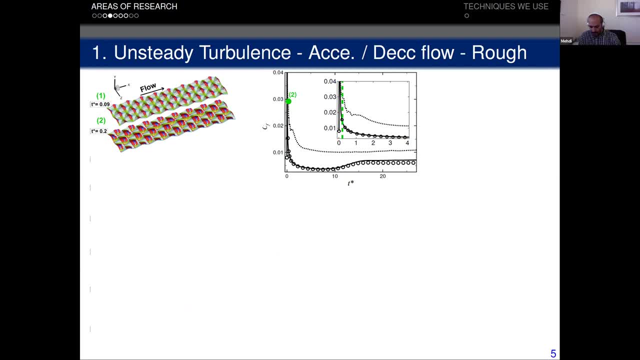 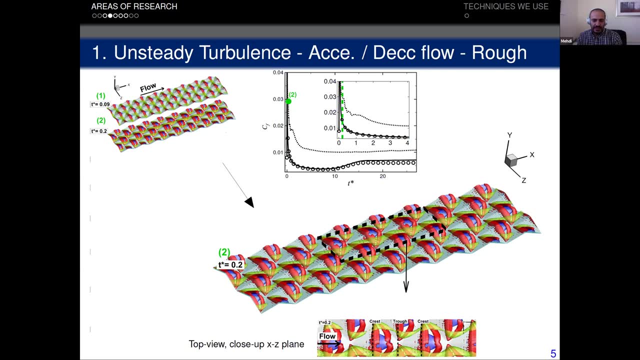 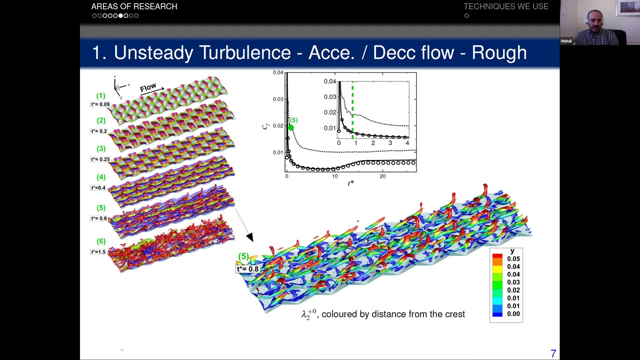 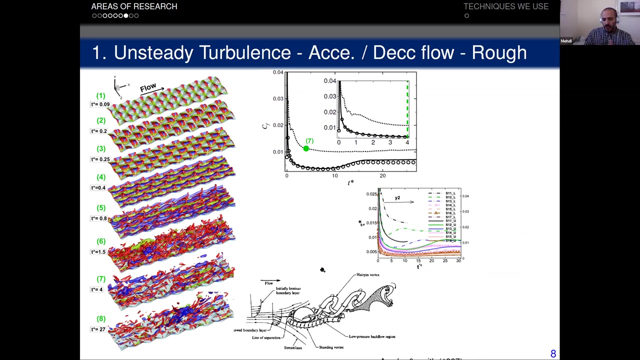 high radius, smooth region and then we accelerated the flow to nearly fully rough regime and again, in terms of procedure, we can see that is, I mean similar behavior have been shown for the development of turbulence and which is resembles, again, roughness induced transition. so, on addition to that, because all of the things are for turbulence onset, 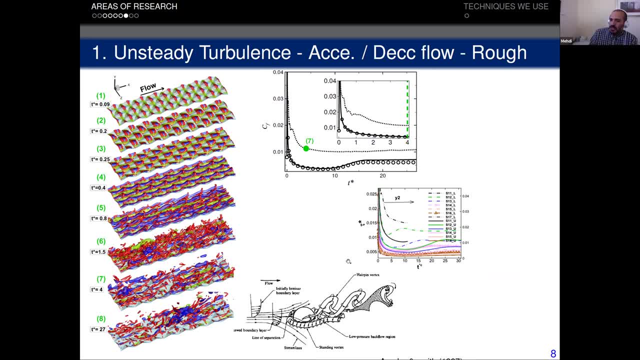 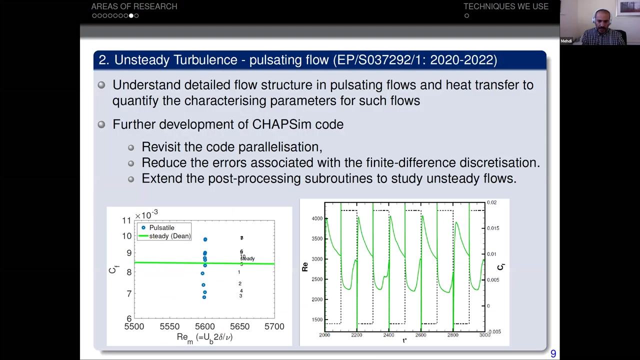 but we have accelerated, accelerating individually and obviously we have done that for some other other flow, condition that it is not only towards the fuller of regime within the transition of regime. there are also some, some some research we have done on and the other I mean type of research on our study that we have just started. 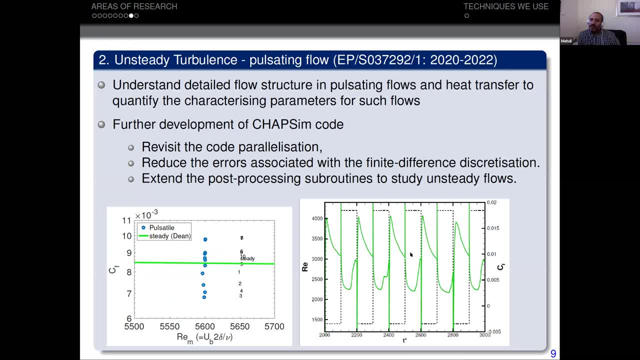 together with DFC, Charles Mullinek is to look at, I mean, pulsating flow. again, in pulsating flow there's lots of literature already, but this is, I mean, some contradicting sort of things presented in terms of how pulsatoid flow I mean affects the heat transfer as well as 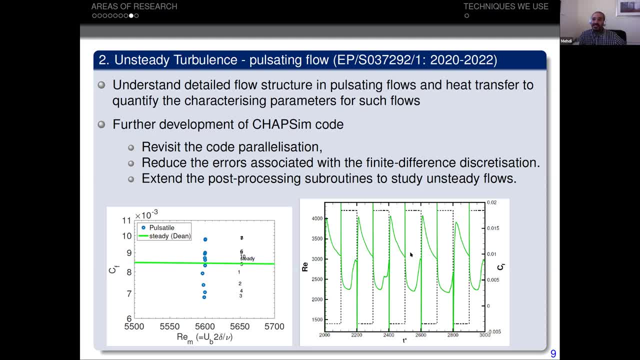 flow only cases. in some cases they show enhanced heat transfer, in some cases it's suppressing the heat transfer. so we are looking at that To understand the flow structure and flow and heat transfer performance when we have pulsatoid flow in terms of the, the computational and the code development part, we also look at 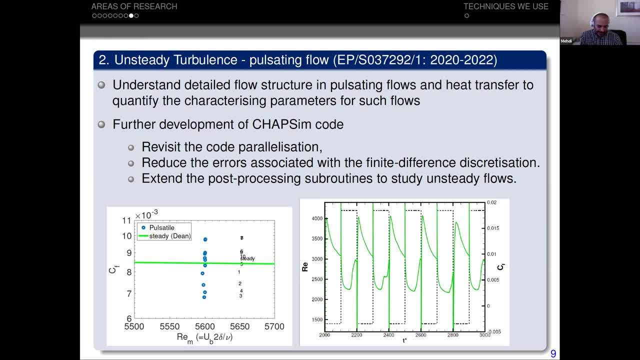 some modification to Chapsim that I'm sure you already probably aware. I mean a few times by Wei and Xu Sheng that are the full polarization- and Wei has already started that And some, some other aspects of the code development that we are going to contribute to- is to look at to improve the, the, the spatial discrimination. 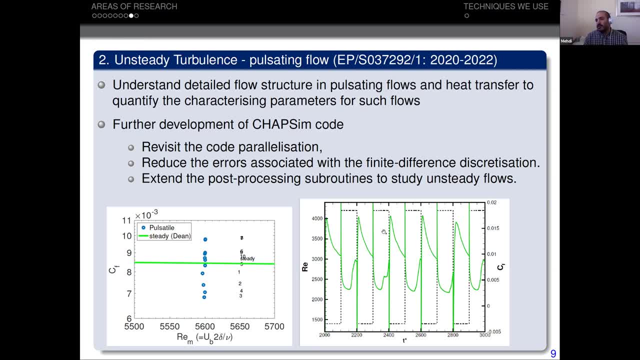 error. and also we got, I mean, quite many post-processing subroutines, as, as Wei mentioned earlier in by developed by different users, but we are going to combine them and make them in one subroutine. So, in particular, the main focus is really is to look at their own study flow, and when I talk 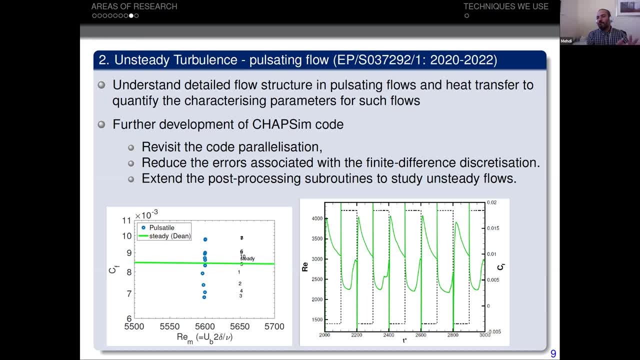 you know, say almost study, I mean changing, mean flow, not instantaneous, which is obviously. I mean changing. again in terms of drag, reduction is always shown. this is for some particular amplitude and a period we see some direct reduction. but again, this is something that we're going to look at. 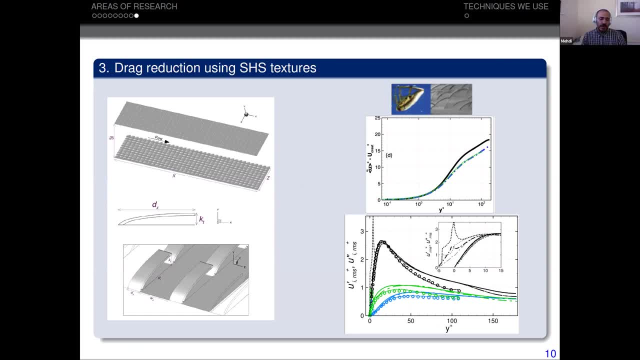 and, yeah, this is also a very important slide. The other type of research that we are doing is to look at some drug production using super hydrophobic surface. This is a research that we are currently doing and just getting some volumetric text surface using that back swimmer and we got some quite interesting and promising. 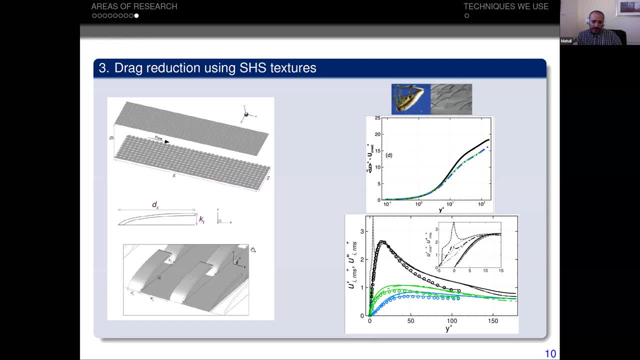 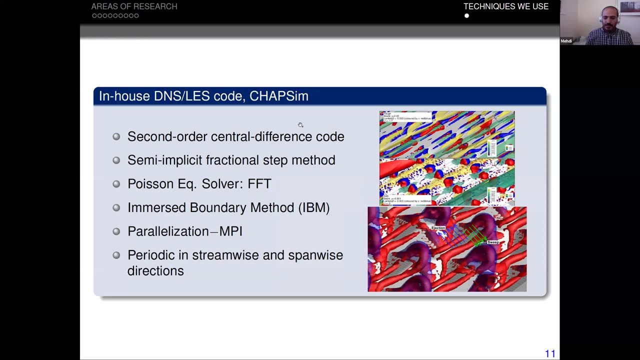 results. This is a simplistic model for that back swimmer and we got quite significant rapid action. In terms of the methodology, I think I don't need maybe to explain that much. Wei has already indicated that we use Chapsim and is now for more than a decade that is under development. 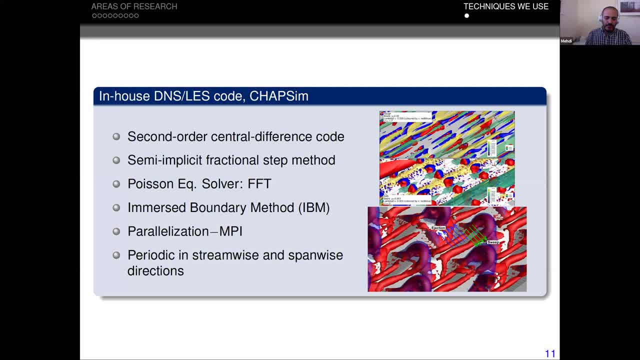 by different people, and we are also aiming to improve it. I mean more and more over this CCP project as well as this EPSRC project that is working on the Pulsar Typhoon. Thank you very much for your attention. I want to stop now. 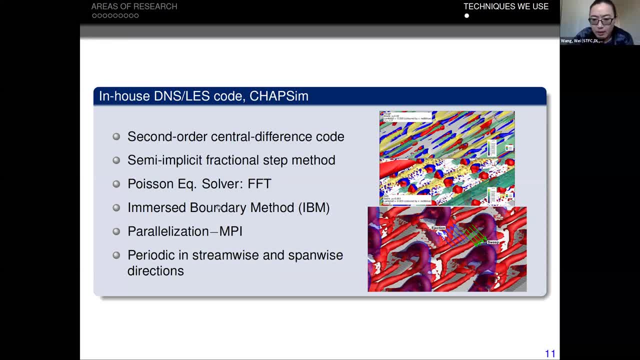 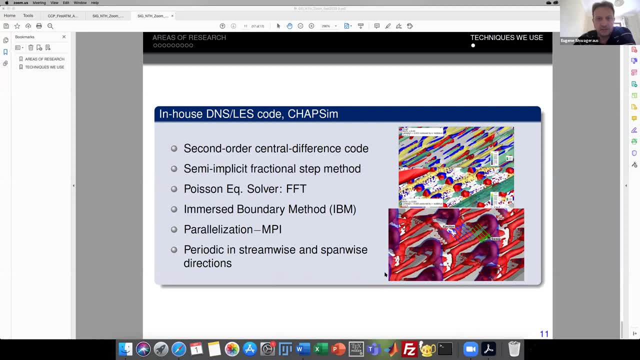 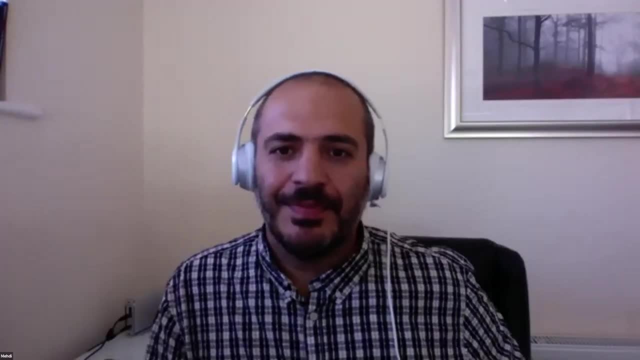 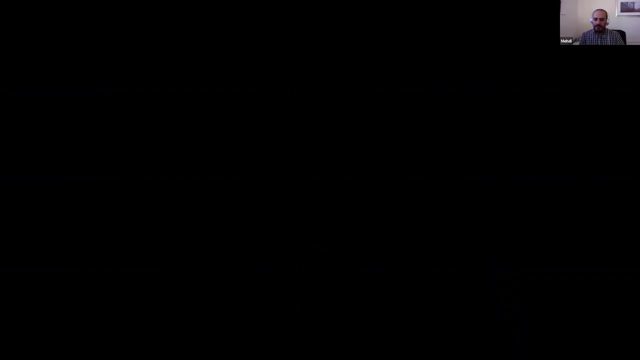 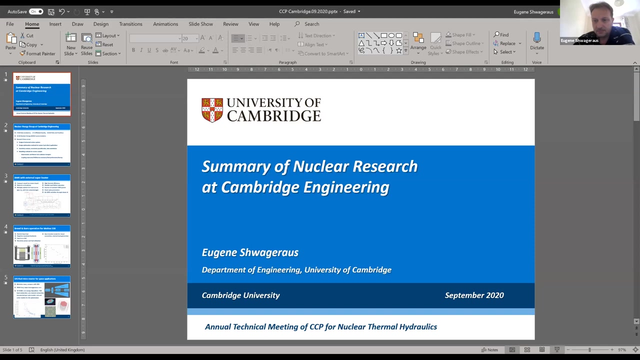 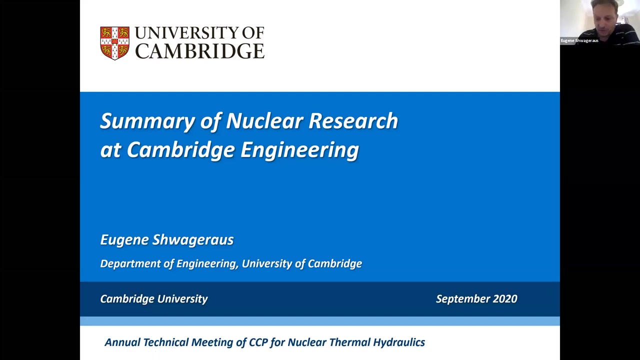 Thank you, Maddy. Our next presentation is by Eugene from University of Cambridge. Hi everybody, So let me see how I could stop my stop. share, Okay, can everyone see this? Okay, so this is an overview of Cambridge University engineering department activities. 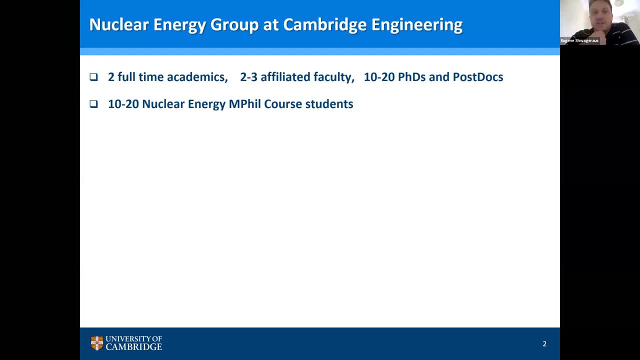 I should say that this is not a reflection of what university as a whole is doing. There are various bits and pockets of activities in other areas like materials policy and economics and so forth. So in engineering we are pretty much only two full-time academics with two or three affiliated faculty and 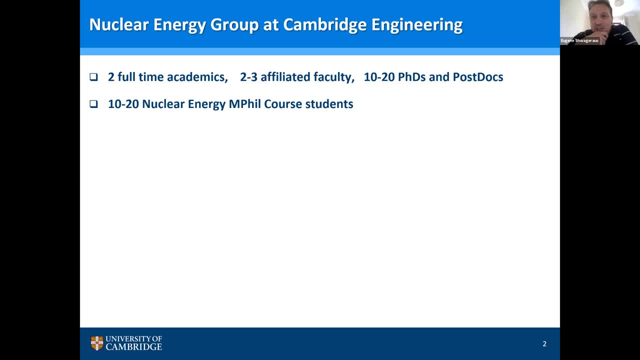 at any given point in time we will get all the information that we need. So I would like to say: anything you are aware of could help, so I am not sure where the word that you're going to get is from. given point in time, we're between 10 and 20 PhDs in postdocs graduated, quite a few recently. 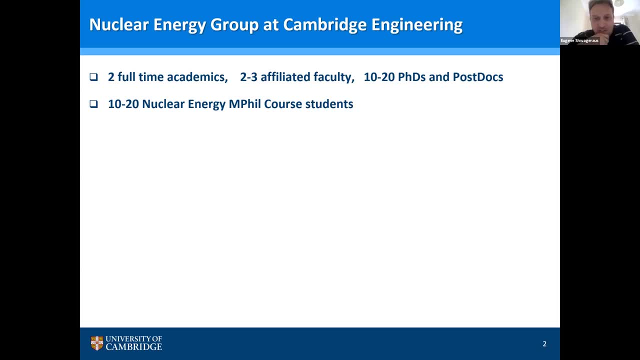 so we're in the bottom of the cycle at the moment and hiring. Another thing to mention is nuclear energy master's course that is run out of engineering, which I'm directing, and that's a lot of master's level dissertations to supervise. So in terms of research areas, 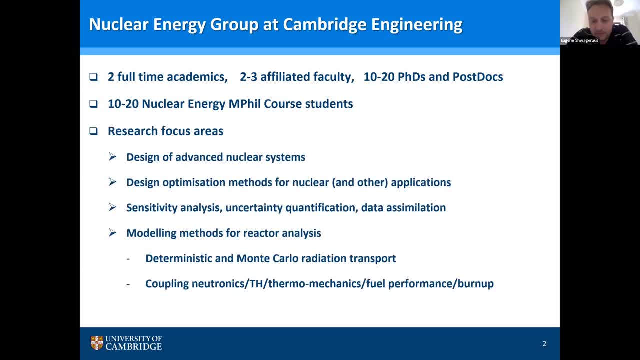 we're more of practitioners of thermohydraulics models aiming at the design of nuclear energy systems, and the emphasis here is on systems because it requires not just thermohydraulics but other things. My colleague, Jeff Parks is well known in design optimization methods which can be applied to 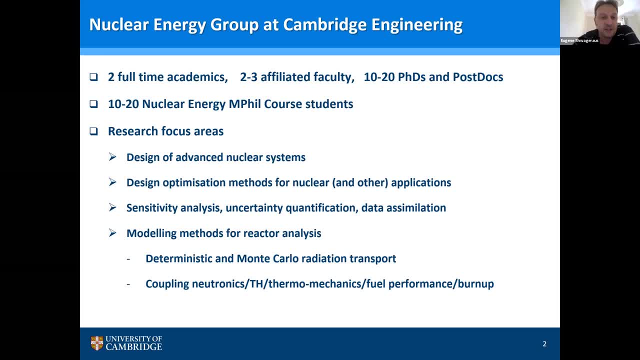 nuclear but also other applications, And engineering department also, as many of you may know, have academics who are not actively involved in nuclear but with a wide range of knowledge and expertise in thermal fluids development, and at uni they are deep in that field, and so are researchers like Peter. 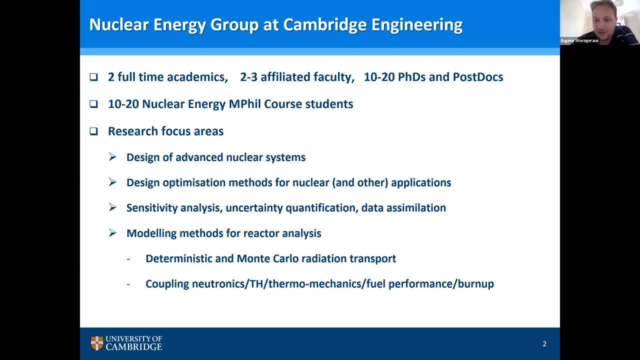 Davidson and our fluids network. Matthew Juniper was a leader- I don't know where he still is- and few others. So these are the areas of activities and I will just briefly mention a couple of recently completed PhD projects to give you a flavor of what we are doing in this direction. 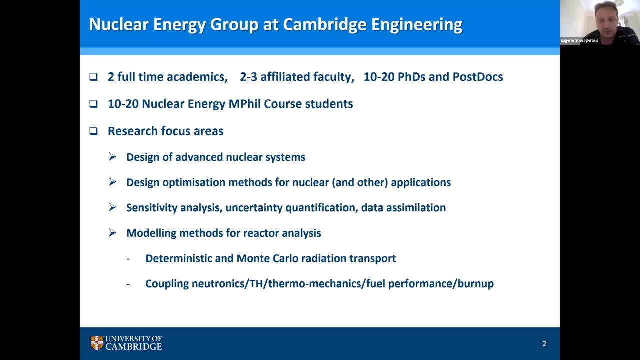 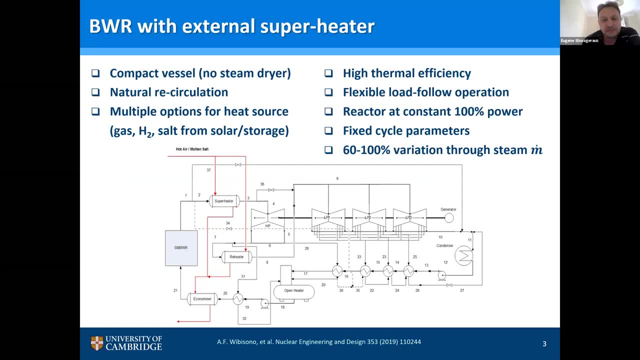 alah been doing So. one project is on BWRs with superheater. Some of you may remember Ferry Urisono, who was a PhD student in the group, participated in a nuclear thermoeutronics interest group live meeting a couple of years ago So he presented some of his work. So the idea is 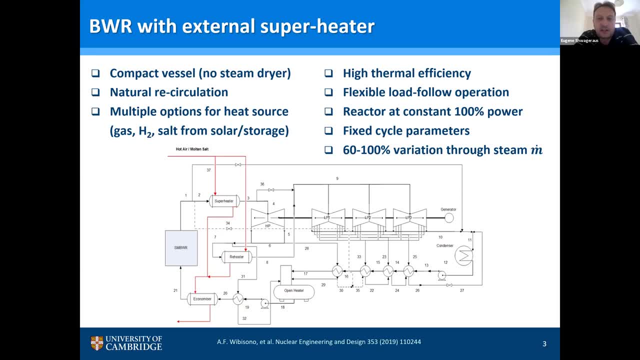 to attach a superheater to a BWR, which allows improving many design characteristics of such a system So it can be smaller, it can improve thermal efficiency of the whole thing and load follow and so forth. So this required a range of couple tools that has also have to run sufficiently fast. 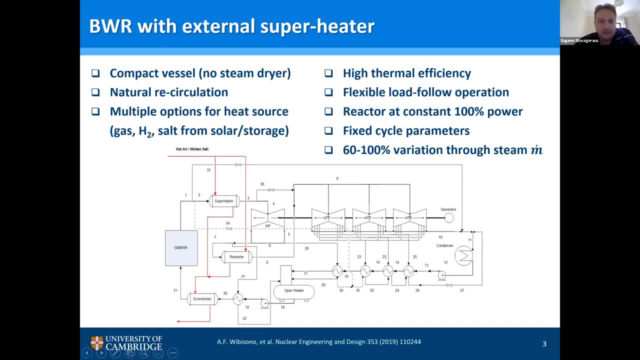 to allow full system optimization. So thermodynamics of power cycles, coupled to various effects that it will have on the nuclear reactor system which, through this superheater, can run at 100% power 100% of the time And load following, is enabled by this variable. 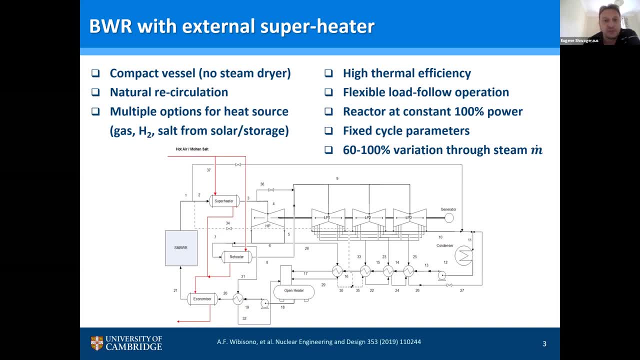 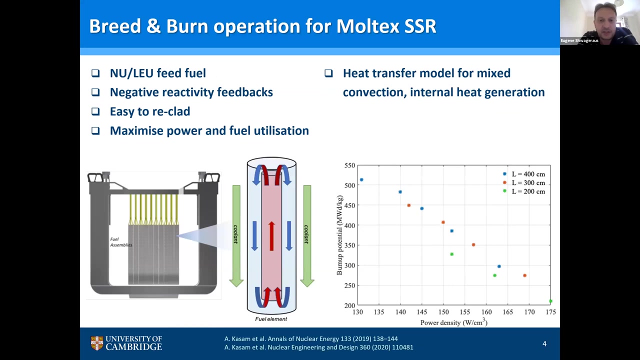 heat superheater that can draw its energy either from burning natural gas or hydrogen or ammonia, or using heat stored from things like concentrated solar. So this is the third example. Another recently completed project is that required several sort of different angles of expertise is molten salt tractor, more in particular Moltex version of it. 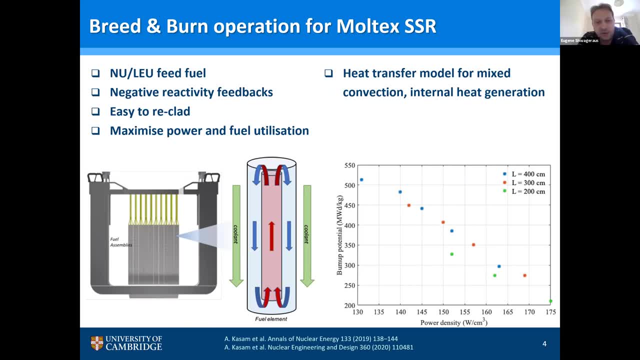 Some of you may be familiar. So this is a concept that uses molten salt as a coolant, which is encased in relatively thick fat fuel pins, and the clean salt as a coolant which removes the heat. So the trade-off that we were trying to evaluate was so some of you may know that Moltex is. 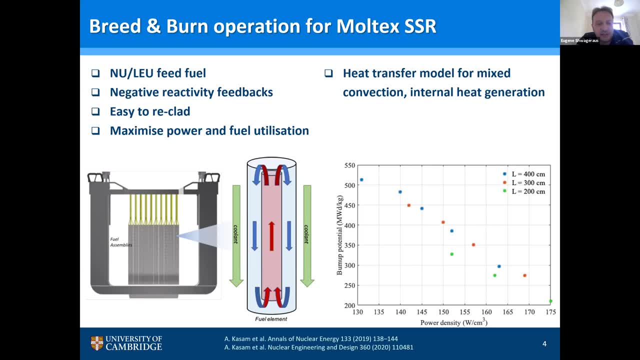 designed as a burner reactor, we were trying to see whether it can be a breather reactor. so we want to try to breed actinides and improve fuel utilization. So it was apparent from the beginning that it should come at some cost of achievable. 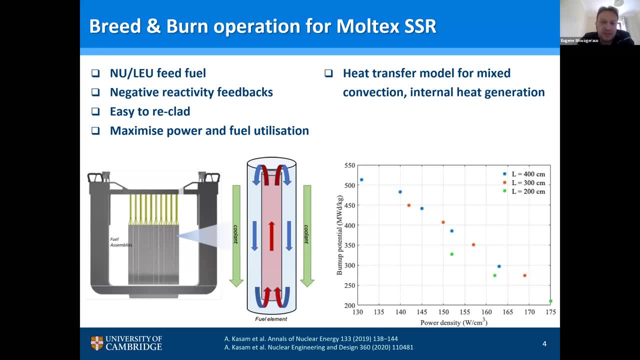 power density, which is the main driver of economics of the reactor. so this breathing potential versus power density was a very interesting exercise which required a wide range of models to work together Through coupled interfaces. So one of the more interesting things were development of heat transfer model for this. 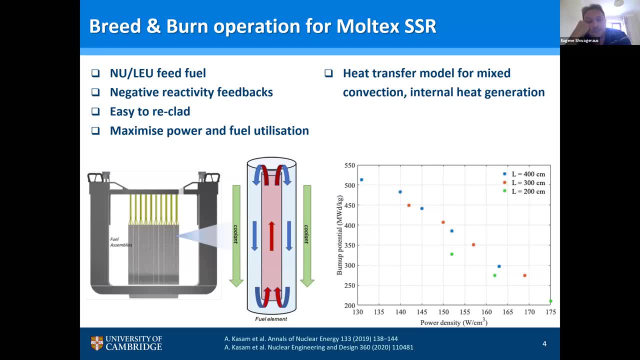 naturally circulating heat generating fluid within a pin, which is then that heat is removed by water. We figured a downward flow of the coolant is beneficial because that enhances the circulation and allows greater heat transfer. so lower the fuel temperature. fuel salt temperature. 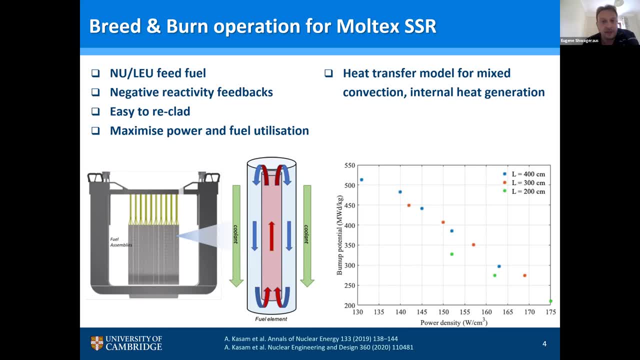 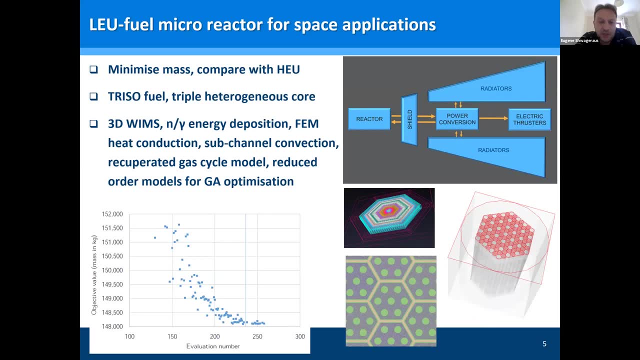 and, as a result, allowing a higher power density. Another exercise which was recently completed is- I don't know if you've heard of it, but it's a very interesting exercise. It's a very interesting exercise. It's a very interesting exercise. 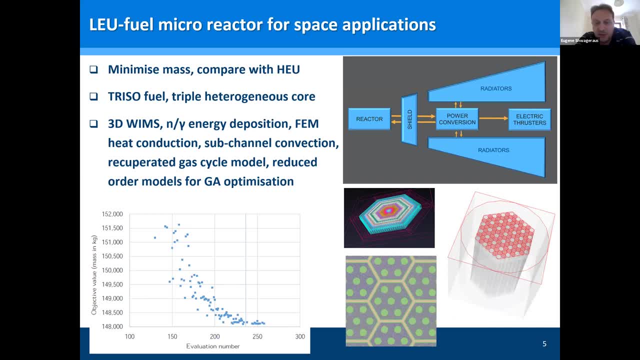 It's a project done for NNL as part of their collaboration with the European project on space reactors. So this is another sort of multi-physics exercise that required both nuclear fluids, thermo-hydraulics and power cycle models all working together. 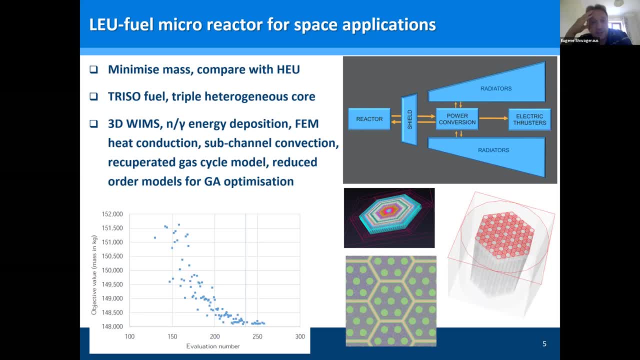 It's a very interesting exercise. It's a very interesting exercise. It's a very interesting exercise within reasonable time and to be fed into a genetic algorithm optimization for evaluating minimal mass, which is obviously critical for space reactors. The main question was: all space reactors used to use highly enriched uranium in their 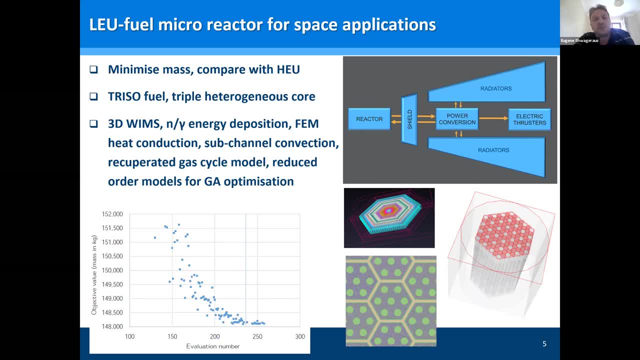 course, which is politically problematic, and we wanted to see what will be the mass penalty If we switched to the non-nuclear one, to low enriched uranium. So it will be heavier, but we didn't know by how much. So by having 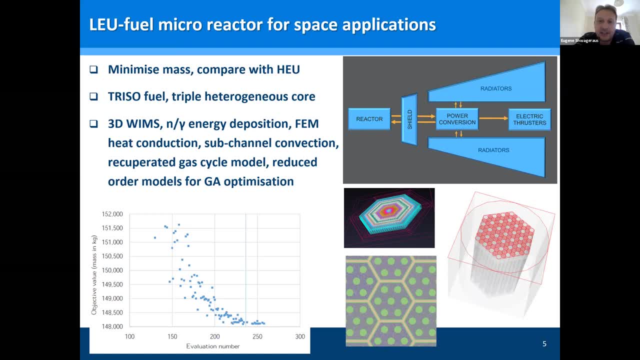 a pretty detailed model of power cycle and heat exchanges, the radiators and so forth. So coupled multiphysics models allow that optimization to happen. So we came up with a reasonable answer. I will be happy to expand on any of those And thank you very much for. 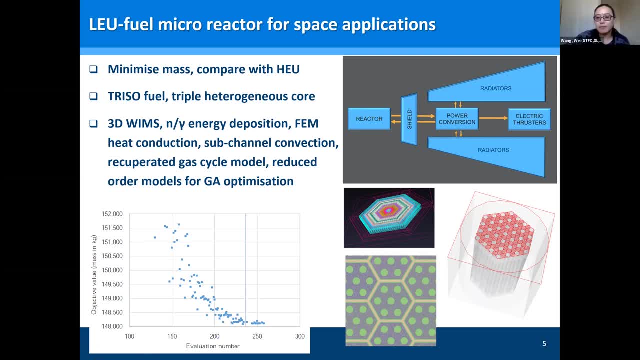 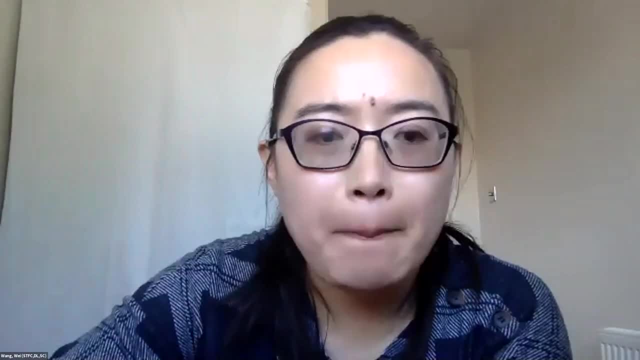 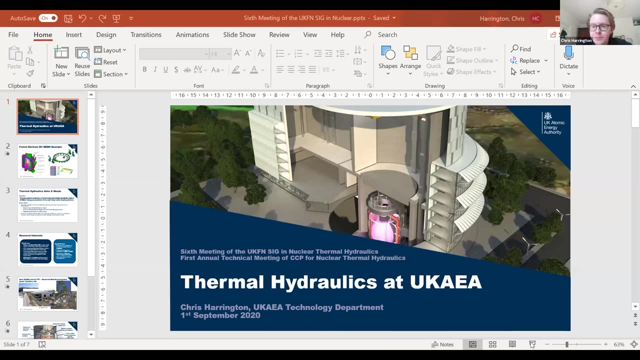 your attention. Thank you, Eugene. The next talk is from Chris Harrington from UKAEA. Thank you, Let me know if you can't see that. Yes, Okay, thanks everyone. So my name is Chris Harrington from UKAEA. 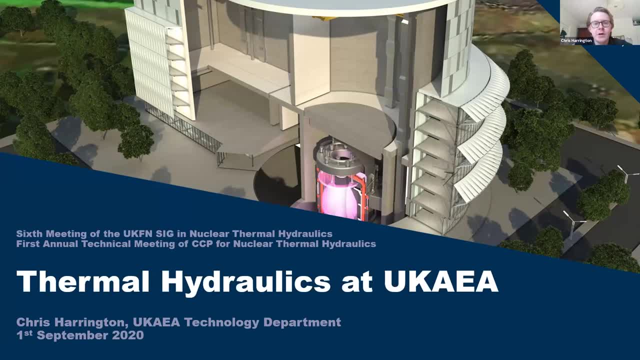 This talk is a bit of an overview. It's quite broad and not too detailed on our interests at UKAEA. Our mission is to realize fusion power but to, in doing so, explore enabling technologies, of which thermohydraulics is obviously a big one. So there's strong overlaps. 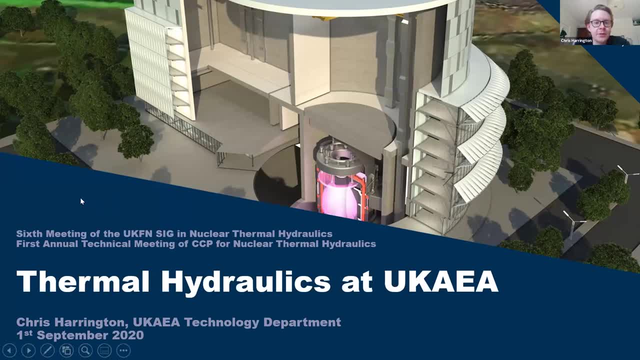 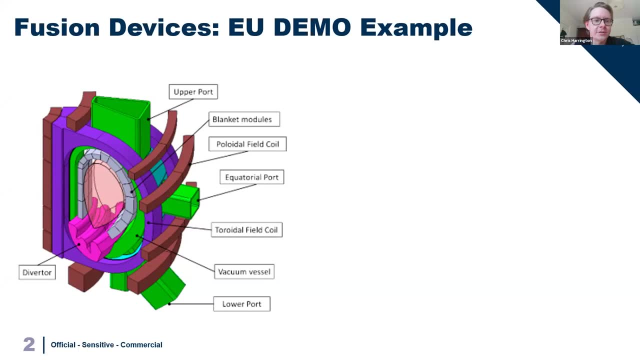 with fission, but also some quite unique challenges as well. So I'm going to start just by talking about the basics of a fusion reactor. A lot of you probably already know a lot of this, but I don't like to presume. so it's always good. This is taking the EU demo project as 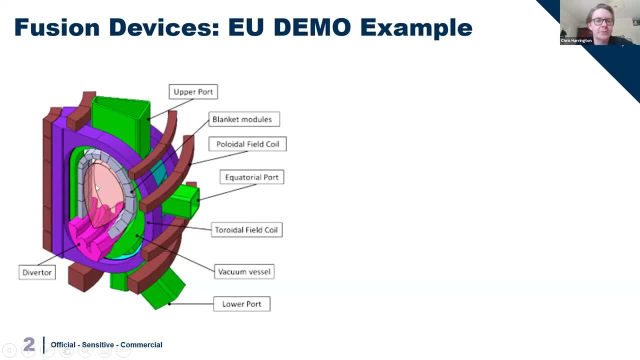 an example. Effectively, we have a torus-shaped machine, of which you can see a segment here: a burning plasma in the center, confined by strong magnetic fields, And around the wall of the machine, in this gray area divided up into blocks, is a component we call the. 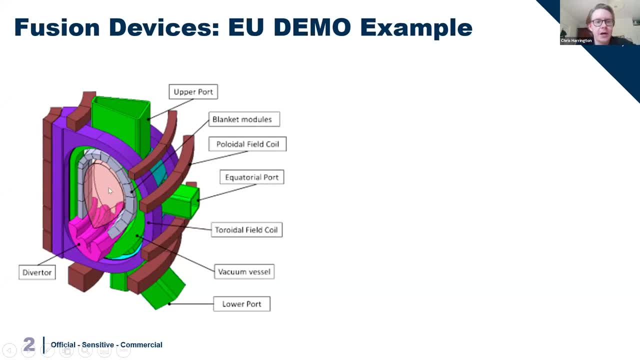 blanket That absorbs neutrons, Okay, Okay. And in doing so it becomes hot and the challenge is to extract the heat from that blanket, turn that heat into steam or some other fluid to dry the turbine and use that to generate. 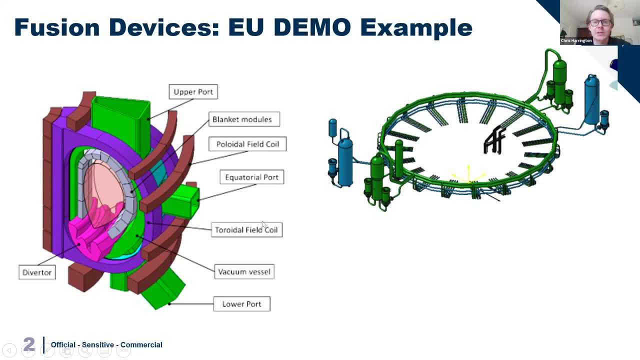 electricity. So that's the internals of the machine, but that obviously has to be supported by a large range of other systems Outside the vessel. this is showing one particular design for a water-cooled reactor where we would have this quite large water-cooled reactor. 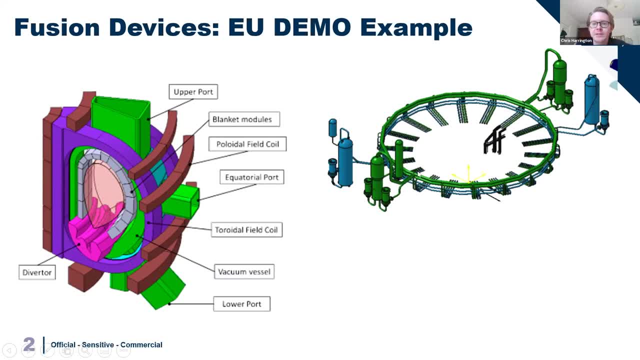 quite large and quite complex ring header system with various piping channels coming down from that and eventually connecting into the upper port of this machine. And around the outside you can see standard components that you'd recognize on a fission reactor, such as a YouTube steam generator, pressurizers and so on. 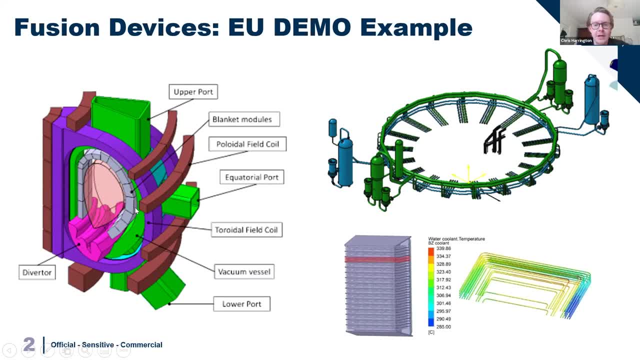 The blanket components themselves. these gray blocks that we're looking at on the left might look something like this. This particular one, again, is water-cooled. It's effectively a steel box full of molten liquid metal. Okay, It's a lithium-lead eutectic. That liquid metal is circulating slowly and getting hot. 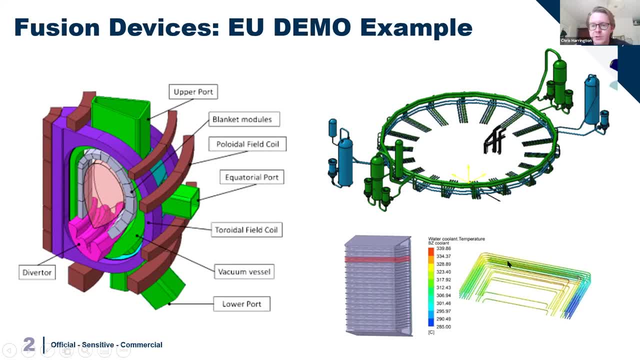 So, in order to extract the heat, there is a network of pipes- U-shaped pipes- running horizontally through that And through there we are running liquid water, pressurized water and PWR conditions to extract the heat. So you can see the scale of the problem is everything. 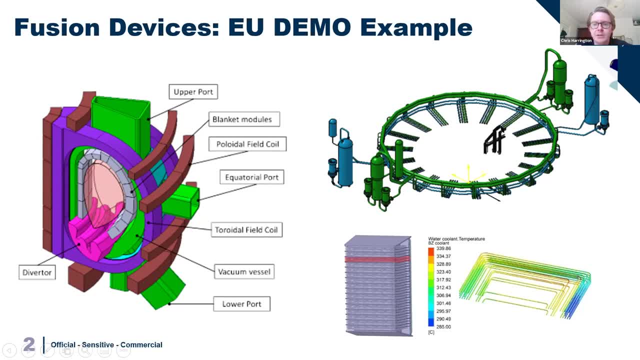 from this very large circuitry up at the top, which then breaks down into various branches all the way through into smaller channels, to extract the heat from a breeder blanket component And within that you've got liquid metal heating up in a strong magnetic field. 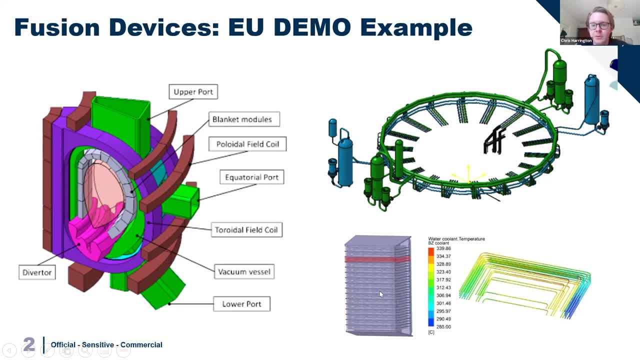 So there's MHD effects, You've got heat transfer from the metal to the pipe board, to the water, So you've got all of these very complex problems. plus you've got neutron bombardment and a non-uniform heat distribution through the axis of this component. 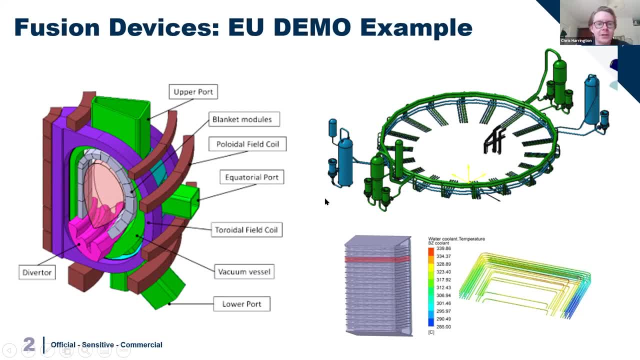 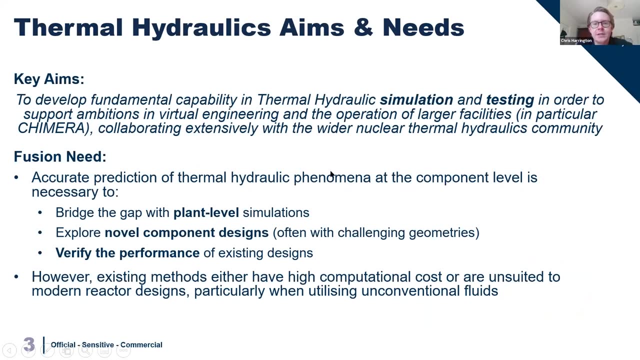 Okay. So the question we're trying to get to the bottom of it is: how on earth do we simulate, test, validate a power plant that looks like this? So, in terms of our aims at UKAA, what we're looking to do is develop the capability in. 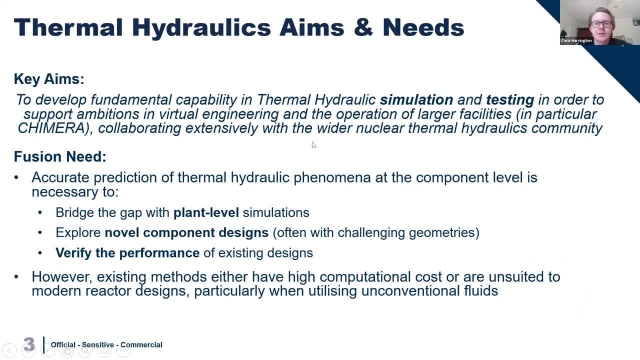 both simulation and testing of components for virtual engineering and the operation of some of our facilities. The big one that we'll come onto in a bit is called Chimera, And we want to do this collaborating extensively with other parties- Okay, Universities, industry groups and so on. We're aware there's a lot of excellent expertise. 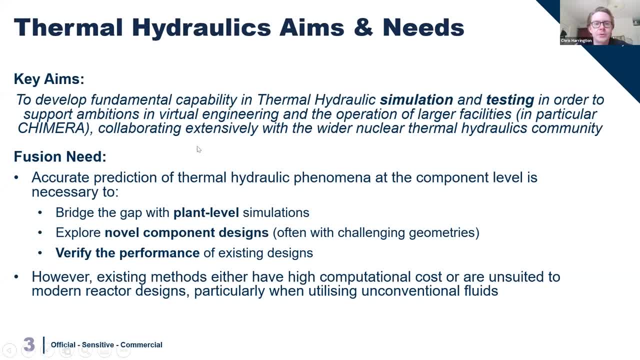 out there amongst a lot of people on this call. So really we want to work with others where we can, and hopefully the CCP is a prime opportunity to do that. In terms of particular needs, we need to bridge the gap with plant level simulations. So that's what I'm talking. 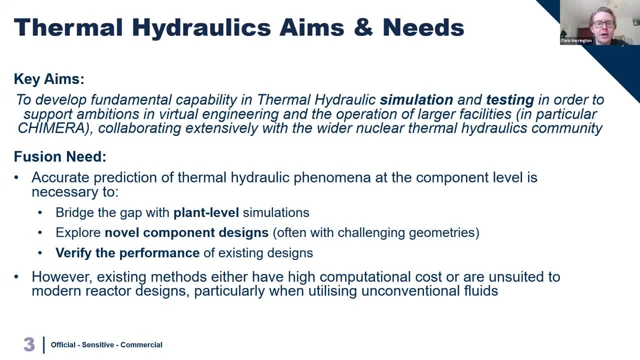 about when I talk about that larger loop, but also breaking down the simulations into more detailed simulations of the blankets. Okay, We need to be able to explore different designs of components, often with challenging geometries. So that water-cooled blanket that I showed you is just one design. There could be many. 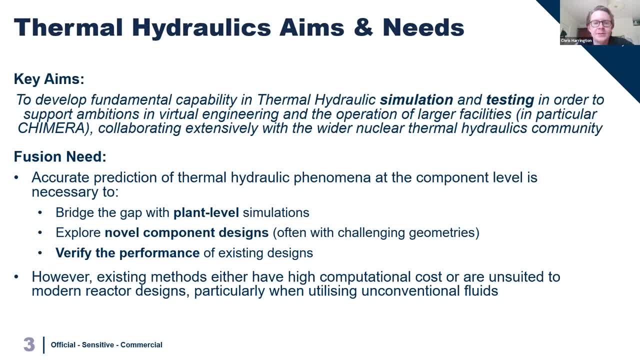 others involving fewer pin type arrangements or pebble beds, And then even within that, there's optimization to be done in terms of geometries, sizes and so on. We need to be able to do all of that design work and we also need to verify the performance of existing. 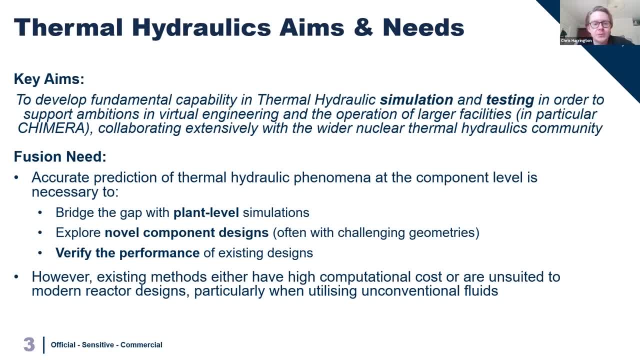 designs, So that involves putting them under test conditions. A lot of the methods that we have at the moment at UKAA we have a reasonable base in thermal hydraulics. It tends to be a little bit in pockets around the organization and 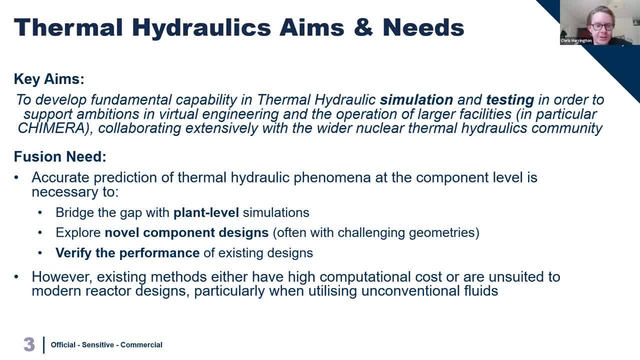 we tend to use either system codes or quite industry standards, CFD tools such as ANSYS, fluent- A lot of these are okay, but really we need to take that to the next level, And that's what we're aiming to do over the next few years. Our priority areas are listening. testing and monitoring. So that's what we're aiming to do over the next few years. Our priority areas are listening, testing and monitoring. So that's what we're aiming to do over the next few years. Our priority areas are listening, testing and monitoring. 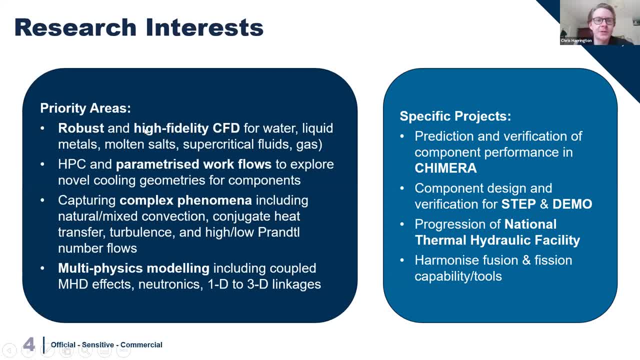 So that's what we're aiming to do over the next few years. Our priority areas are listening, testing and monitoring, And that involves a robust and high-fidelity CFD. were a pinch those words from the CCP, because it very much is about that, But specifically that we need. 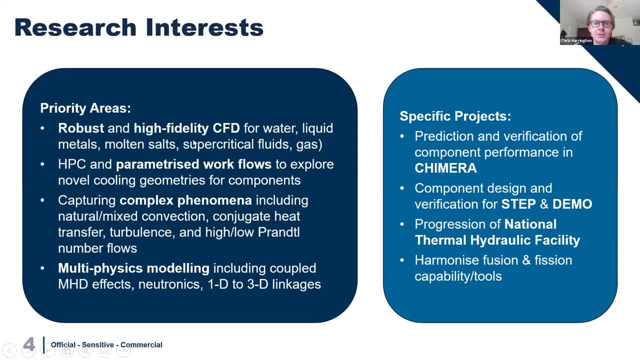 to be looking at: water, liquid metals, potentially salt, supercritical fluids, So the whole range of possible fluids that could realize a fusion reactor. We need to exploit high-performance computing and parameterized workflows so that we can come up with designs of different invessel components but also tweak those designs and 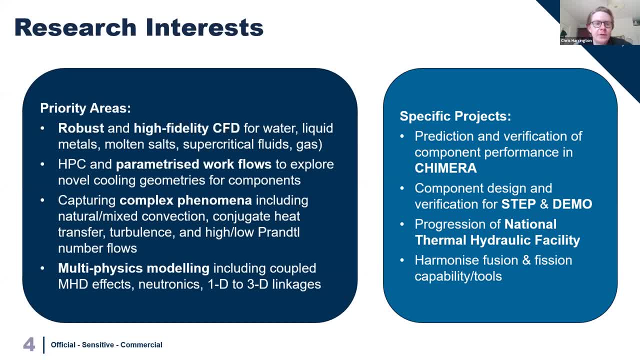 optimize them possible. to improve the heat transfer, we need to be able to capture complex phenomena, so that might include natural or at least mixed convection, conjugate heat transfer and high and low parental number flows, particularly relating to molten salts or liquid metal usage, which might be 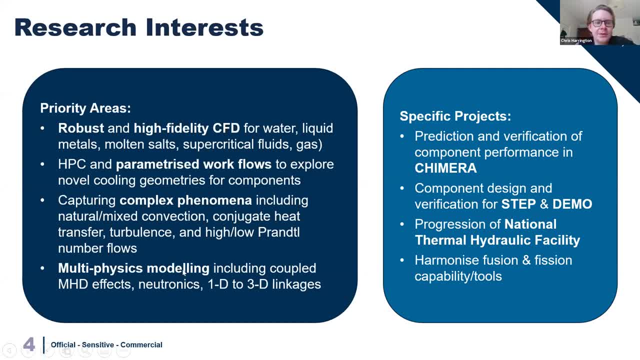 very enabling for a fusion power plant. and that that last point there is about linking all of these things together. so mhd effects if we're talking about liquid metals in magnetic fields, neutronic simulations and going from the system code to the cfd level, where we need to, if we want. 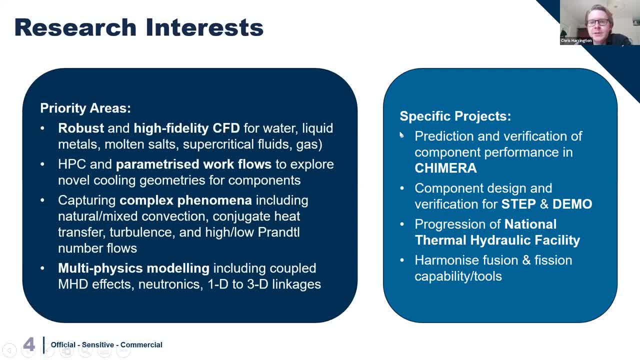 to simulate the entire plant. some particular projects lifted there, listed there on the right. so prediction and verification of components in chimera. this is the facility i'll talk to you about in just a second. it's for applying blanket type components to expected loads so that we can characterize the performance. 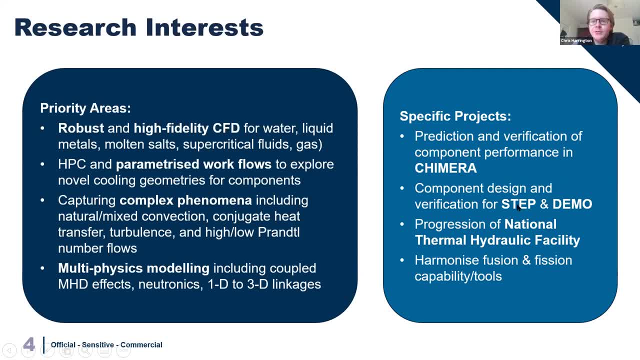 we need to be able to do component design on different fusion power station projects. so demo is the one example we looked at at the start. it's a european project. step is our own uk based project looking at a slightly different version of react, of reactor um. but again we need to do. 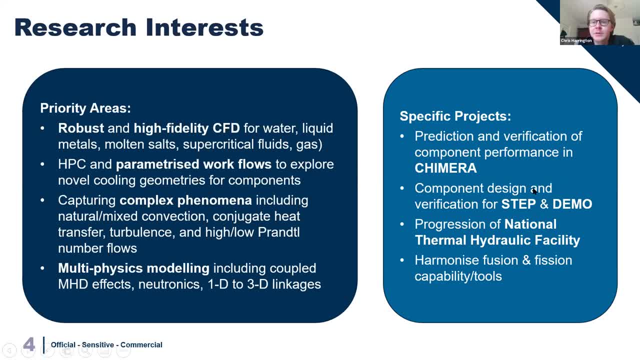 rapid design um components that we optimize for those two. in the meantime, we're also progressing the national thermal hydraulic facility, which is something we can possibly talk about a little bit later. um, that's really. we're acting as um, as overseers of a design of that project so that we can cost it up. 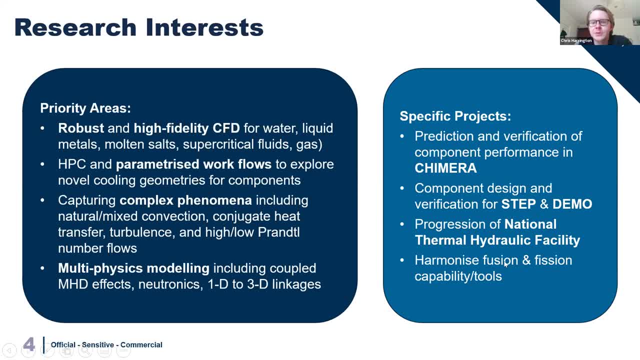 and the last point here is not particularly uh project related, but one of the main things you want to do is link all the codes that we use uh for doing a lot of this analysis for fusion uh to the same codes in fission in order to get a sort of unified capability where possible. um, so that's. 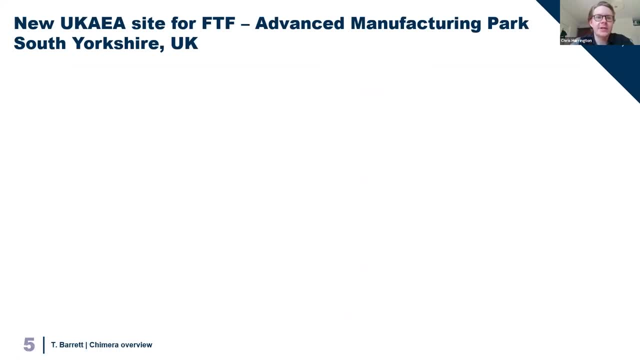 enough words on slides. um, we are opening a new center which hopefully a lot of you are aware of already in your atlas today, and you will see a lot of the information as we go along, including the Yorkshire just outside Sheffield, and this is going to house a lot of our. 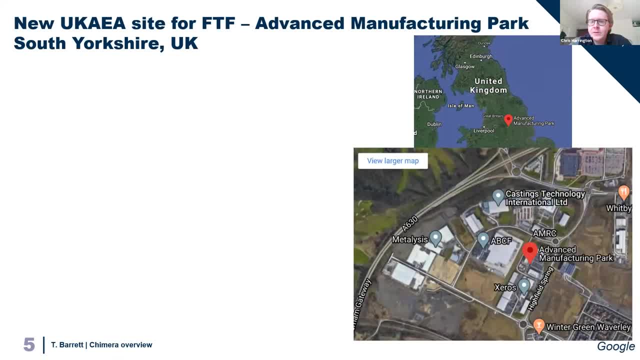 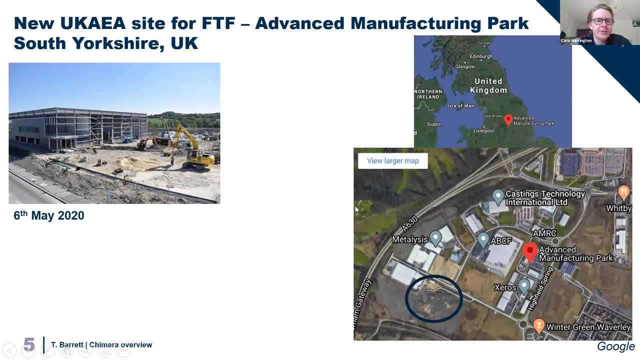 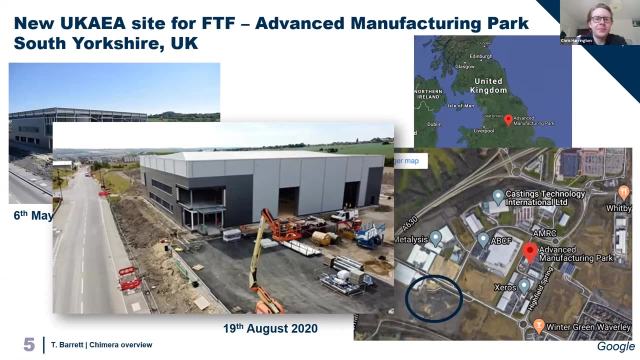 experimental capability. It's on the Advanced Manufacturing Park just between Sheffield and Yorkshire to be precise. we've got a plot of land here. The building is progressing very well. so this was earlier this year and this is it taken just a couple of weeks ago. So this facility will be open by 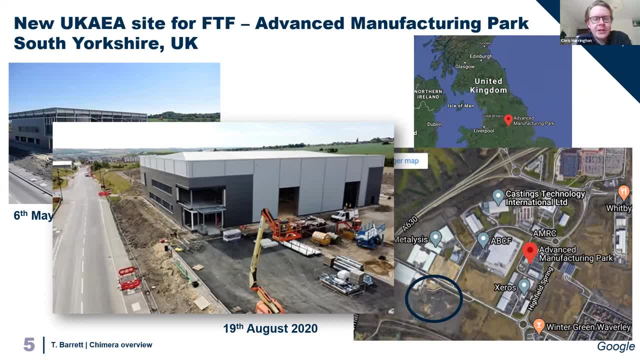 October, the main bits of kit coming in beginning of next year, The idea of this facility: we're looking to house a new thermal hydraulic group up there, and so that will bring together a lot of our capability that we have at the moment under one roof and, in particular, this building will host our Chimera. 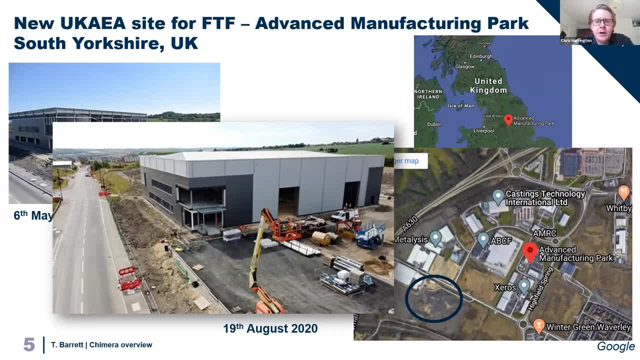 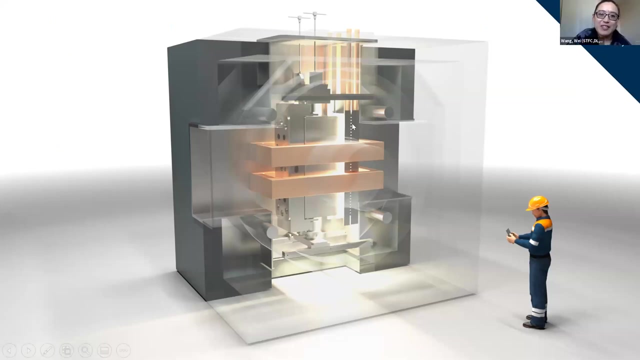 experiment which, as I say, is for applying: taking a component scale blanket module and applying heat loads, magnetic fields- to that module with instrumentation so that we can both simulate and characterize its performance and performance. So here's a quick little mock-up of how that will look. it is okay, this is my. 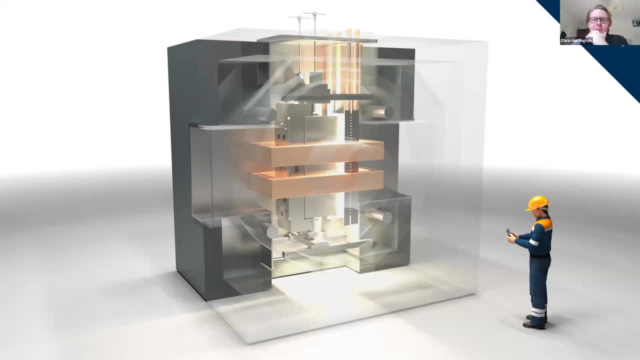 last slide, so I'll just skip through this quickly. There's a blanket module in this central position and around that there are magnets supplying high magnetic fields and there's cooling coming in at the top and there's a heat load being applied to the front of this, and so these are all magnets and a 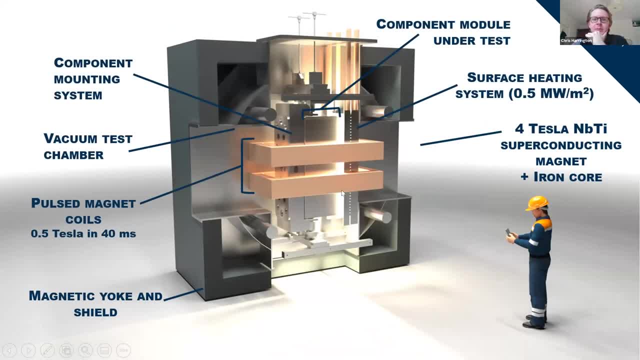 vacuum vessel that houses it. It's about a meter in scale. so this is a serious piece of engineering: High heat loads, high magnetic fields, high pressure water, high temperatures- that we'll be able to simulate in this facility, and we're looking for ways to characterize that flow and validate it as well. 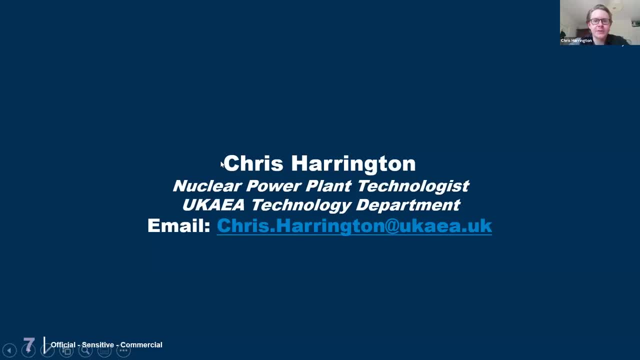 So that's quite an exciting time, and I'll just leave a virtual business guard there on the screen. if there are any questions, just feel free to email me. Okay, yeah, thank you, Chris. The next one is from a man from Eheimenダイエモン・カレー・キリシー・. 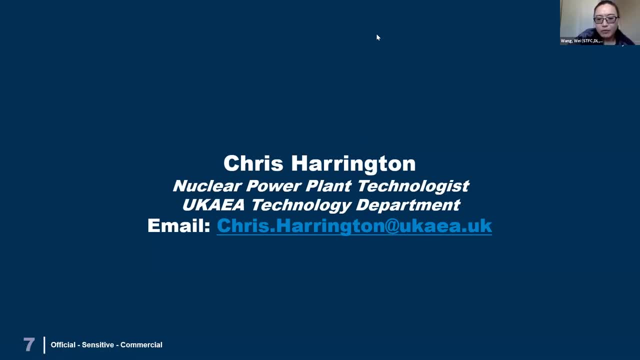 Iheimenダイエモン・カレー・キリシー・. Thank you, Chris. The next one is from a man from Eheimenダイエモン・カレー・キリシー・. 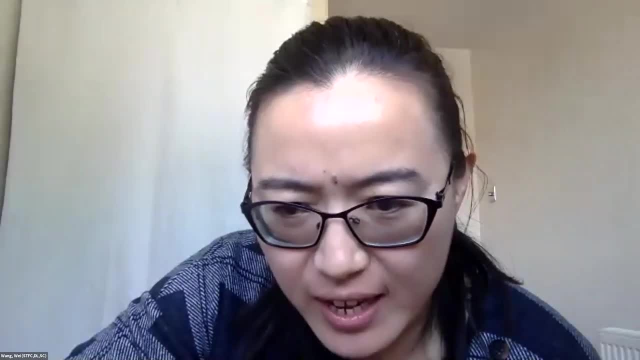 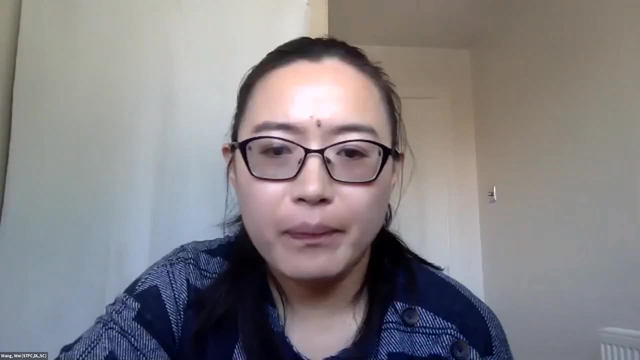 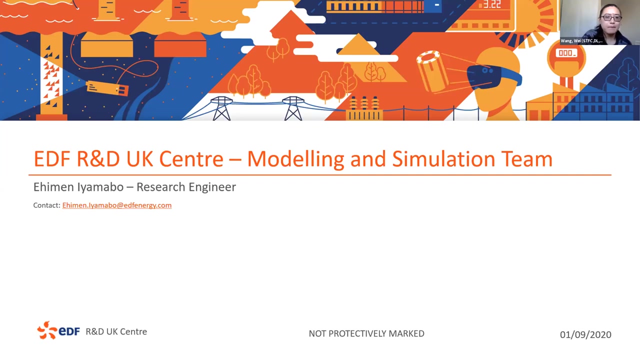 Thank you, Chris. The next one is from a man from Eheimenダイエモン・カレー・キリシー・ Iron Marble or EDF Energy R&D UK Centre. Hello everyone, good afternoon. can you see my screen very well? 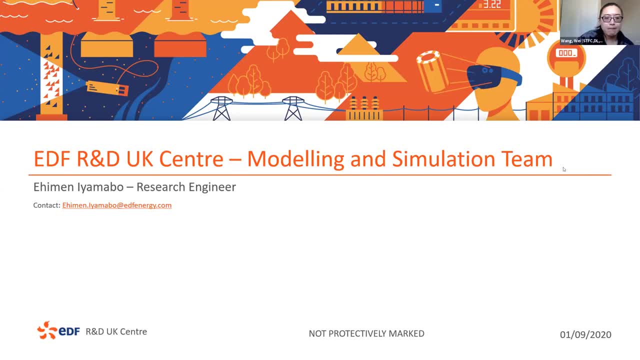 Yes, Okay, My name is Ehime Yamabo of EDF R&D UK Centre And I'm also a concluding PhD student at the University of Manchester. I'm going to give a brief overview of what we do at the Modern Energy Research Centre. 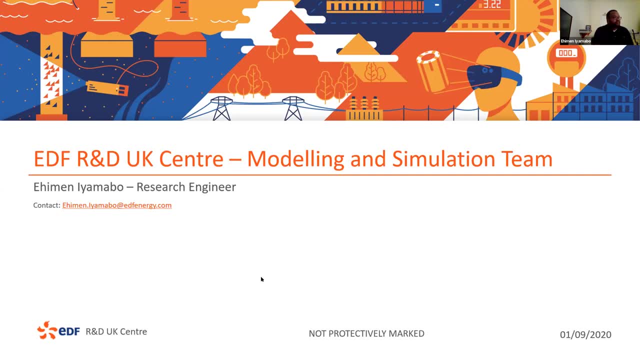 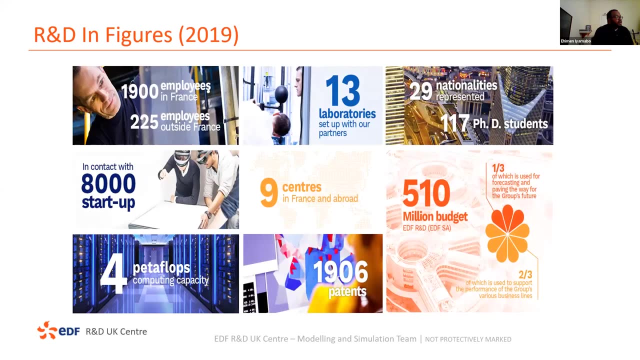 at the University of Manchester. So our rating figures: we have about close to 2000 employees in France and about 325 employees also in France. 13 elaborated. We have labs and set up all over the world with about 2,000 nationalities represented. 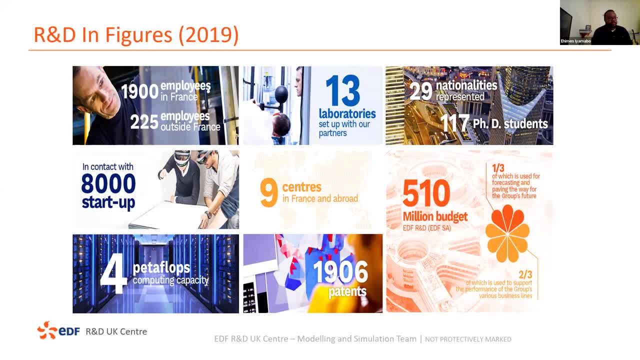 and 117 PhD students either have been funded or supported by us, And currently we have a budget of about €510 million, with about two thirds going to supporting the business activities or the group and one third for forecasting or paving new technologies or new systems in our group. 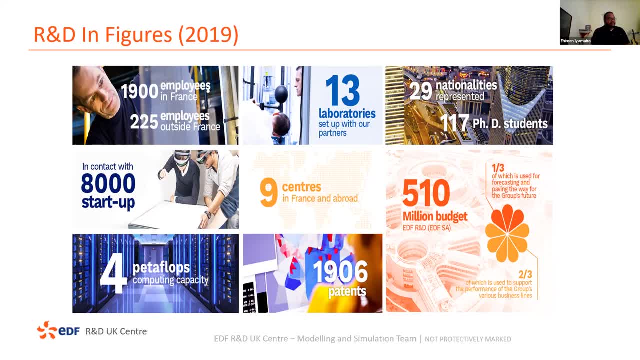 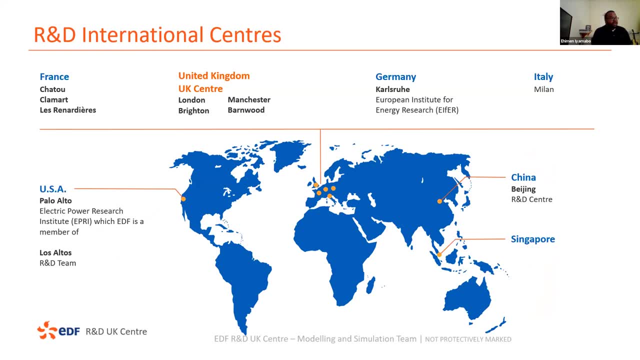 We have a very good super computing facility. We have about with a capacity of about four petaflops. So the R&D group has centres all over the world. We are scattered in France, Germany, Italy, United Kingdom. In United Kingdom we have centres in London, Brighton and Ballard. 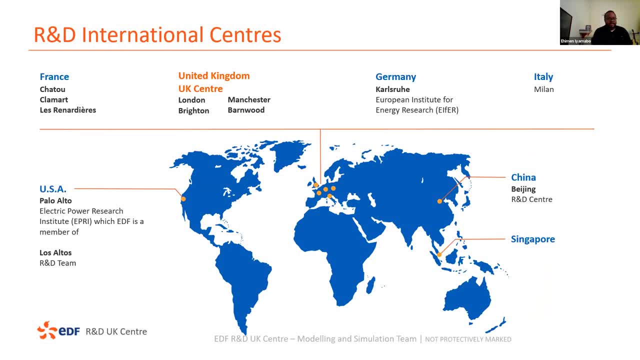 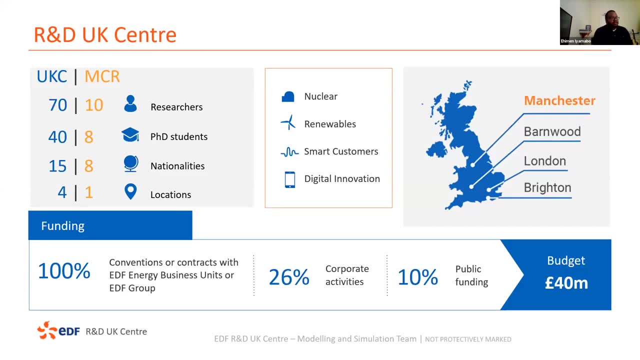 And, as I've already mentioned, the Centre, Modern Energy Research Centre, which is embedded in the University of Manchester, And so this is an overview of the R&D group And so this is an overview of the R&D staff in UK Centre in the UK. 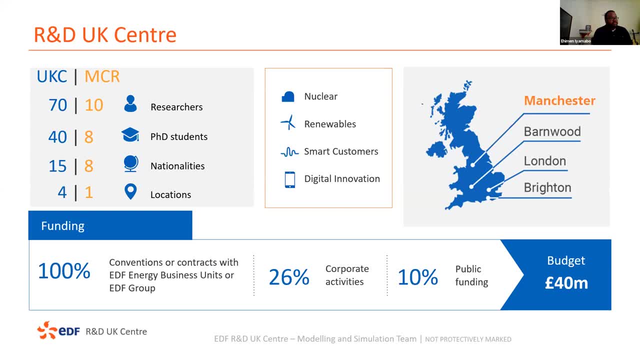 So overall, there are about 70 full-time researchers, with 10 based in Manchester. We support 40 PhD students overall, with 8 based in Manchester, And we are quite diverse, with about 59 nationalities. 100% of our funding is from conventional contracts with the EDF business units, of which we have. 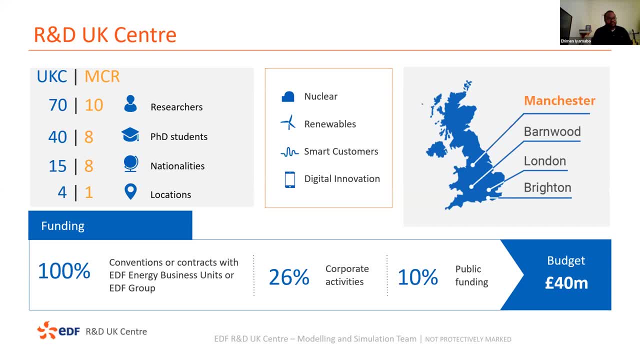 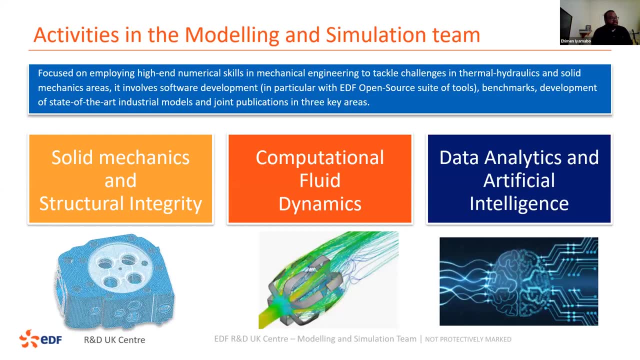 26% comes from corporate activities and 10% from public funding. So activities in the modeling and simulation team. So we are in the Modeling and Simulation Centre at the University of Manchester. We are focused on developing high-end numerical skills in mechanical, structural and nuclear engineering. 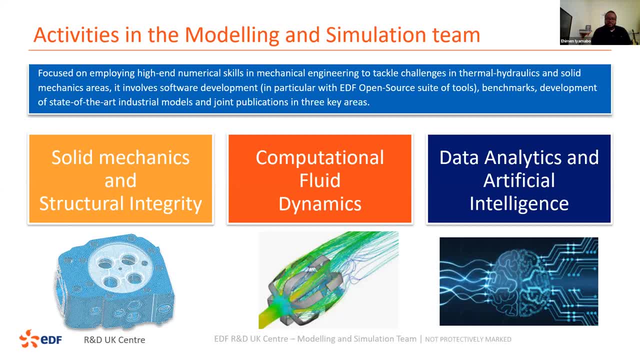 We tackle numerous challenges in thermal, hydraulic and solar mechanics stress in the nuclear industry. It involves a lot of software development, of which I'm sure you're aware of, the numerous sets that we have, the numerous open source codes that we have at EDF. 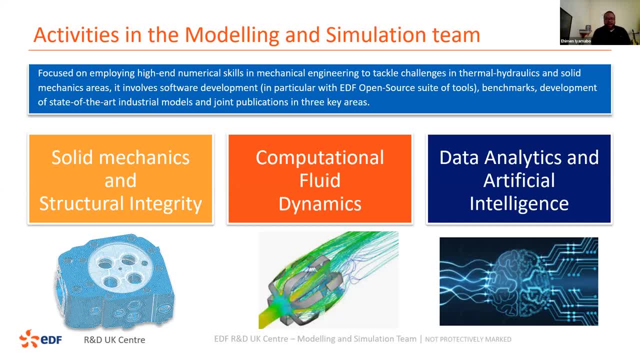 Benchmarking and the development of state-of-the-art industrial models and publications in three key areas, which are solar mechanics, structural integrity, computational fluid dynamics, and now we are increasing activities in data analytics and artificial intelligence. Thank you, Thank you, Thank you. 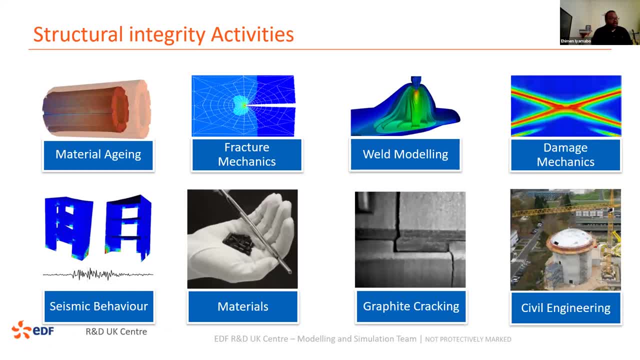 So in structural integrity activities we have our research focuses a lot on the following things on the screen, which is the study of material aging of our AGRs, structural mechanics and wall model and model of which we have strong collaboration with at the University. 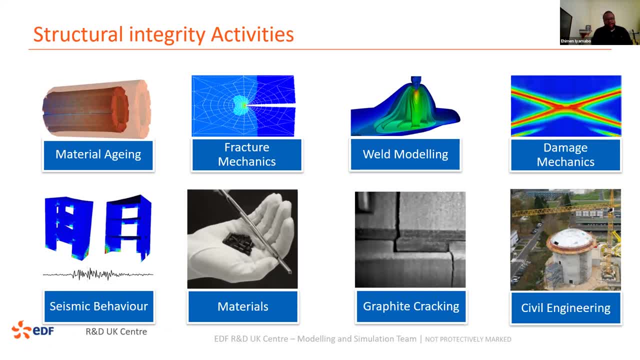 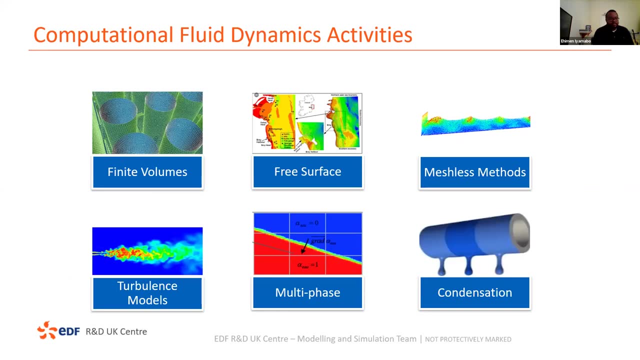 of Manchester and damage mechanics and seismic behavior, materials and graphite cracking, and also we do have activities in civil engineering. In computational fluid dynamics. we focus a lot on final volumes of which we have developed in a number of states, particularly with Saturn and other open source codes. 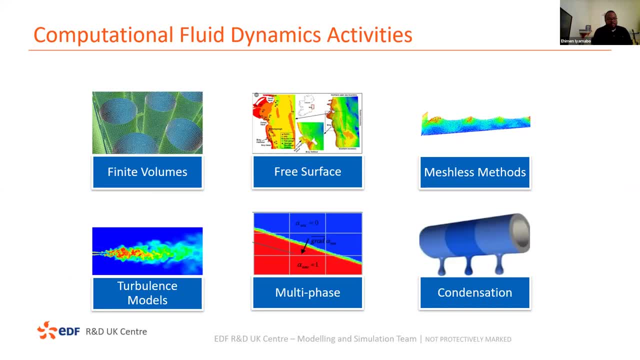 We have research in free surface. Currently we are expanding our research in measureless methods, which is quite relevant to us, particularly with SPH At the Model and Simulation Centre. we have developed a lot of advanced stimulus models, particularly in RANS and recently in hybrid RANS-LS methods. 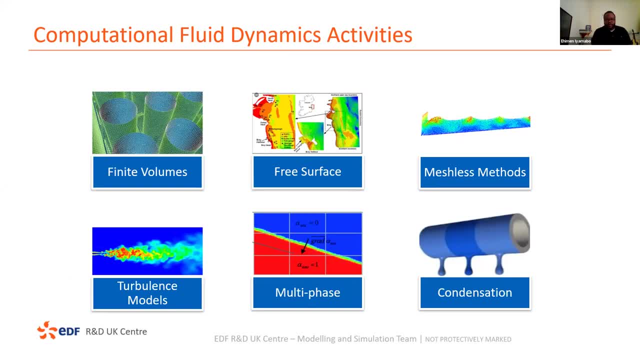 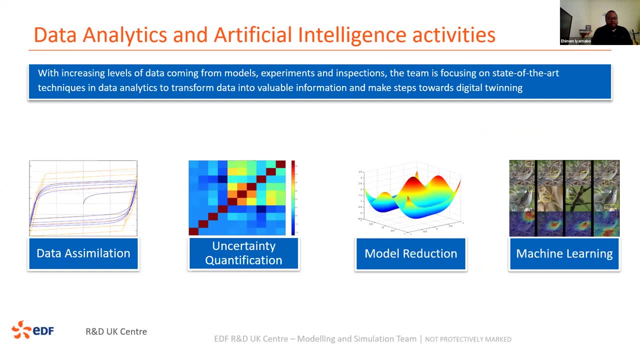 Thank you. And now we're also moving. we also have research into multi-phase and conversion activities, So recently so our research activities in Boydsea, at the Instructional site that generate a lot of data, a lot of data from our models, experimented on different investigations. 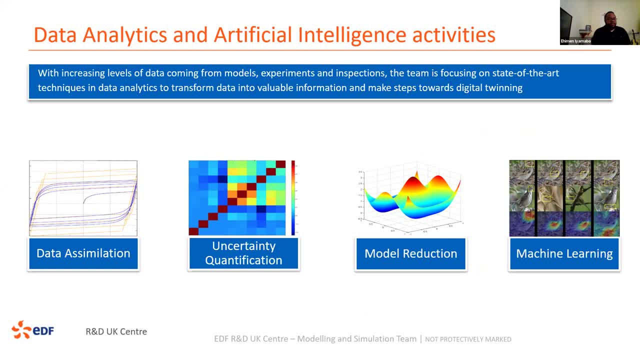 and now? the team is now focusing on developing, say, the art, techniques and analyzing this data and transform this data into more volume information to enable us to make more effective decisions in the future. and our data analytics involves data simulation and uncertainty classification and model reduction and machine learning. So the Model and Simulation Centre and 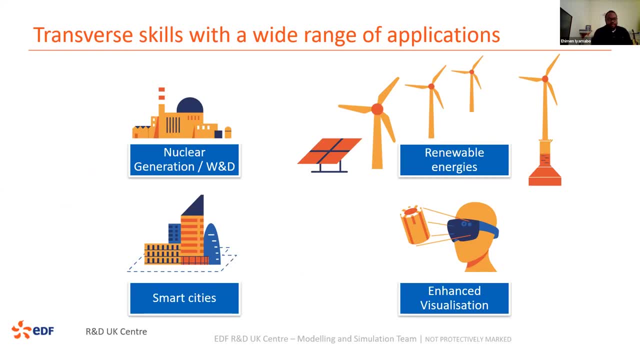 the R&D Group in the UK has a lot of engineers with various skill sets, which is used to support a wide range of activities in nuclear generation and waste and decommissioning, in developing technologies and renewable energies, and also developing solutions or innovative innovations in smart cities and enhanced visualization. 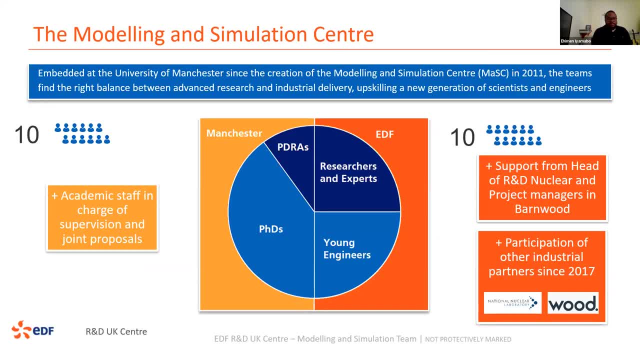 So I'll move on to our partnership. So our Model and Simulation Centre is split into two sides. We have the University of Manchester side and the EDF side. The University of Manchester side is supported by the experts or the staff members from the academic team at the University of Manchester. 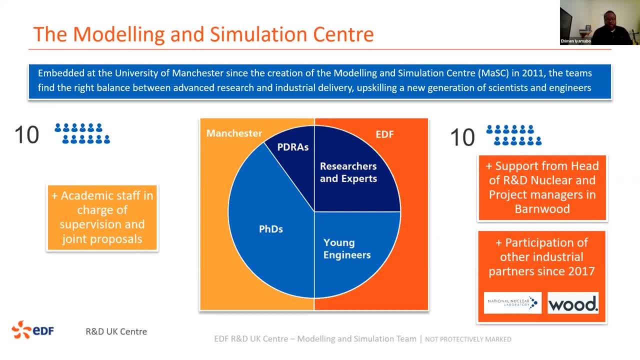 who are in charge of the supervision and supervision for PhD research and also proposals. And in the EDF side we have about 10 staff of researchers and experts and we support also a lot of interns and young engineers and we develop them, we upskill them. 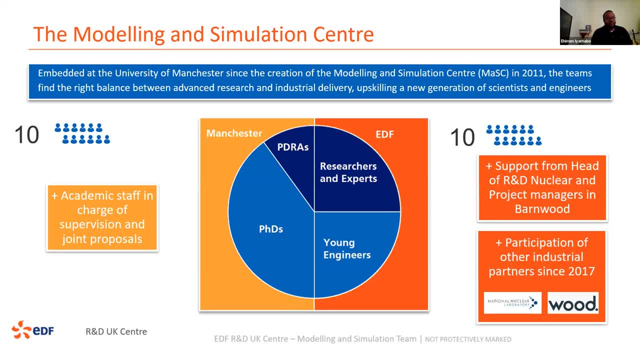 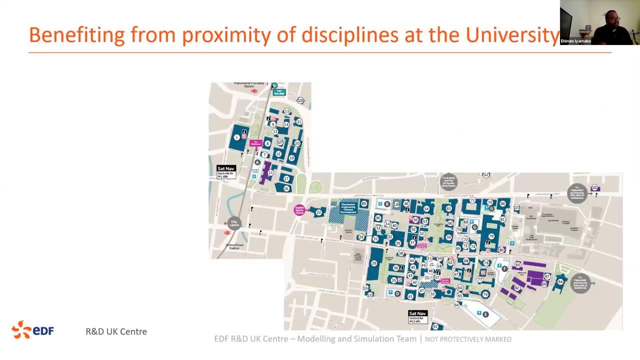 So we're active in the development of new generation of scientists and engineers and with Manchester and EDF, we find the right balance between advanced research and also industrial delivery. Also, we also collaborate with a number of industrial partners, including NNL and Wood. As earlier I mentioned, we are based in Manchester, which enables us to basically pick up a number. 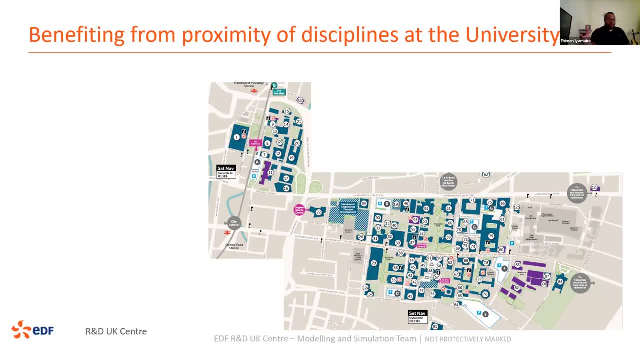 which enables us to pick up a number of or enjoy being close to a lot of actions in research in different departments, in the Model and Simulation Centre which is in Joshua, which is the home of the Model and Simulation Centre, in the Parsevita which I think. your time runs out. 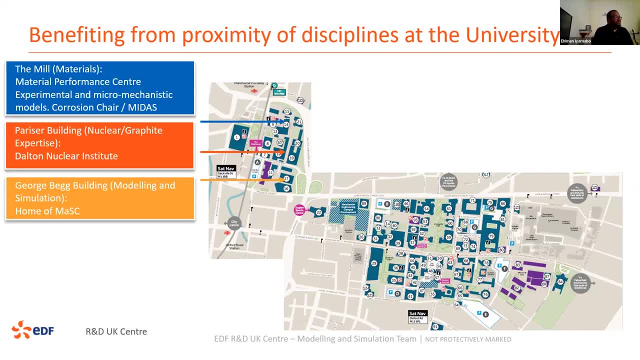 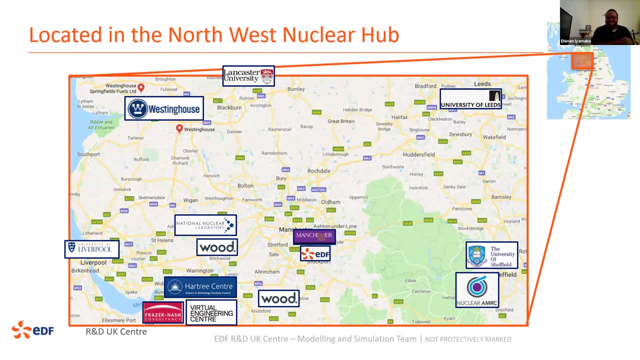 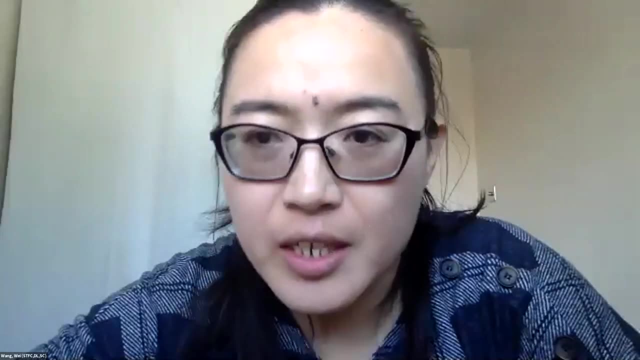 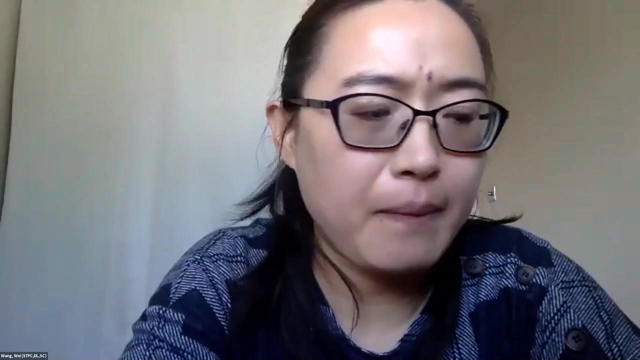 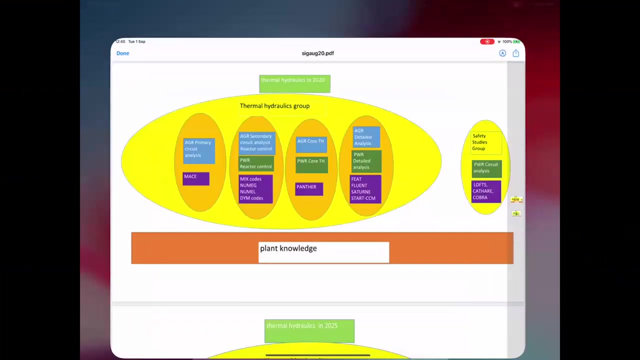 Oh, okay, all right, okay, I'll just end here, and I think this is my last slide, so thank you very much. Thank you, thank you very much. Our next talk is from MacRabbit, EDF Energy Engineering. Hello all, so I work for EDF. can you hear me? 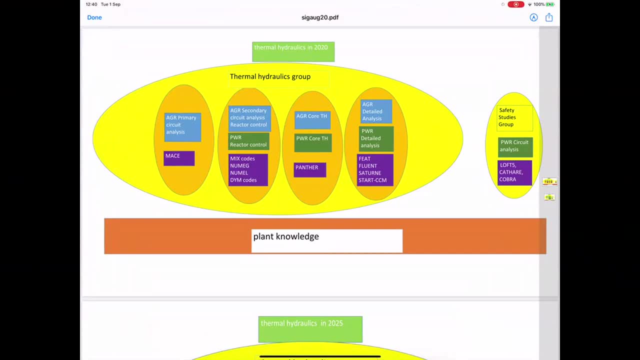 Yes, You're good. So I work for EDF. we operate the commercial nuclear reactors in the UK, So we have 14 gas-cooled reactors and one pressurized water reactor. That won't be the case for too much longer. The two reactors at Hunterston will stop operating. 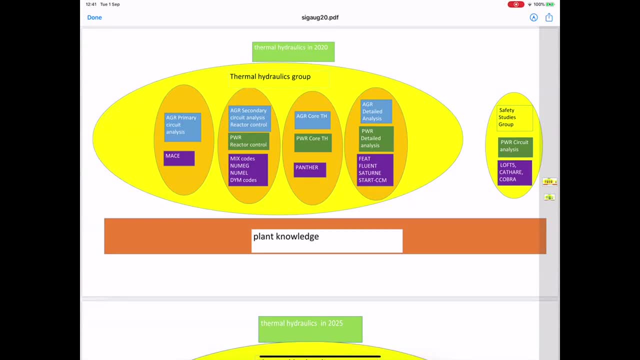 early in 2022, which is just over one year from now, and they are stopping due to the challenge of making a safety case from cracks in the graphite core, Our two newest gas-cooled reactors, which started operating in the late 80s, so that shows you how long ago it was. they'll be closed. 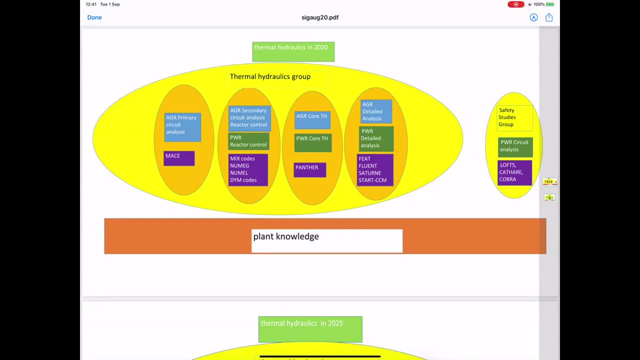 in 2030, so that's two years from now. So we're going to be working on that 10 years from now. So in 2030 we won't have any more gas-cooled reactors operating. We are currently building a new pressurized water reactor at Hinkley Point C. 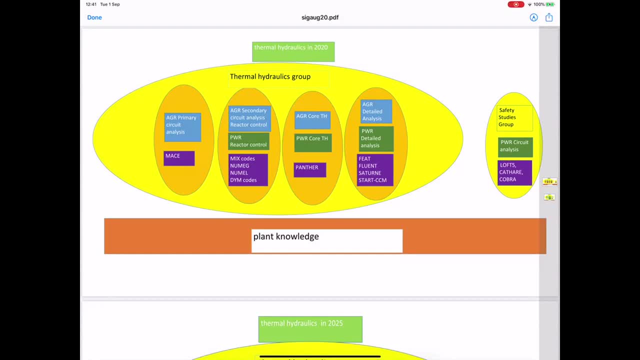 and that will start operating in 2025.. So the ratio of gas-cooled reactors to pressurized water reactors at the moment- now we're considering that Hinkley is an operating reactor- is 14 out of 16.. So most of our thermal hydraulics support is done on the gas-cooled 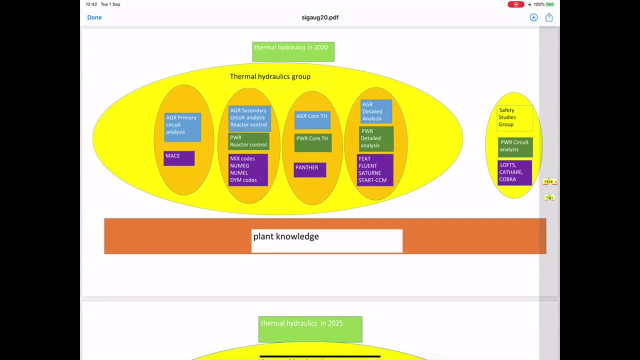 reactors. So in the period of time between now and 2030, we've got to move from supporting a fleet of ostensibly gas-cooled reactors to a fleet of pressurized water reactors, and we're hoping to build another PWR down in Sizewell as well at some point in the future. 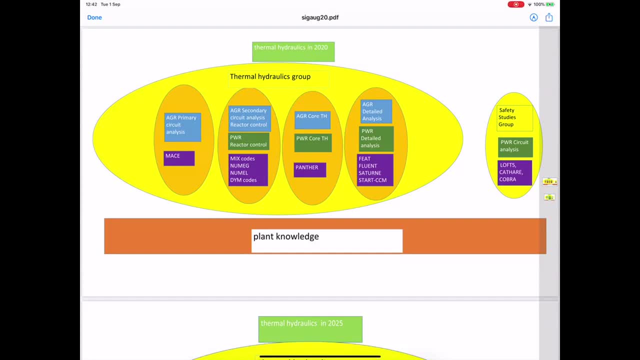 So I'm showing you a slide here of where we are at the moment. so thermal hydraulics in 2020.. So we have a thermal hydraulics group and we support the operation of our nuclear reactors in four main areas. So we have a team which looks at primary circuit analysis, which looks at what happens in 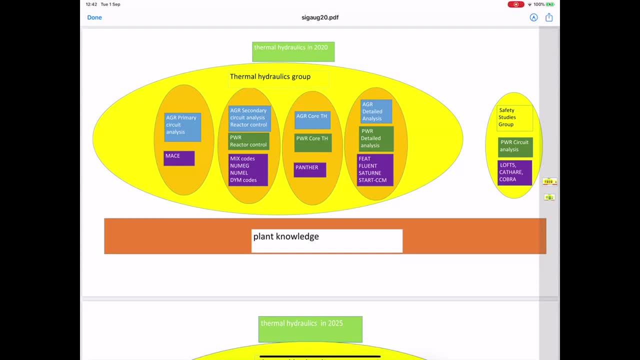 the primary circuit, ostensibly during normal operation, steady state and also postulated faults. That uses a network flow solver called MACE. The next team looks at management of boilers, and they're him and the previous presenter is working on building a CFD model of a boiler. 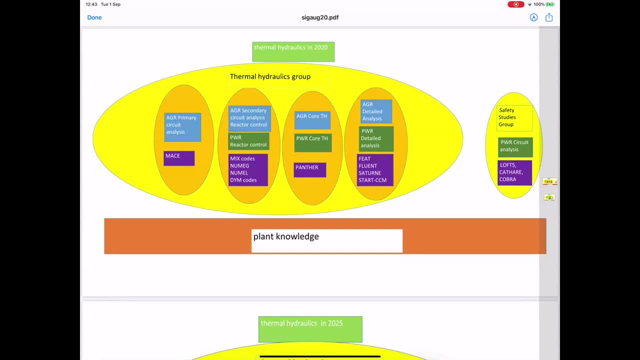 by the way. But this team looks at managing boiler tube temperatures to make sure that we can operate to the end of the life that we'd like them to operate to. We also do things like thermodynamic cycles to make sure we can get the most of our reactors into the Rainbow, and that's. 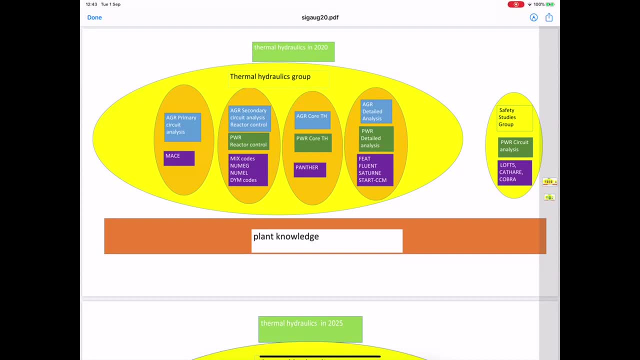 the goal for us. We also do things like dynamic cycles to make sure we can get most of our reactors, reactors, reactor control, so they they use codes which are again of the network flow type of technology. the third team is a core thermal hydraulics, pwr core therm hydraulics, which 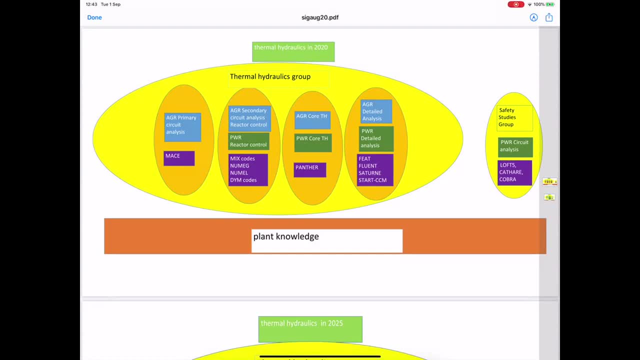 looks at the thermal hydraulics in the core, and our fourth team, which is what i'm part of, looks at detailed analysis. so quite often we'd like to know quite detailed temperature distributions and we would use cfd, for example, to to do that for us. so in in the thermal hydraulics group at 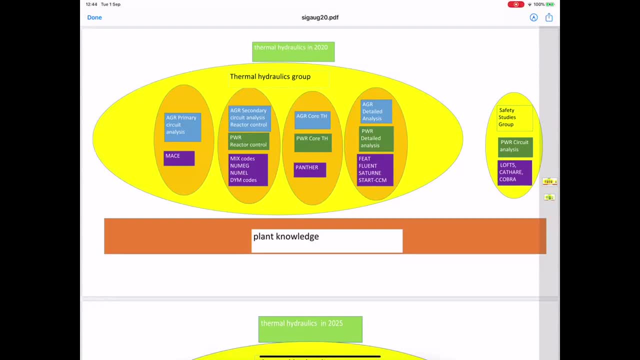 the moment we've got 14 people working as well as that and we have another group of thermal hydrolysis working in safety studies group which is essentially looking at what goes on in a pwr. i think there's maybe five people looking at that. so that's what's going on in at the moment and in 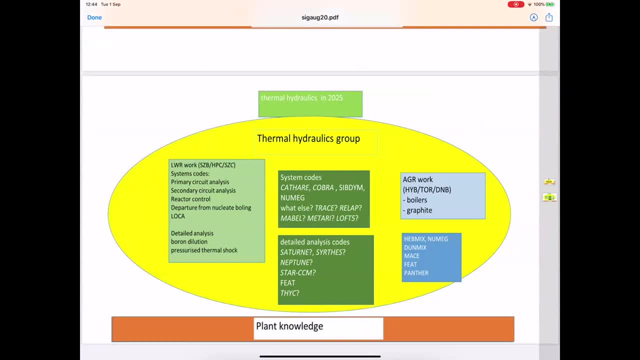 2025, which is just five years time. we're going to have to do a lot of work on that. we're going to have to move to much more support of the, the pwr stations. we're going to have to carry on supporting the agrs, but we're going to have to learn how to support the pwrs. so 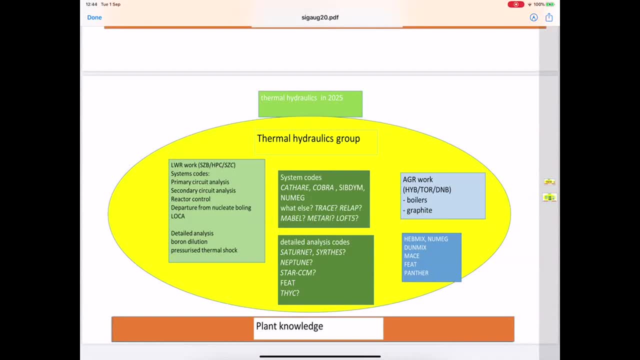 we haven't yet decided precisely which tools we're going to be using, but that's why some of them are in question marks, and there's certainly some things which aren't even mentioned on that slide. so we are trying to define what problems we're going to be having to solve and 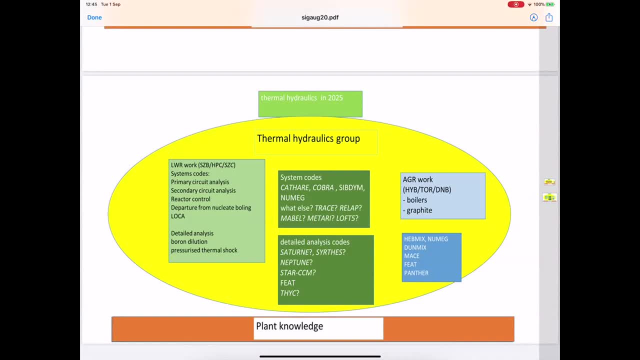 then define which tools we're going to have to solve, as well as carrying on supporting the agrs, and the agrs are those sort of stations where we get a lot of work from, and that will definitely continue. so the problem we have is to train our existing thermal hydraulics community. 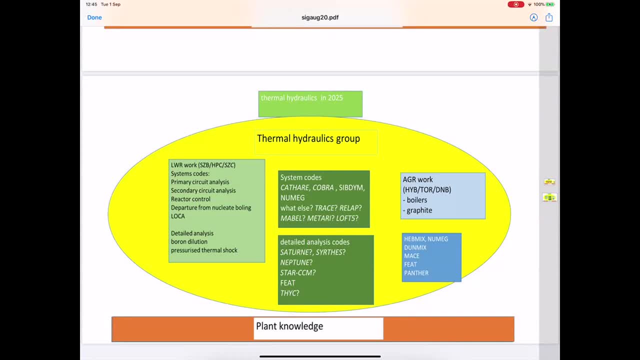 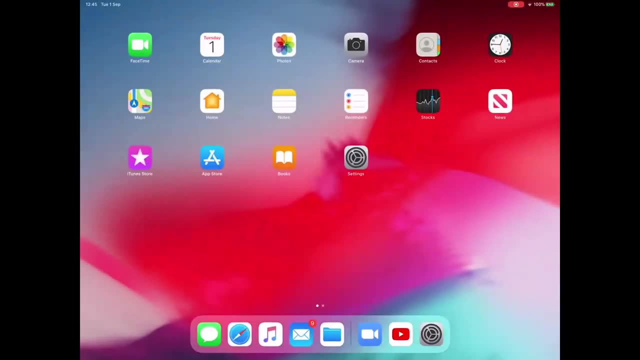 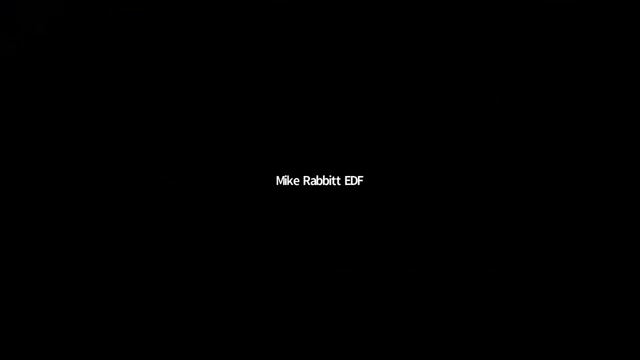 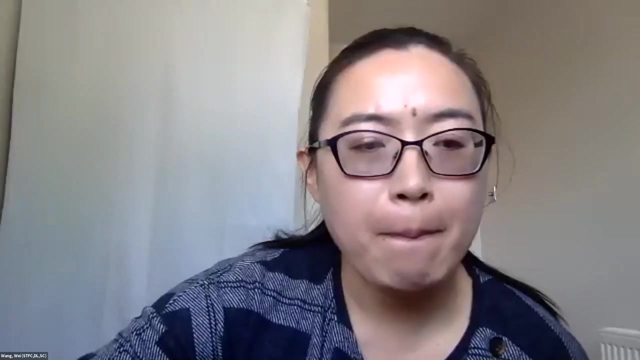 in the tools we will be using in five years time, and i think that will. that will do for today, thank you. thank you, mate. our next one is from ryan thompson ross royce. hi everyone. so unfortunately it's not been possible for us to share any slides, so i thought 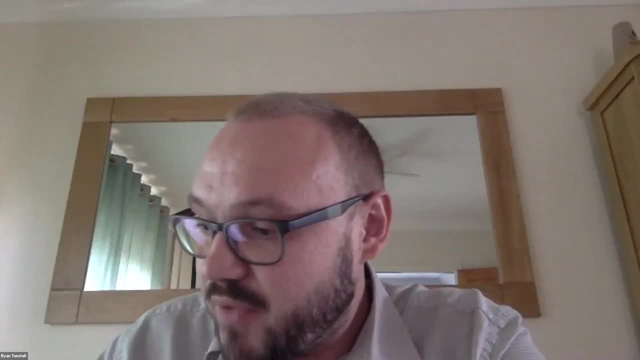 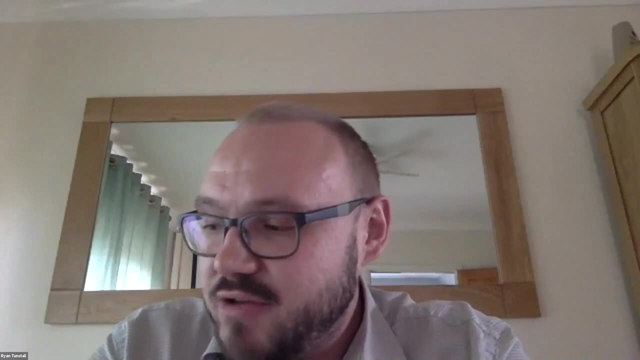 i'd just spend a few minutes sort of saying what our interests in this are. so i'm the section lead at rolls royce for computational fluid dynamics. we've got a broad interest in sort of the wider computational thermal hydraulics discipline. um so we use thermal hydraulics discipline and we've got a broad interest in the wider computational 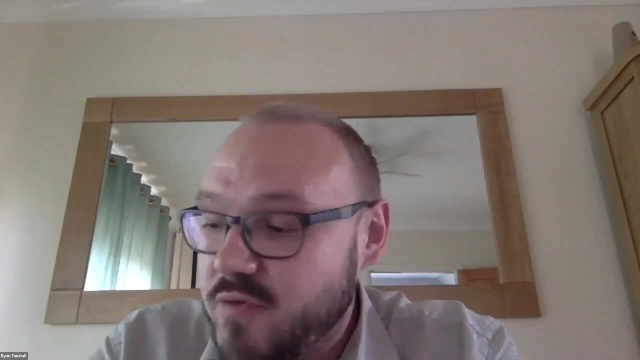 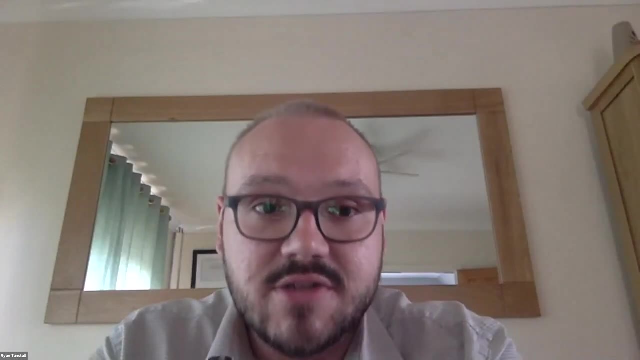 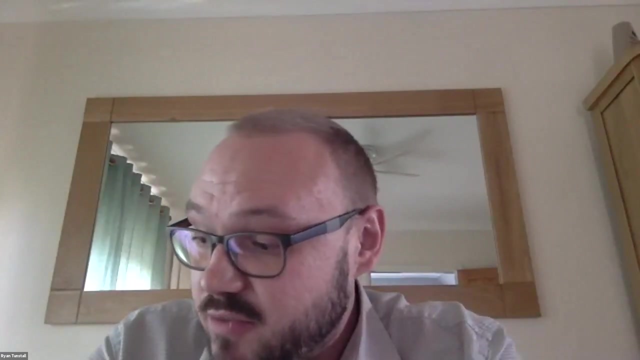 fluid dynamics discipline and we've got a broad interest in the wider computational. we also make quite extensive use of systems code for plant performance analysis- um as mentioned by hector and mike previously, and we've got university technology centers at the university of manchester, imperial college, london, um. so typically we're using cfd to model flows within components. 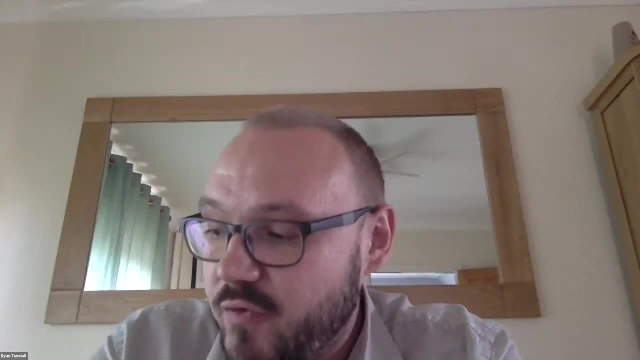 and subsystems um primarily using rams analysis. quite often with transient boundary conditions that can be a challenge um. we also do some limited um les analysis for high cycle thermal loading and we also do some limited um les analysis for high cycle thermal loading. and and pretty much all of our cfd analysis now is in siemens star ccm plus. 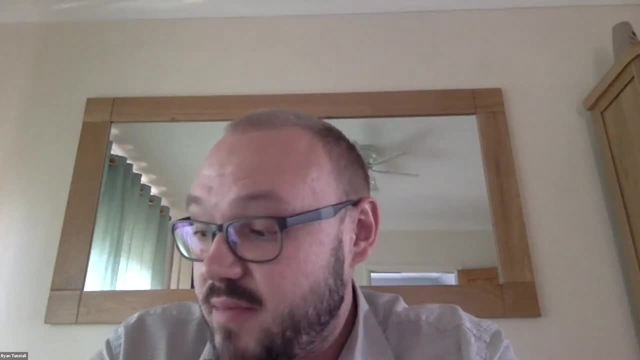 so from the ccp on a cfd front, i think what we're really interested in is improved vmv standardized qa processes, as well as sort of benchmarking, perhaps using high fidelity les dns, solutions to sort of benchmark rams and the like that we use more regularly in industry. 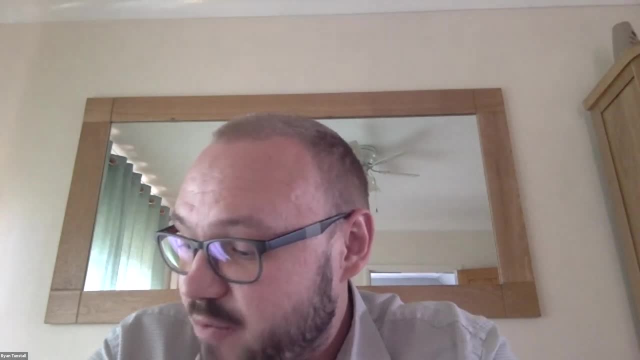 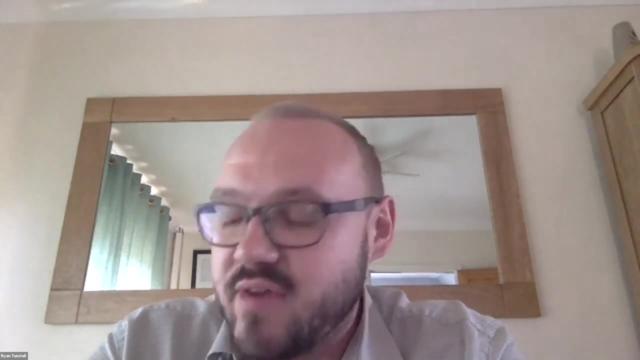 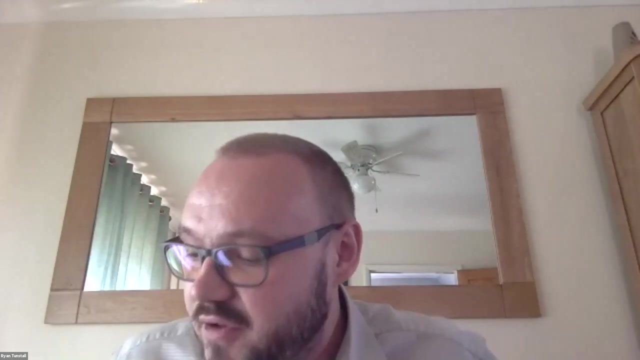 um. one of our main challenges as well that we're interested in how we could try and address partly through this ccp, is sort of improved acceptance and wider acceptance of the use of cfd and safety justifications, and we're also interested in improved cfd modeling for 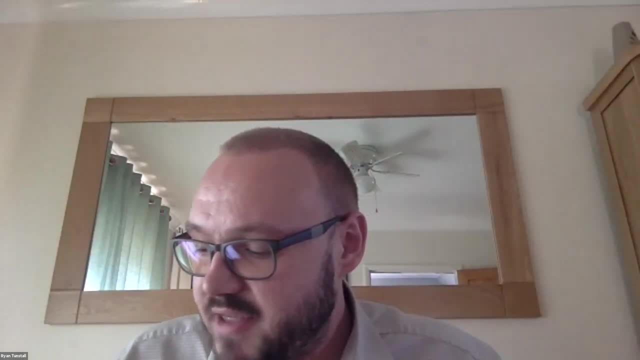 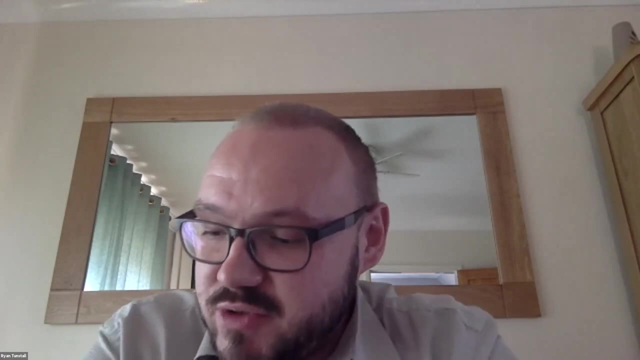 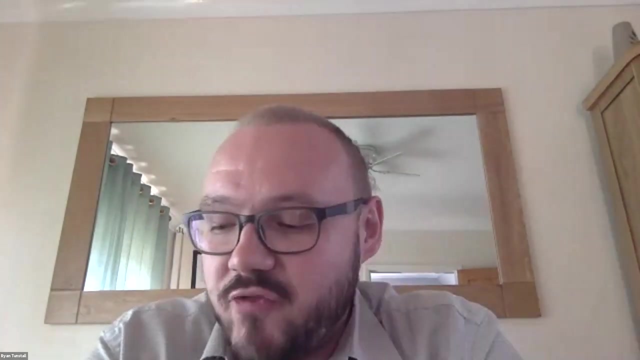 scenarios like nc and boiling, particularly at the macroscopic scale. um, as i sort of mentioned as well, we've made quite extensive use of systems codes for plant performance analysis, but we also know that they've got their own limitations. yes, they're fast to run. you can run them for many, many different scenarios and iterations, and we're also interested in how we 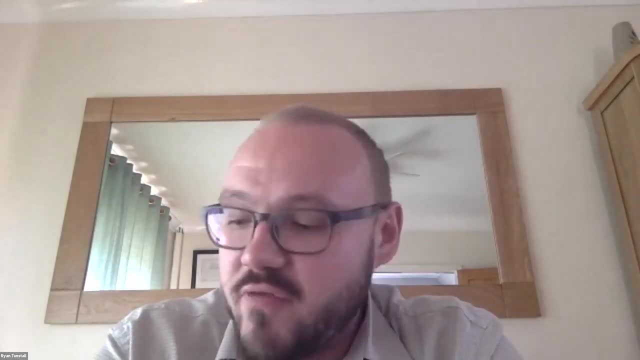 can run them for different types of applications, but in some circumstances their assumptions break down. they're not very accurate. on the other hand, we've got cfd, but it's much more expensive. it's more accurate, but you can't often run it at sort of the whole system level. so something else that 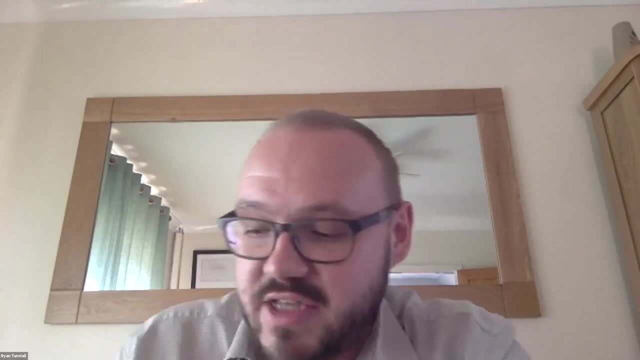 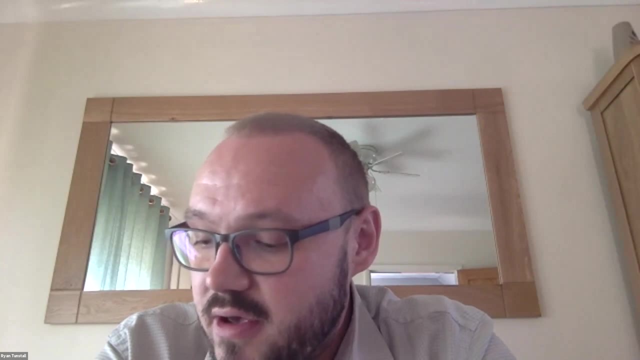 we're really interested in is bridging that gap between systems, codes and cfd. maybe it's, course, cfd of a wider system, maybe it's code coupling, maybe it's reduced order models. so that's something else that we're interested in, particularly for things like natural circulation. 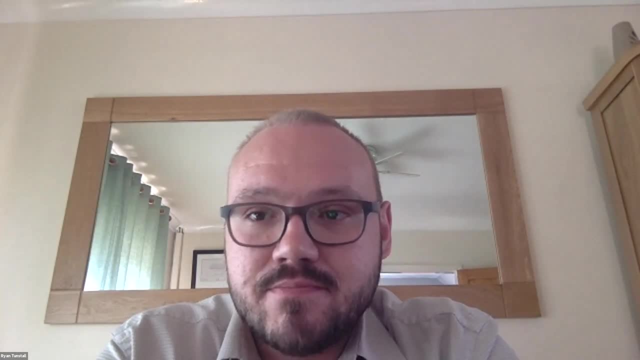 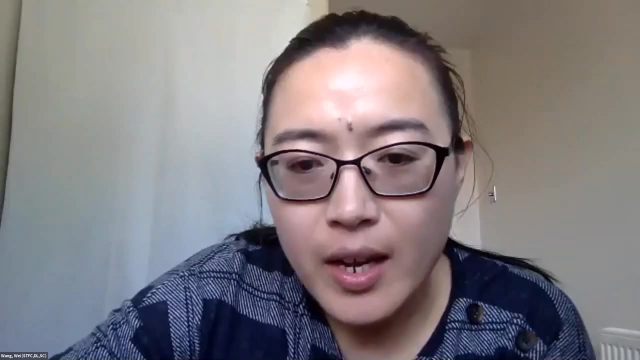 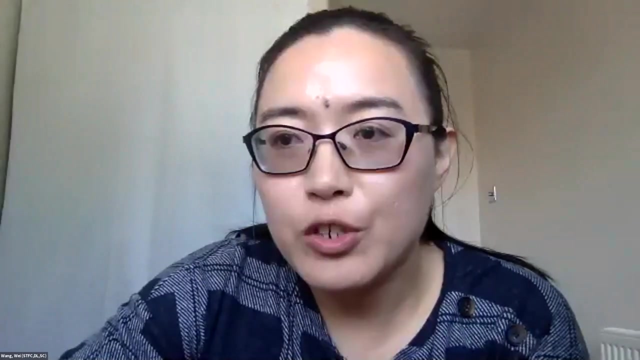 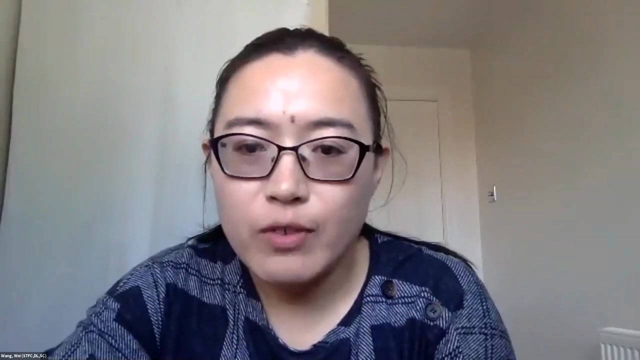 so that's something else that i've got to say. really okay, thank you, ryan. um, the next one is supposed to be adam owen, uh, from molten more text energy. but uh, he mentioned he will share a pre-recorded video, but until now, unfortunately we haven't got got a video from him. so we go to our last talk in this section. 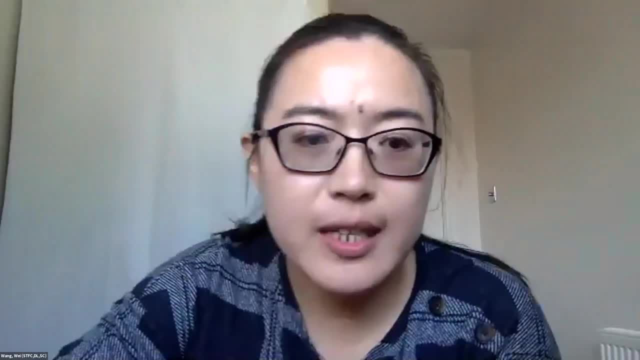 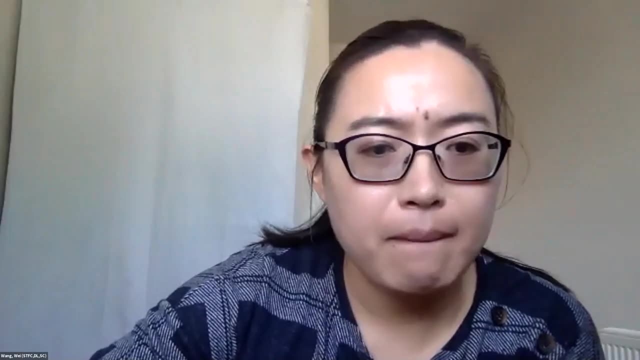 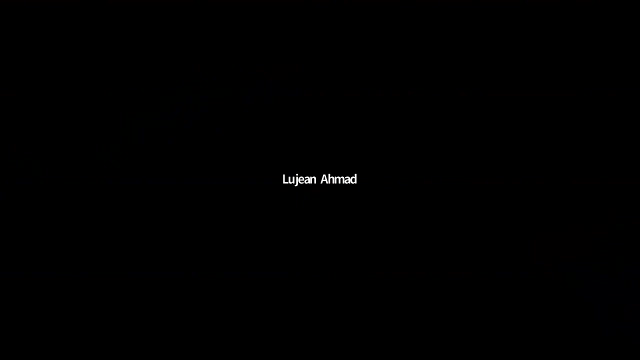 from what we've been talking about in the last part of the presentation, and then we're going to go to our last talk in this section. from what we've been talking about in the last part of the presentation: usan, brunel university. hello, hello, um, unfortunately, professor hassan johara has had to leave. uh, we've got another. 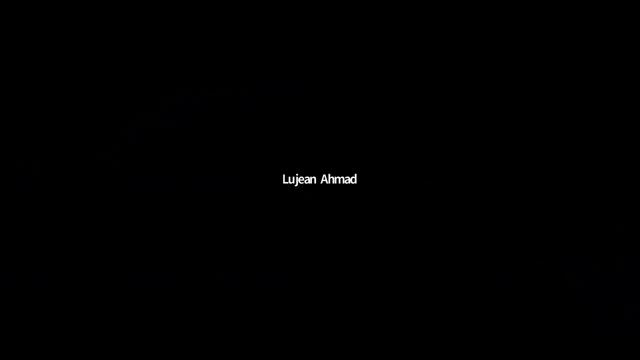 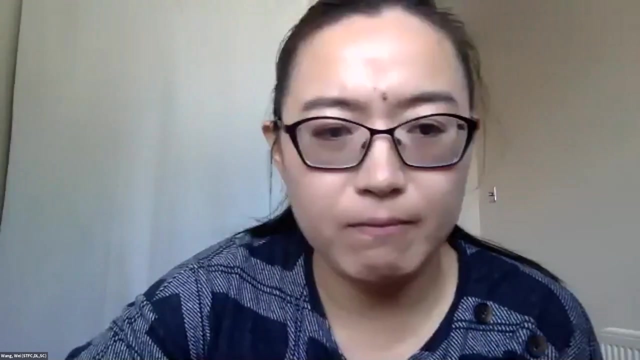 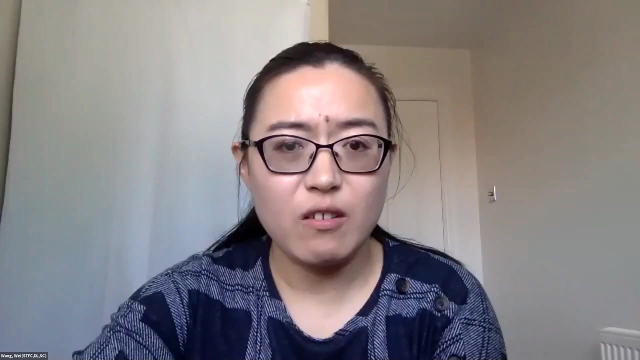 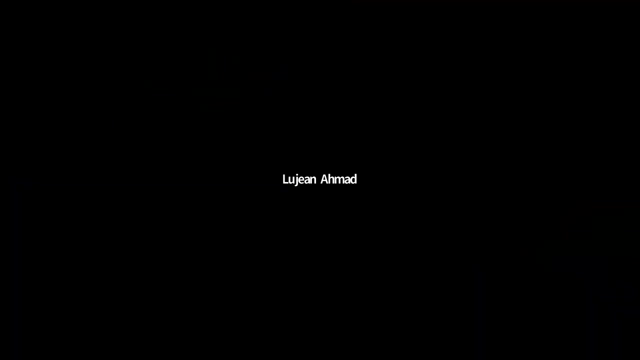 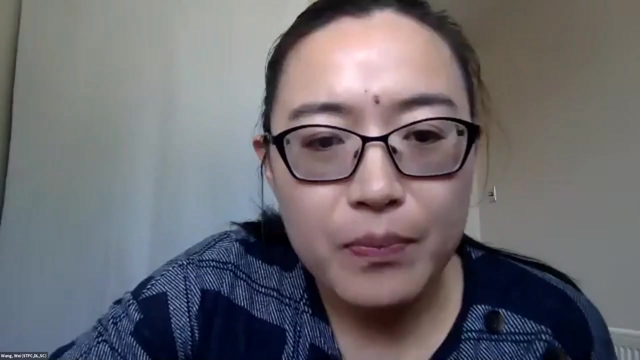 meeting, but we are happy to share the slides, uh, with yourselves afterwards, okay, thank you. thank you, can you share your slides? or? yeah, of course we can share them via email to the whole group while you're doing all the sharing. absolutely no problem, okay, thank you. we go to the end of this section and we hand over to hector for the discussion. 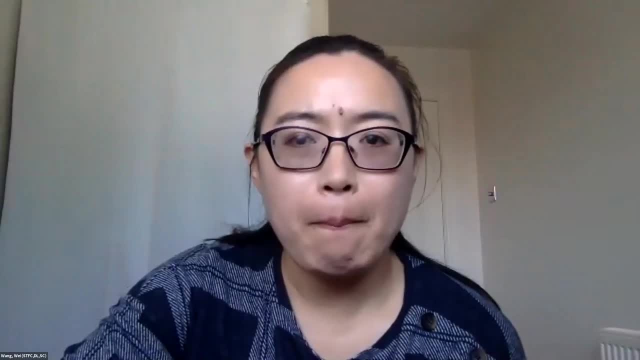 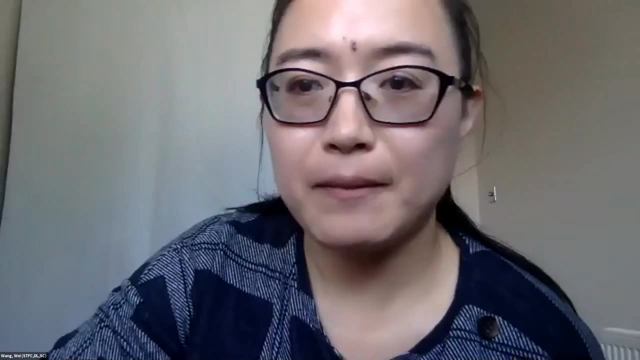 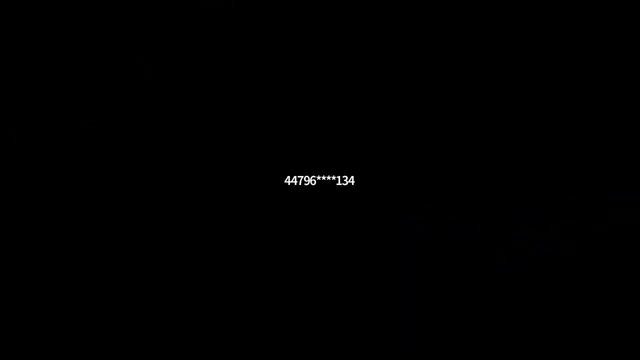 section hector. hello, hi, can you hear me? yes, it's a hector. yeah, well, my, my internet went down halfway through these presentations and i have a few questions. um, you know, in this health, I just managed to get back in using my phone, So I'm a bit out of touch with what happened in between. 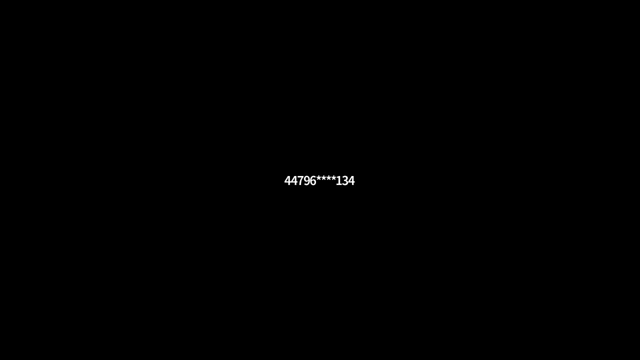 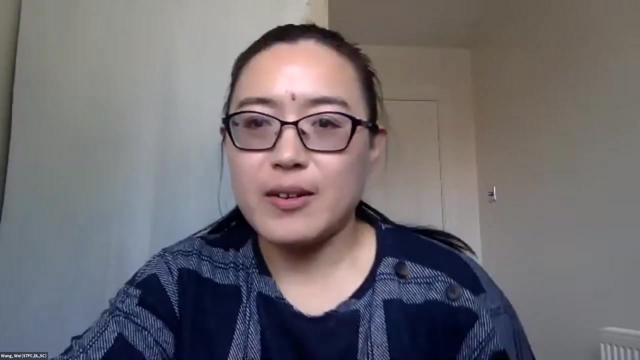 Have we just finished the presentations? Yeah, we just finished the presentation. Okay, Yeah, we have some-. It would be difficult for me to facilitate the meeting because I don't have any visual. I only have my phone. Okay, I think, Professor-. 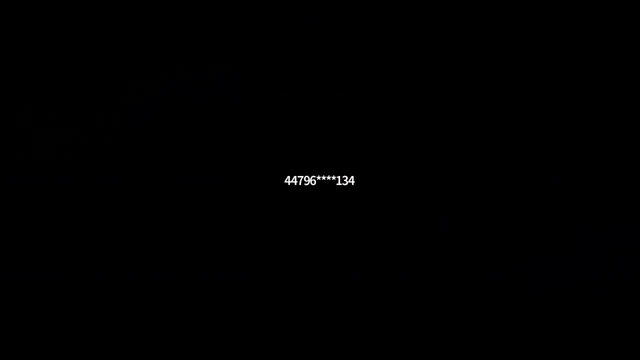 For the moment, yeah, For the moment. my network has gone down and trying to reboot the router several times, but that doesn't come up, So I just thought I couldn't even send you an email, So I can only follow through my phone. 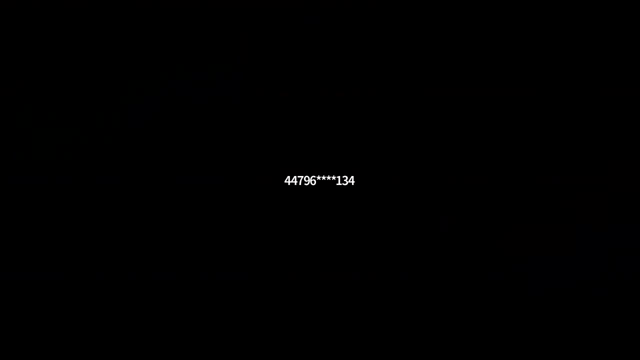 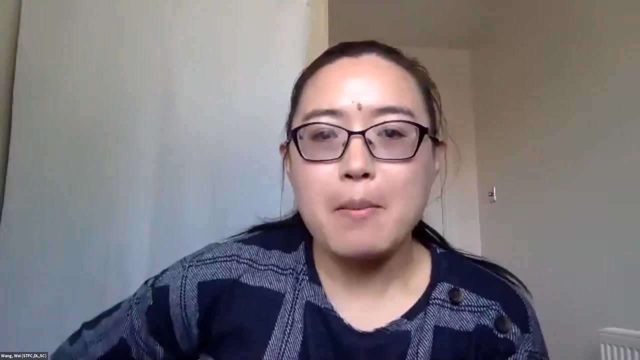 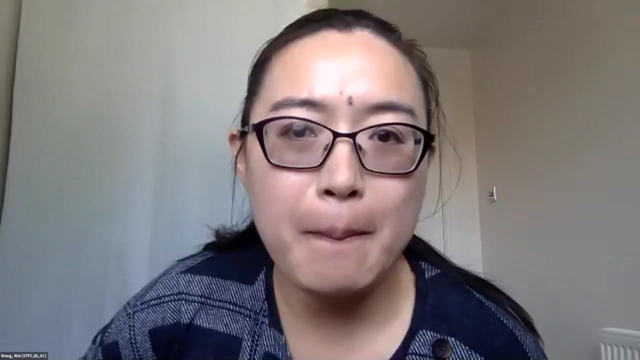 but I cannot. actually, it wouldn't be very easy for me to facilitate the meeting Because I can't see any screens or anything. Okay, yeah, Professor Shui-Hsuan. hey, are you here? Is that okay for you to facilitate the discussion? 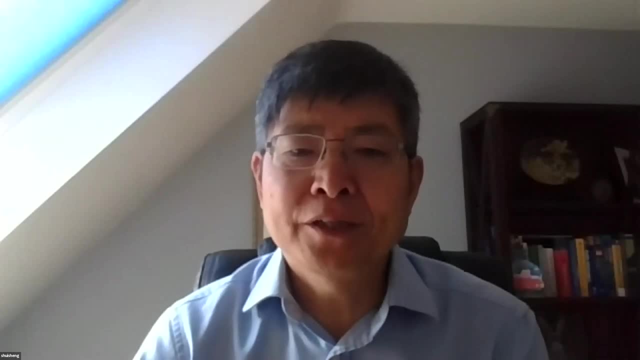 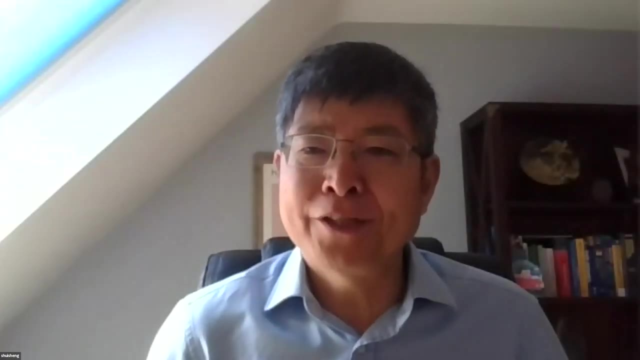 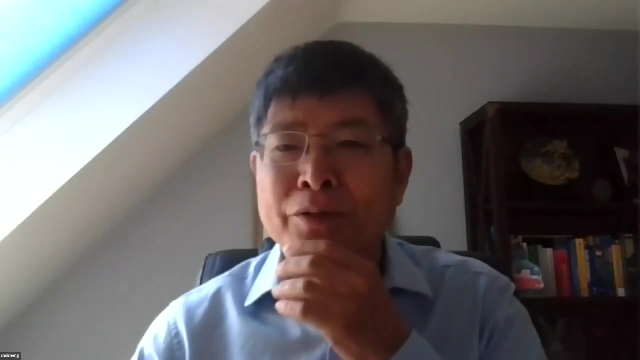 Oh hi, We have. can you share the list of the questions please? Sure, Right, Okay, thank you very much for your presentation. I'm sure it's very difficult to actually limit the presentation to five minutes. I found that was difficult, but thank you very much. 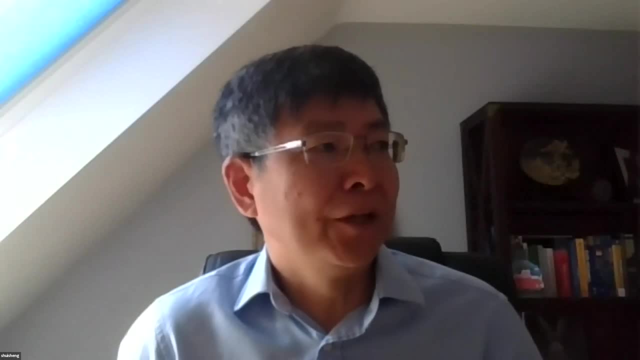 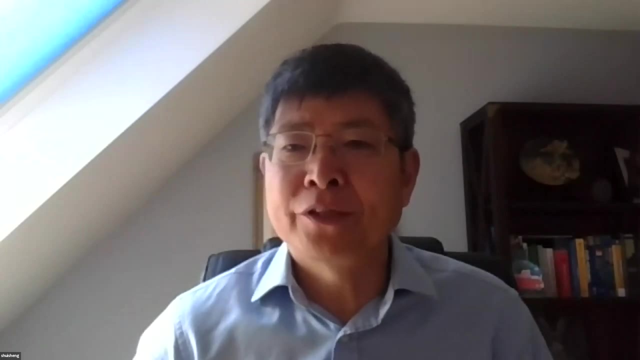 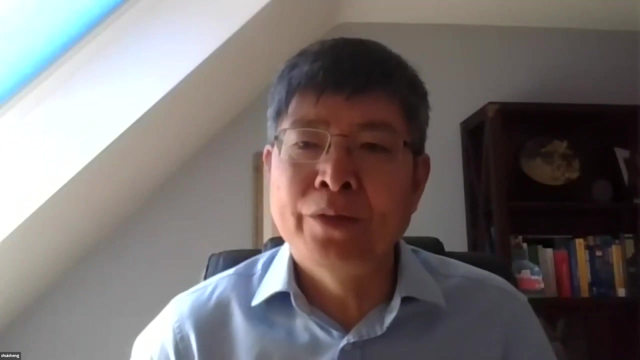 And we're all very useful And let's try to finish the discussion session relatively quickly, but it's important still. We actually have, like we have, feedback and comments from the general community And in the past this is a hugely important part. 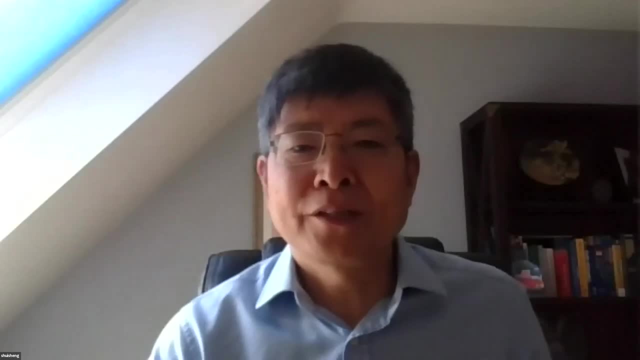 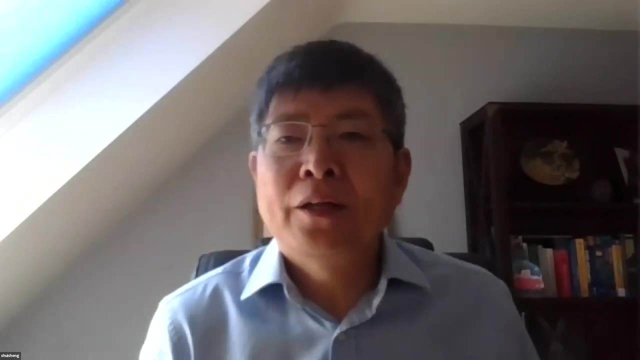 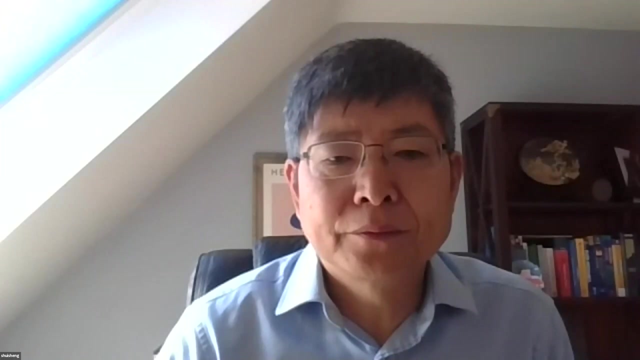 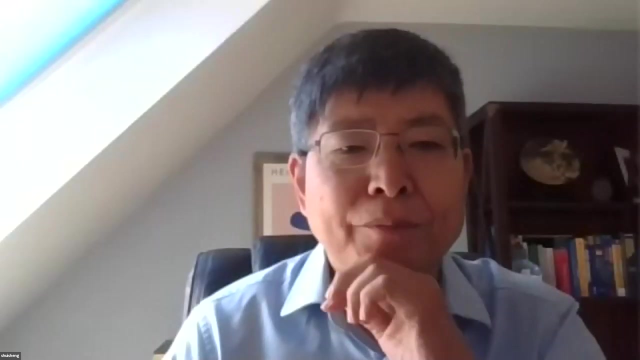 but this time we have to limit this whole thing. But wait, are you going to share your screen about questions? I'll send you an email about the questions. Okay, Okay, It's in my email, is that? Hmm, Okay. 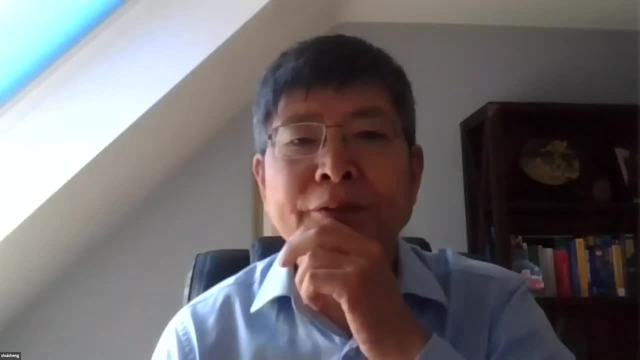 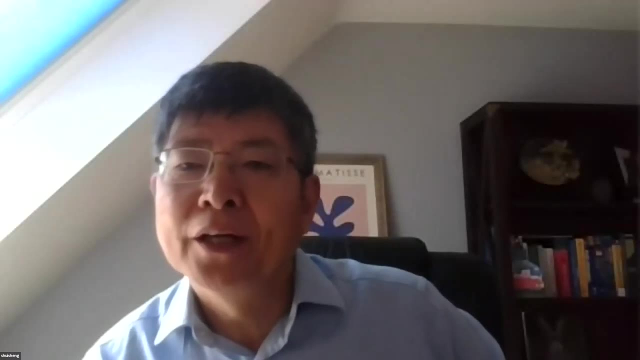 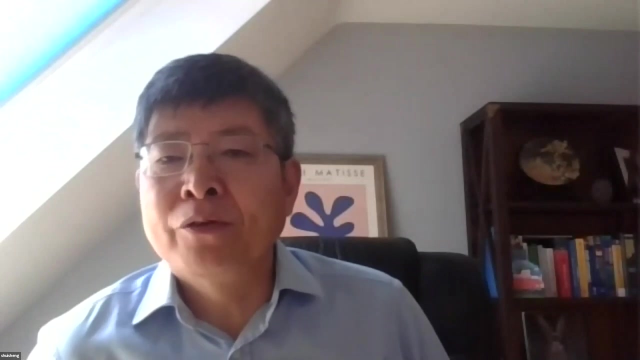 Yeah, I put the questions in the chat. Yeah, Okay, that's good, Right, Yeah, probably still useful for way to share. but for now you can see there are five general questions. Those are just questions for people to think about. 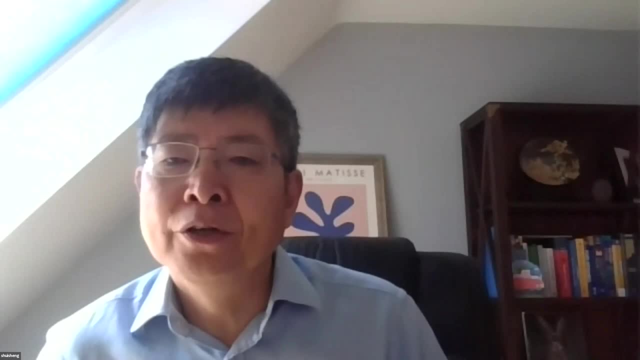 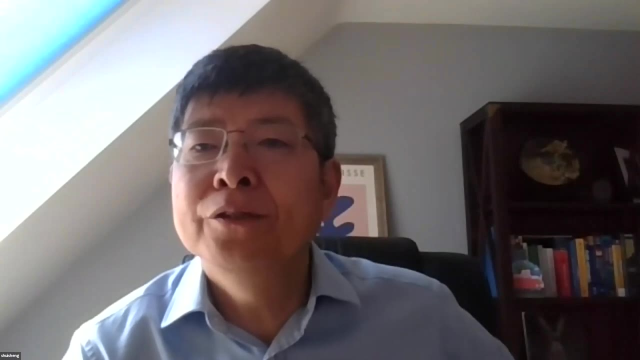 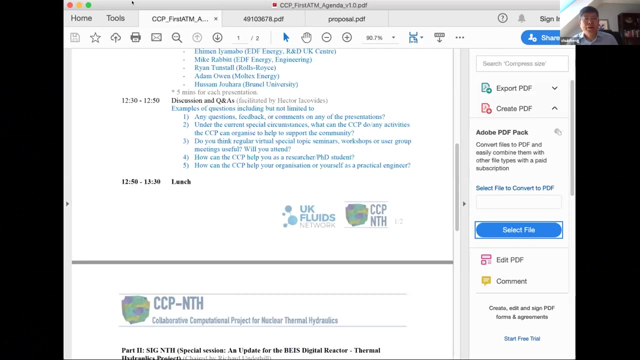 but your questions do not have to limit to any of these. So I wonder whether you know if you have any questions. I wonder whether anyone want to start any questions. It could be general questions about the CCP or any questions to one of the presenters. 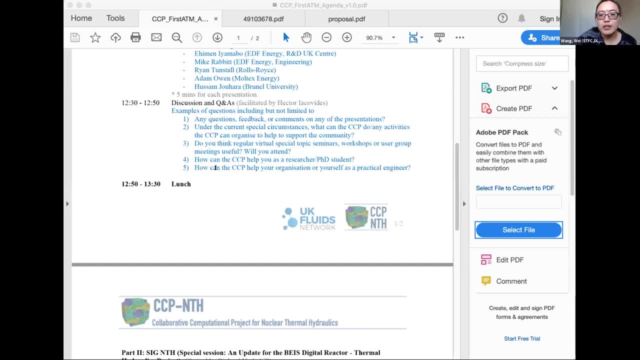 So starting- I think we can start from the questions in the chat. Yeah, we've seen your question way here already, So we've seen say. number one is general questions, feedback, comments on any of the presentations. Number two is under the current special circumstances. 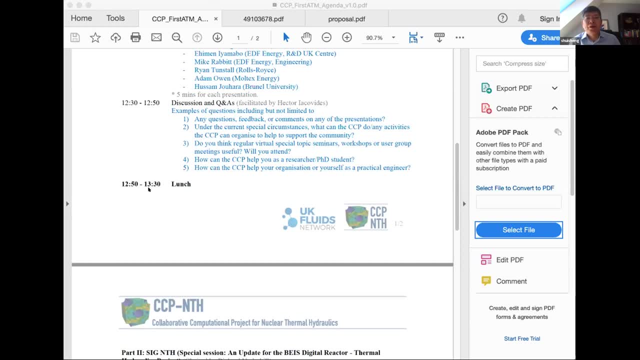 what can the CFD do and any activities the CFD can organize to help to support the community? And number three is: do you think regular virtual special-topic seminars, workshops, user group meetings useful when you attend? Then number four is: how can the CCP help you? 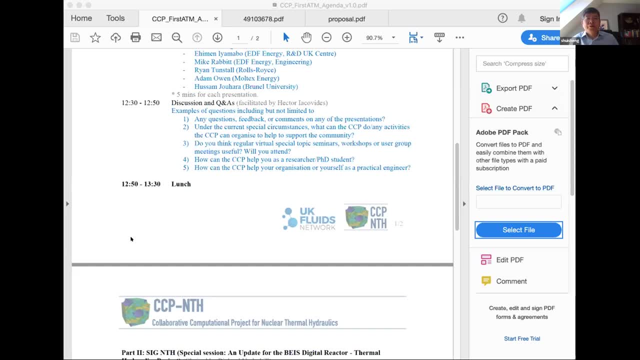 as a researcher or CFD student? Or, lastly, how can the CCP help your organization or yourself as a practical engineer? Why the- Sorry, Yeah. so eventually I have a question for the CCP project. It seems we kind of going to do a lot of benchmark work. 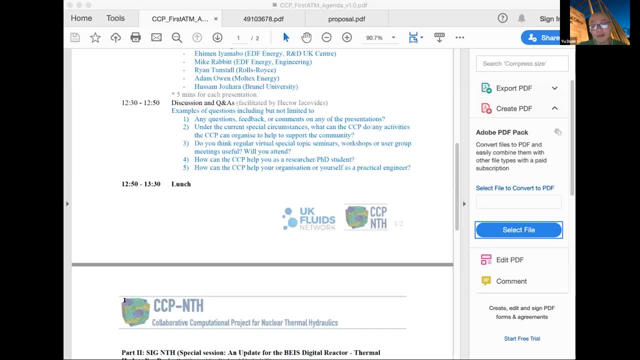 on this framework and I know a lot of people doing the benchmark cases here and there. but is that possible for the CCP to maintain the maintain a sharing database or sharing like a data bank for people or for the other users in the group to do the benchmark or some data analytics? 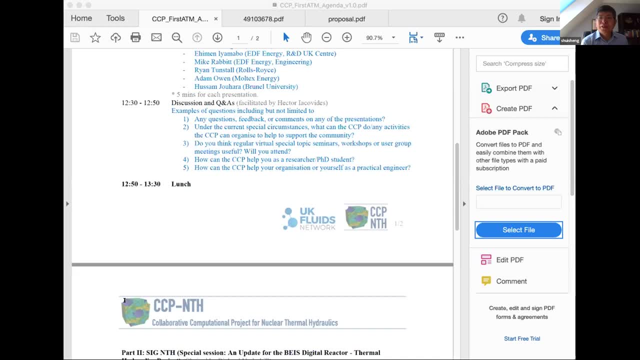 Right, I'll try to answer this and probably some others can come along later. Now you're right- and actually maintain the knowledge and data within the that has been created by the community and actually to make use of it later on is hugely important. 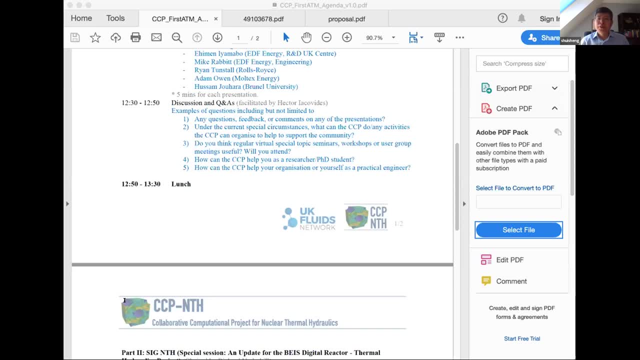 So you probably already seen on one of the slides, we said we'll use the website, the document, the database and also the- the publications generated by this community- and benchmarking is something we were hoping to organize through the years when we basically assess the needs. 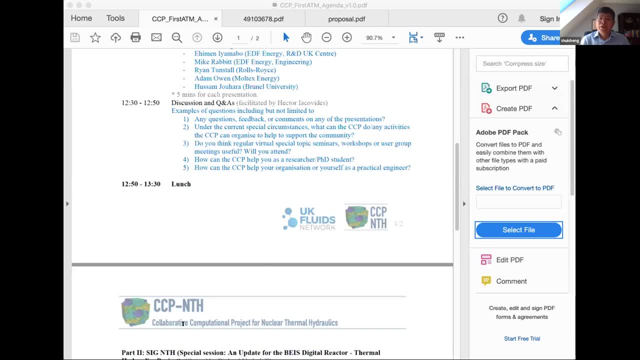 of the community and also the development of the country really, and then organize suitable benchmarking which are relevant to the time and the community. So obviously we open that to international users as well, but the main focus for us is to look at the codes. 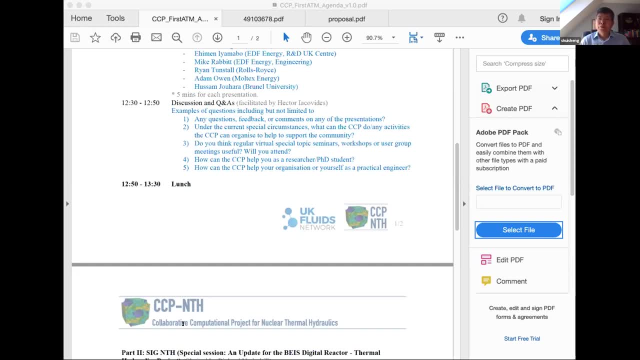 and methodology and the kind of particular records we want to look at, And so that people actually work together to share knowledge, and after that, archiving, as you say, is quite important. Another thing is about how to control the quality of the shared data. 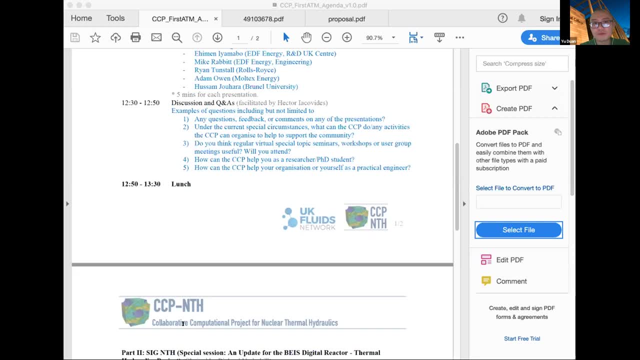 That is. I think that is probably very important, because if we say we're doing the benchmark and these environments kind of biased towards certain mistakes, towards something we cannot really support that, if we're just doing the comparison between the similar miracle and the experimental data, 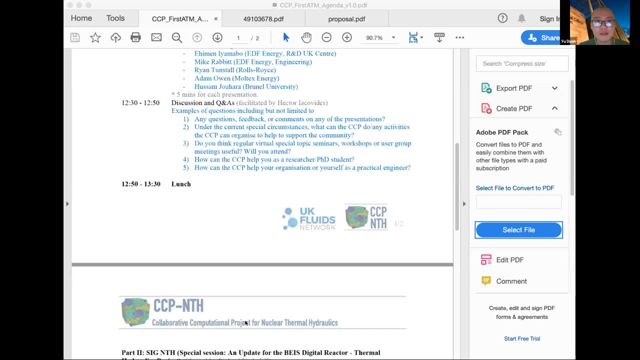 I think. is there any like? can we generate any guidelines about how to generate data? Anyone want to comment on that? Yes, Xu Sheng. Yes, please, Dominic Lawrence here. Maybe it's a bit philosophical, but I'm amazed about the rapid progress. 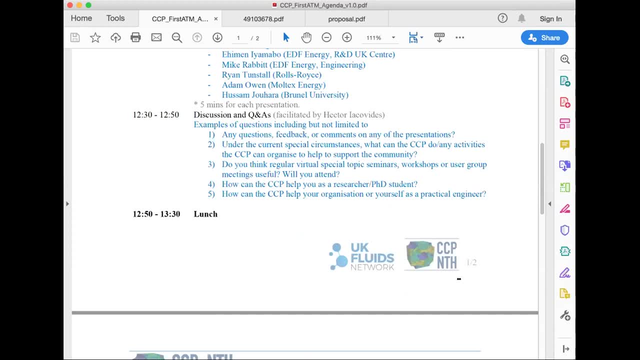 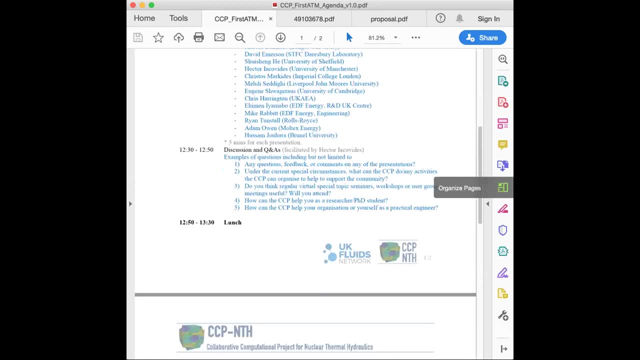 of DNS and what MISARI has been doing and EAMS et cetera. It's very interesting. Thank you, It's. I mean, there's no doubt about the quality when you're doing DNS with such a high resolution, And I find it a bit disappointing that so few people 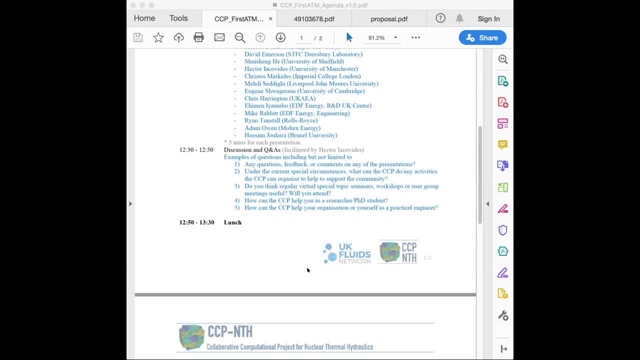 are actually interested in using other people's data. I think the first test cases that the NEC 5000 group shared was only used by the Dutch group and the Belgium group. I mean, there was a test case, I don't know if it's spiral wire. 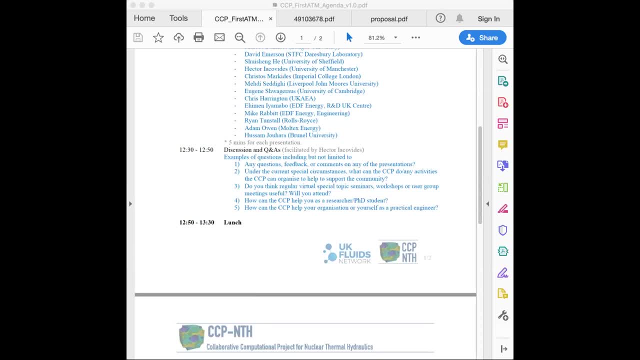 It's the same thing with the John Hopkins Turbid database. You know they have channel flow up to Reynolds 5000 now And it's so easy to use. I've been trying to get my PhD students to use it for over five. 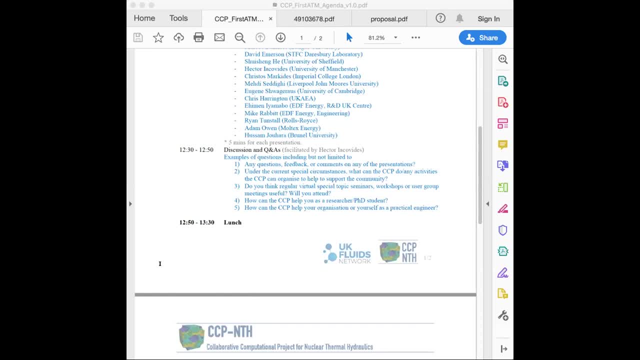 nearly 10 years now, But it seems all the PhD students are interested in is running their own little LES and little DNS. Nobody's interested in using somebody else's data And I find this really sad. I mean, We're not. we could make much more rapid progress. 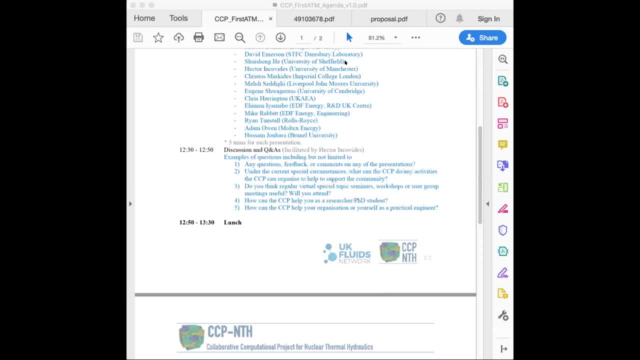 Why don't we? Why don't we participate? Missouri proposed another fantastic benchmark there. Why, Why is no one- So few people- interested in using some? you know these. The world is now completely global in every area, except maybe turbulence, modeling, research. 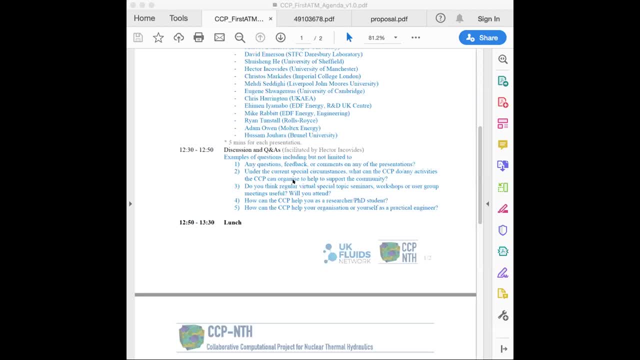 Okay, That's my philosophical statement, But Think global. now, you know, share globally, And we don't need everybody to to run their own little DNS, which will be obsolete in six months. Let's use this fantastic supercomputing power. 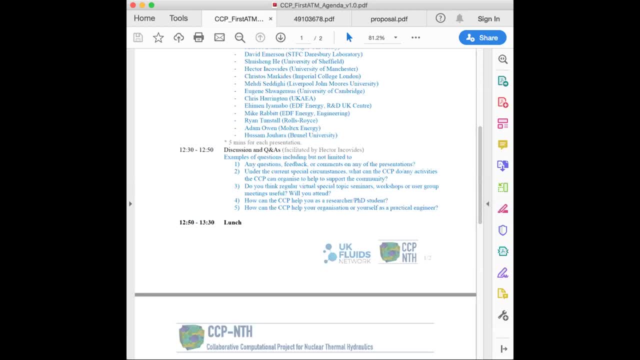 And and the fact that you know everything is open now. So that was my comment. Thank you, Right. And unless anyone else wants to comment on my personal view on this, it's just like I mean experiments that has been done over the history. 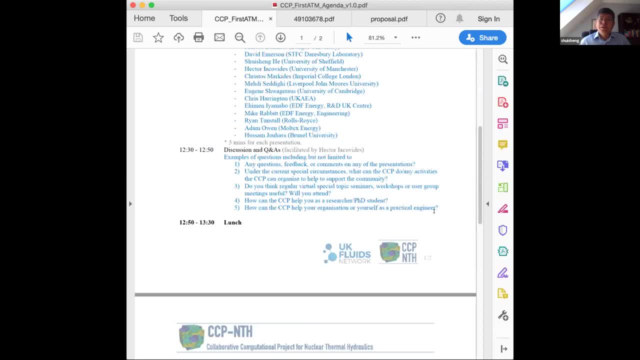 You, you, you wouldn't be able to generate All the experiments relevant to all designs In one place, In one go. So, like experiment, I think there are are going to be a lot of research In the High fidelity. 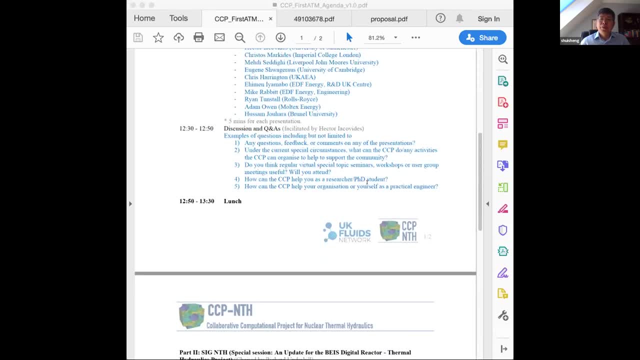 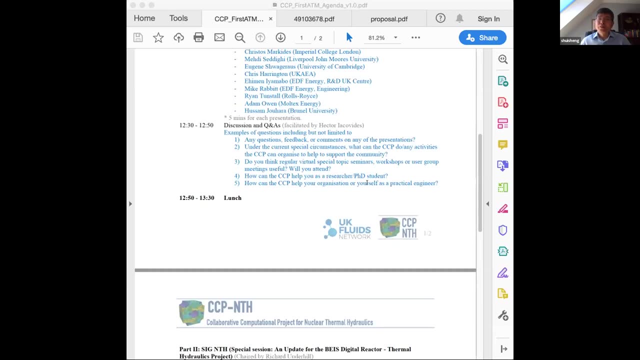 Simulations to tackle their particular problems And the the the rock bundle test case generated by By through the names System. I agree with you: That was hugely Inspiring. I don't think it's just a Dutch People have used, I know they have. 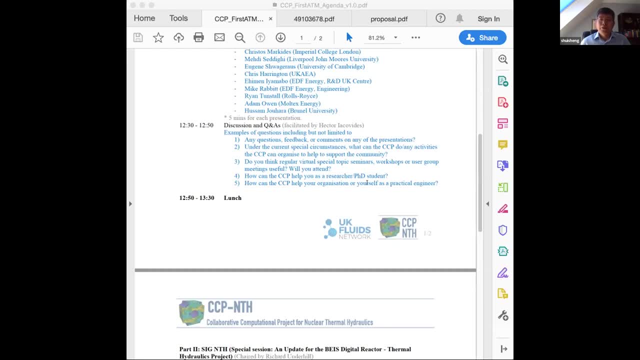 It's through the European project, Projects that actually have a particular Branch of their work to collaborate with needs program And have done some Validations. I know other groups are doing similar things, But not What do they Published The same with John Hopkins. 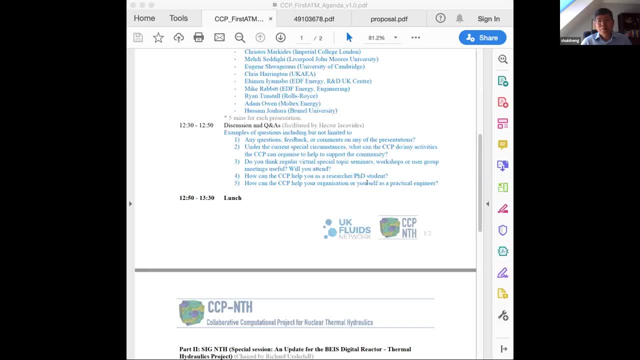 Like Database, Often those are used For validation. We In our group which we use that For validation For our simulations. But Remember Those are very limited To Certain. You know geometries and certain violence numbers. 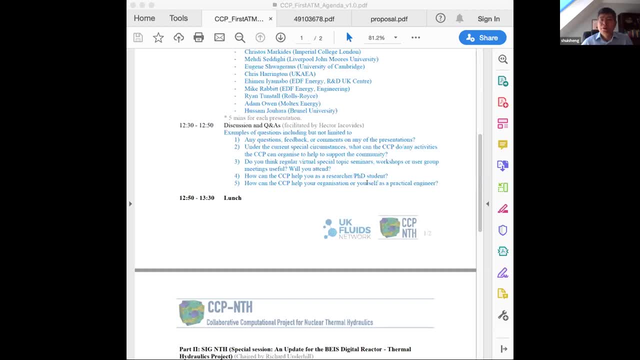 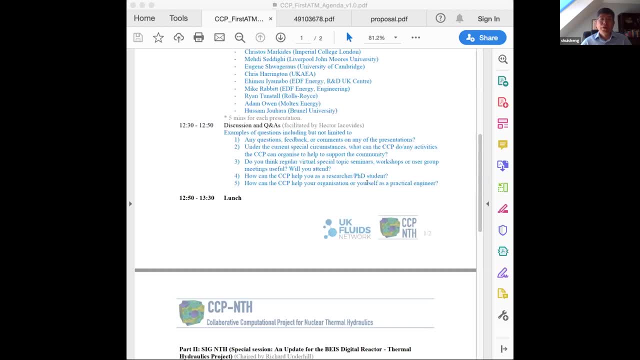 You know. You know The Structure and the Detroit's Kind of software is is is Important. I think the analogy that should Shane makes between validation experiments And the high fidelity simulations is a good one, because If you look at people like the guidance from over campus, 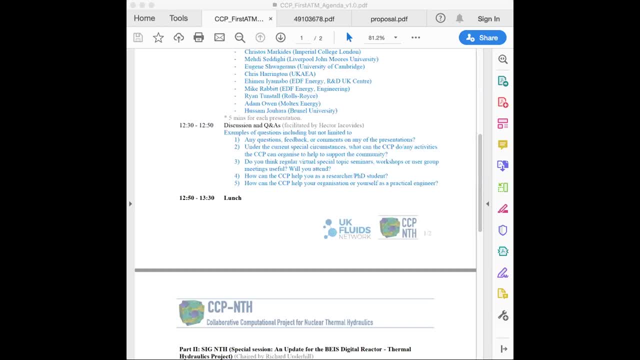 over campus. The validation experiment should be designed alongside the analysis It's intended to support. there needs to be push and pull, so if you have a problem to solve and you think you can address it with high fidelity simulation, you probably need to then kind of pull the. 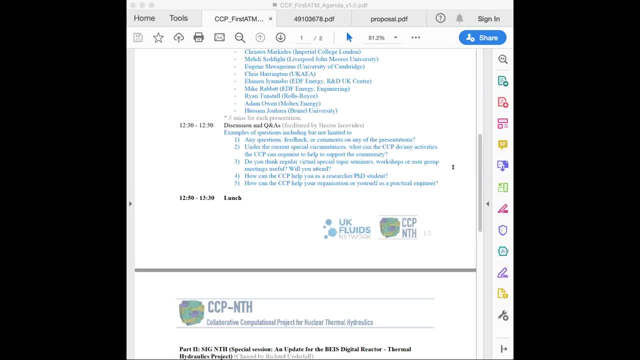 high fidelity into that regime and that domain, rather than it being the high fidelity work being done on simple cases and it being pushed towards who could possibly use it. I think there definitely needs to be an iterative requirement setting and satisfaction in that loop. I'd echo what Graham said there. 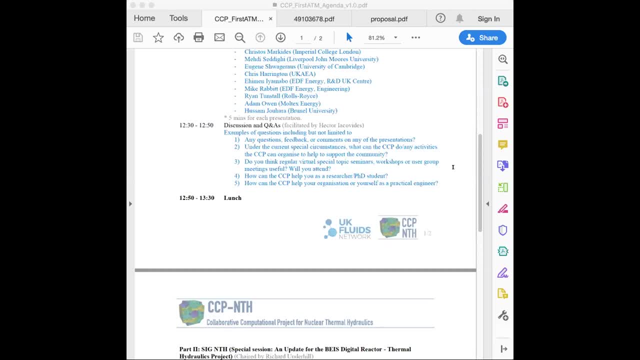 from our perspective. I think that's very well put. I think there's also some challenges in terms of industry people trying to sort of back up their own work using high fidelity simulations at the minute, in terms of just getting regulators and the like on board with the fact that a DNS 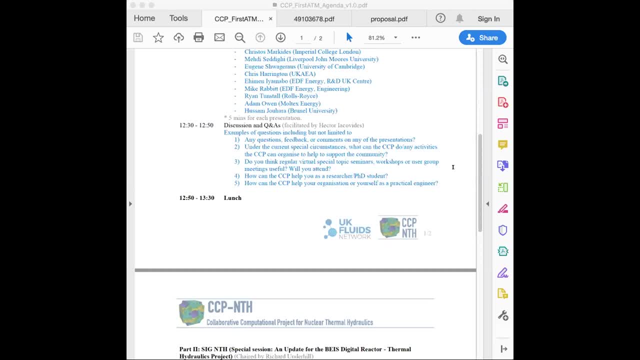 can be as good a benchmark as an experiment. Let me say something here. It connects to what Ryan was asking, And so I just want to make clear that I mean. the reason we perform these large-scale simulations is not just for fun. 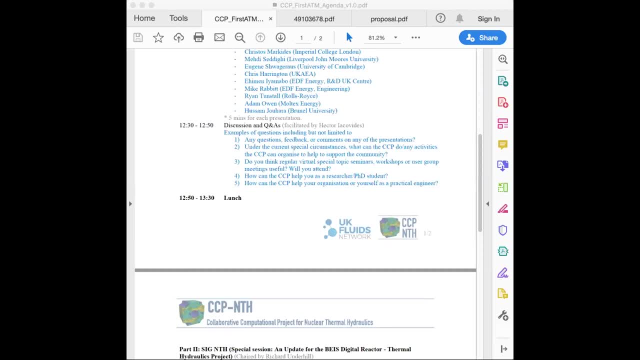 So, for instance, some of those large pebble bed cases you're seeing, they are being performed to really because we there is a driver now to improve porous media models for pebble beds And that's one of the reasons we're performing this. 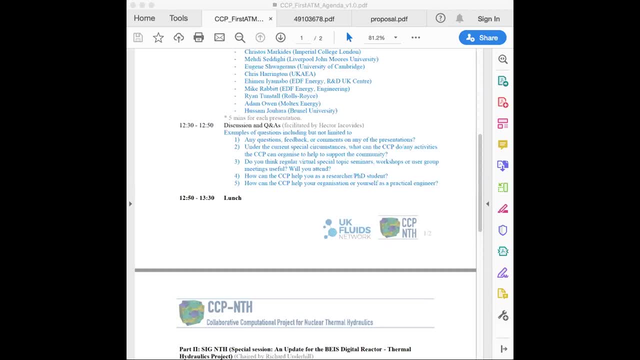 So to use the full multi-scale stack, going from these DNS calculations, LES calculations, improve RANS models for these particular geometries, which is very challenging, And then go to the, to the improved porous media models, That's. that's sort of like the. 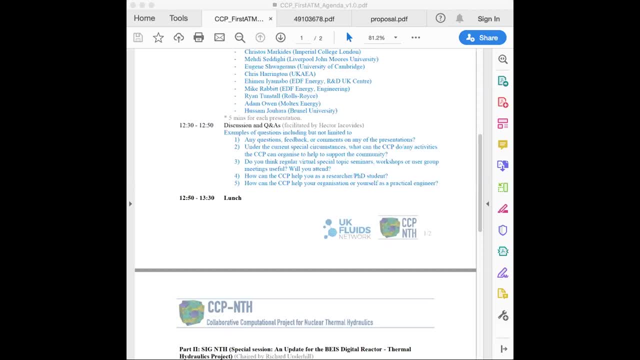 the usage of these calculations. So I would agree that, in general, these calculations need to be, need to be tied to a need, and- and it is an iterative process- I mean you do need more of those. At the same time, though, I 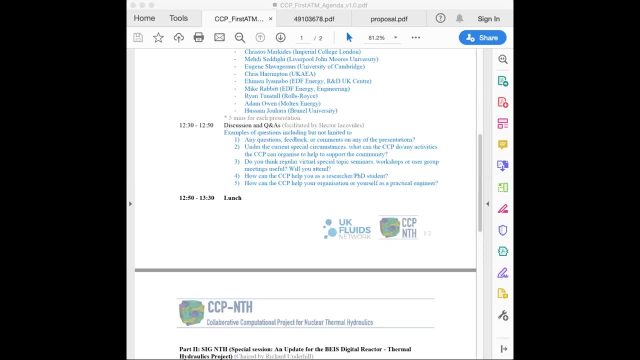 I do sympathize with the spirit of the comment of Dominic, because we do need more, I would say more- usage of each other's data and act more as a community. I'm not talking just nationally, but internationally too, so that the and I- I was hoping that some of 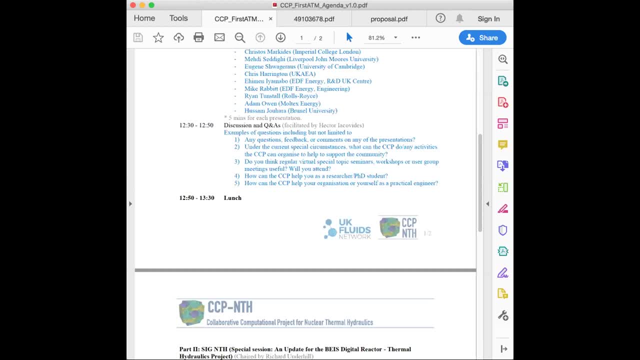 these NEA benchmarks would help. I think we need in any benchmarks built around DNS data. that's all we need. I think that would be something that can help getting getting this data used. and can I just say part of- I think it's part of the issue here- what the regulator sort of wants. there's the scientific question of 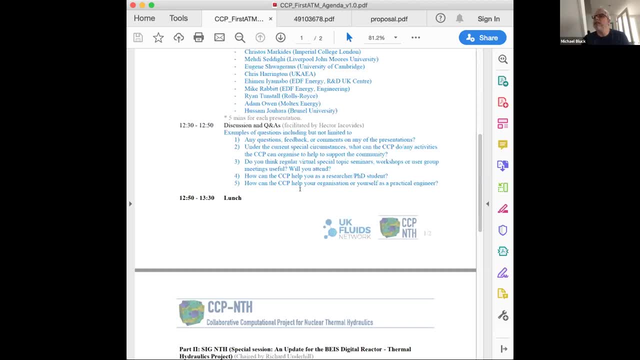 using DNS as a means to validate other method- be rams, alias or whatever that can subsequently be be used on things, but certainly in the UK the the desire to use it for thermal hydraulics and nuclear is is in large part driven by what the regulator wants and what the regulator trusts, and particularly in 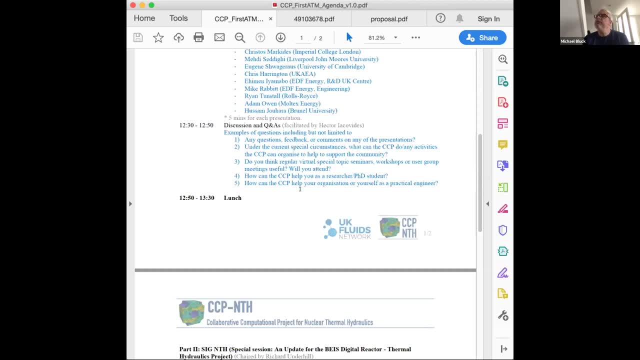 regard to the use of the data that's being used in the UK and in particular to sort of accident scenarios and and- and I think regulator would say for good reason there that benchmarks or all well and good, but there is not necessarily a big part of the jigsaw. but I'm just suggesting that's maybe why we don't. 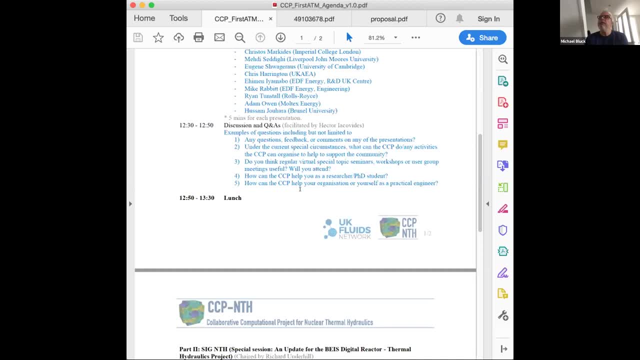 make as much use of them as I would agree we should. yes, can I just comment? I would agree we should. yes, can I just comment? I would agree we should. I would agree we should. I would agree we should. I was interviewed by think tank from the was interviewed by think tank from the EU Commission who was asking who was. 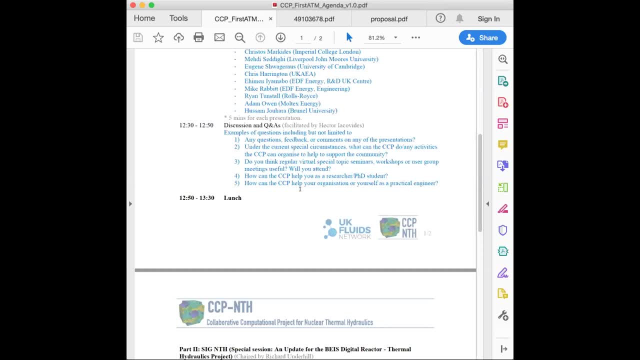 EU Commission who was asking, who was noting that there's a lot of enormous noting that there's a lot of enormous collaboration going on in structure collaboration going on in structure, mechanics in materials etc. and their mechanics in materials etc. and their question was: why? why is research in CFD? 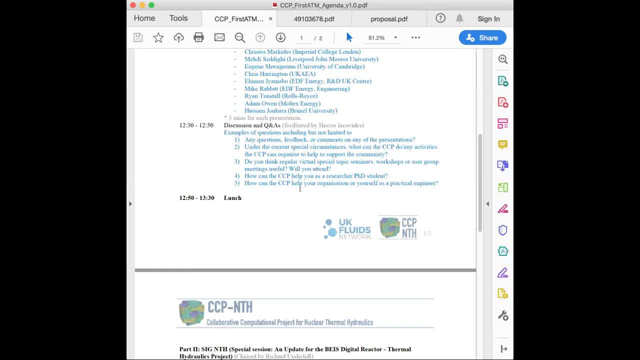 question was: why? why is research in CFD internalist modeling so fragmented? why internalist modeling so fragmented? why are they receiving all these proposals? are they receiving all these proposals from different, different teams, etc. why from different, different teams, etc. why is there not more collaboration? that was 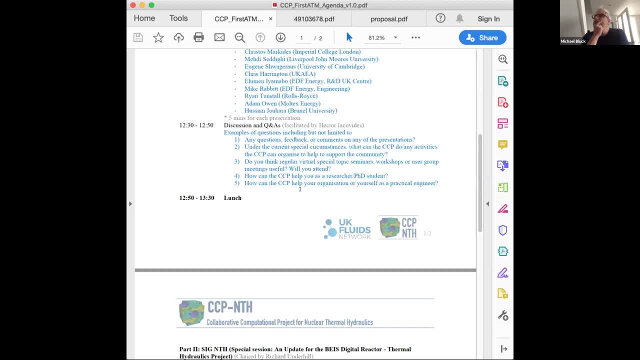 is there not more collaboration? that was many years ago and it seems it hasn't many years ago and it seems it hasn't really many years ago and it seems it hasn't really little progress and there's so much, really little progress and there's so much. 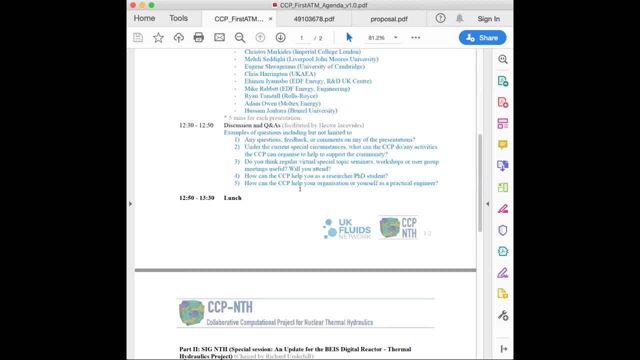 really little progress and there's so much to be done nowadays, just to you know to be done nowadays, just to you know to be done nowadays, just to you know, if we conjugate heat transfer liquid metal, if we conjugate heat transfer liquid metal, if we conjugate heat transfer liquid metal either, there's so much progress we. 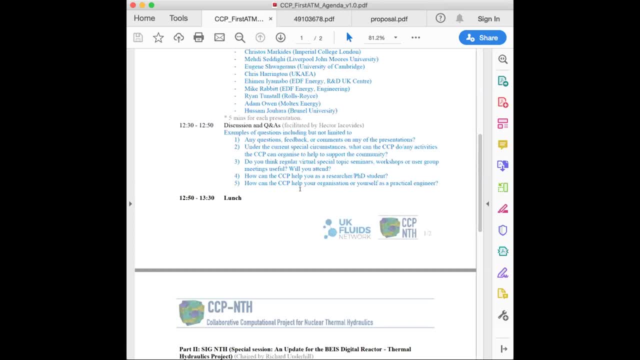 either there's so much progress we, either there's so much progress we could make if, as I said, instead of everyone could make. if, as I said, instead of everyone could make, if, as I said, instead of everyone running his own little DNS in his, running his own little DNS in his. 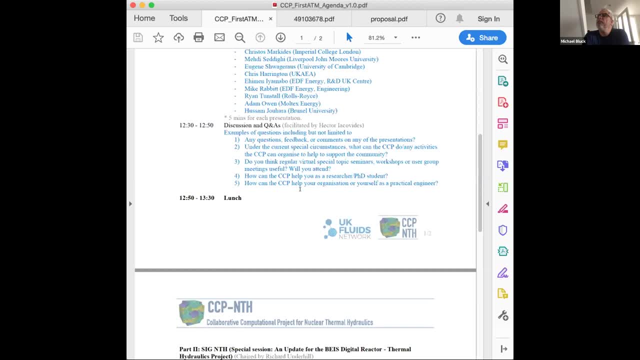 running his own little DNS in his corner. if it was a really truly global corner. if it was a really truly global corner, if it was a really truly global approach to it. we're seeing global approach to it. we're seeing global approach to it. we're seeing global collaborations in many areas. Cove it. 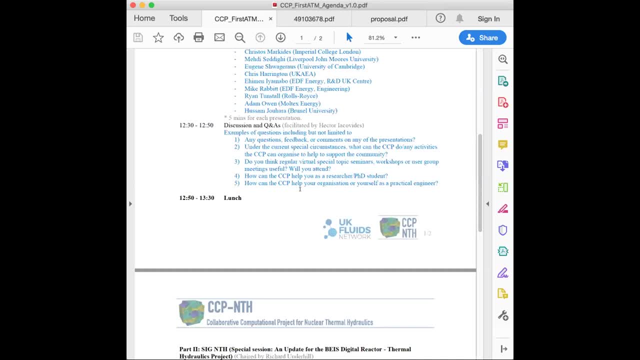 collaborations in many areas, Cove it, collaborations in many areas, Cove it, etc. and John Hopkins, and it's just not, etc. and John Hopkins and it's just not, etc. and John Hopkins, and it's just not happening and happening in the sea of the happening and happening in the sea of the. 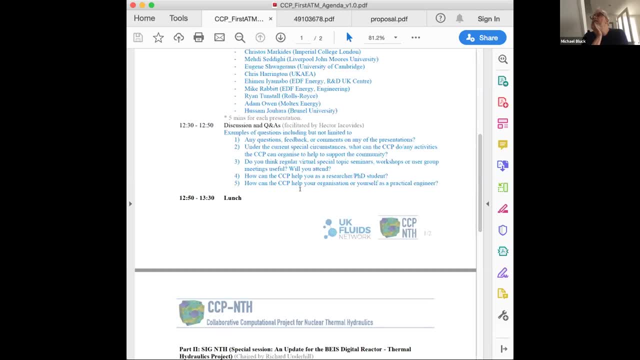 happening and happening in the sea of the intelligence model community. I think intelligence model community. I think intelligence model community. I think to the problem is so hard. everyone thinks to the problem is so hard. everyone thinks to the problem is so hard everyone thinks he can make a little dent, you know. 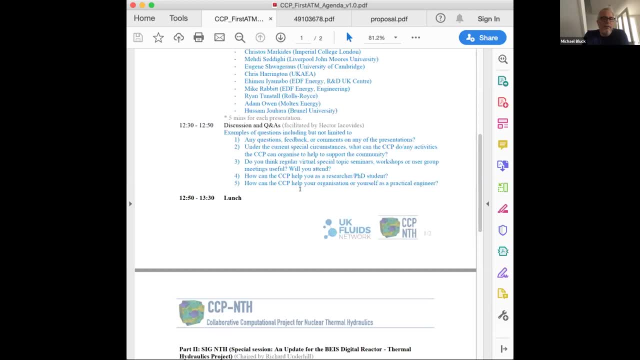 he can make a little dent. you know he can make a little dent, you know. wants to have a go at it? yes, all right. wants to have a go at it? yes, all right. wants to have a go at it? yes, all right, Steve. Steve Graham here from the. 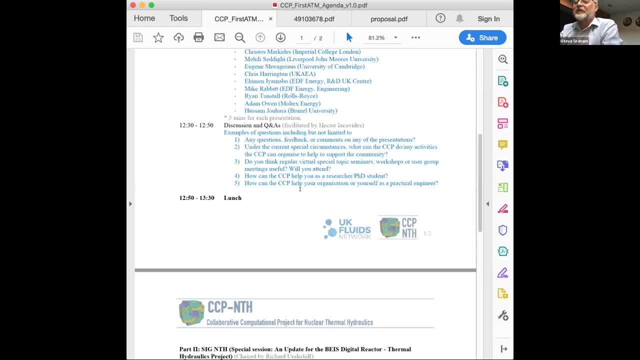 Steve Steve Graham here from the Steve Steve Graham here from the National Nuclear Laboratory. I just like National Nuclear Laboratory, I just like National Nuclear Laboratory. I just like to reflect on what Mike said and also to reflect on what Mike said and also to reflect on what Mike said and also what Dominique said is as well. I mean, I 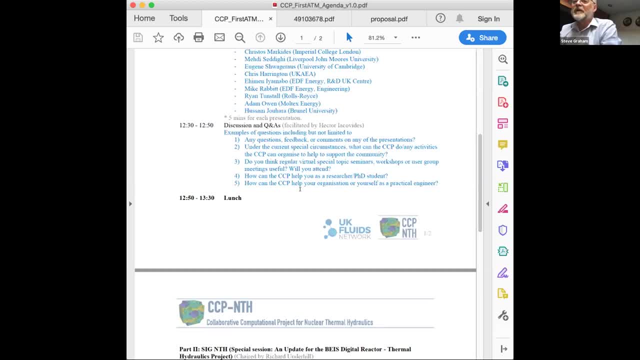 what Dominique said is as well, I mean I what Dominique said is as well, I mean I think they both have a valid point to think. they both have a valid point to think. they both have a valid point to make. I think, from experience speaking to. make. I think, from experience speaking to make. I think, from experience speaking to the regulator's, I think the issue we the regulator's, I think the issue we the regulator's, I think the issue we have that there's some really great have that there's some really great. 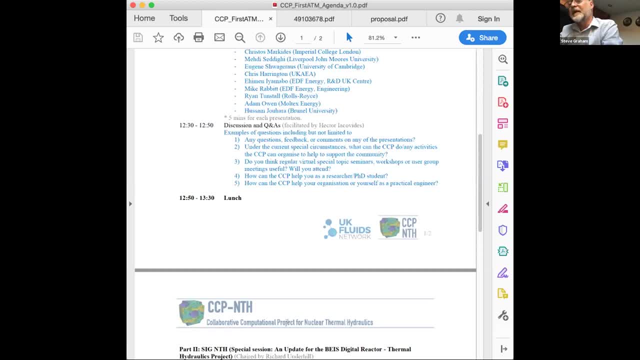 have that. there's some really great fundamental stuff that's being done in fundamental stuff. that's being done in fundamental stuff. that's being done in in the DNS and the LES arena, at the in the DNS and the LES arena, at the in the DNS and the LES arena at the moment. but it is quite a long way. 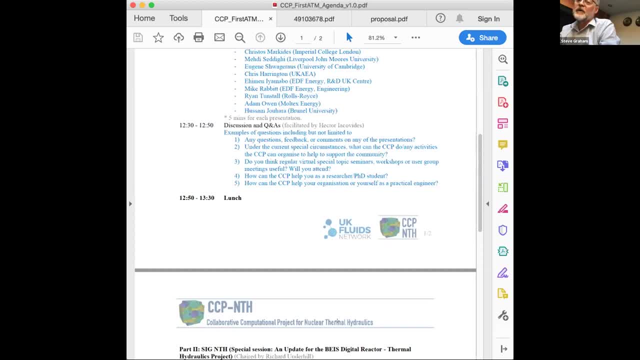 moment, but it is quite a long way moment, but it is quite a long way removed from the actual applications, removed from the actual applications, removed from the actual applications. quite often that we faced with defending, quite often that we faced with defending, quite often that we faced with defending in front of the regulator, and I think 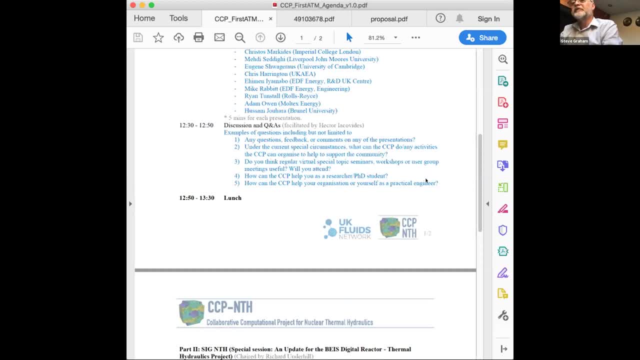 in front of the regulator and, I think, in front of the regulator, and I think it's how we make that journey. it's how we make that journey, it's how we make that journey collectively, from the research to the collectively, from the research to the collectively, from the research to the position where people who actually use 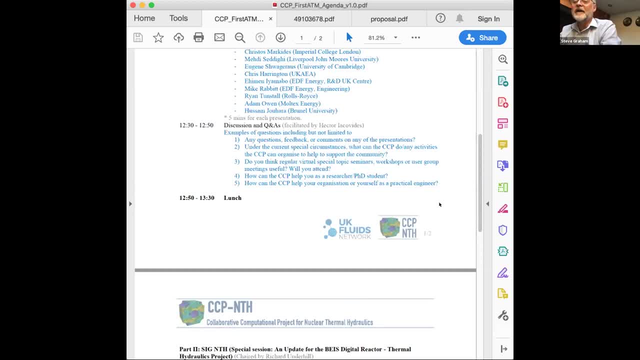 position where people who actually use, position where people who actually use the codes in industry to input to safety, the codes in industry to input to safety cases, actually make it count and I cases actually make it count and I cases actually make it count and I think it's a very valid point that Mike. 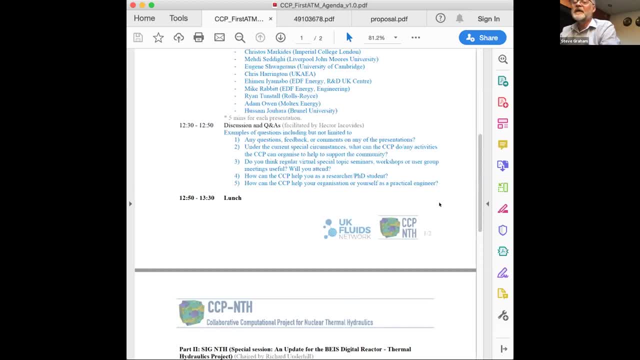 think it's a very valid point that Mike think it's a very valid point that Mike made, and it's all about how we actually made, and it's all about how we actually made and it's all about how we actually do this. now it may be that we just need 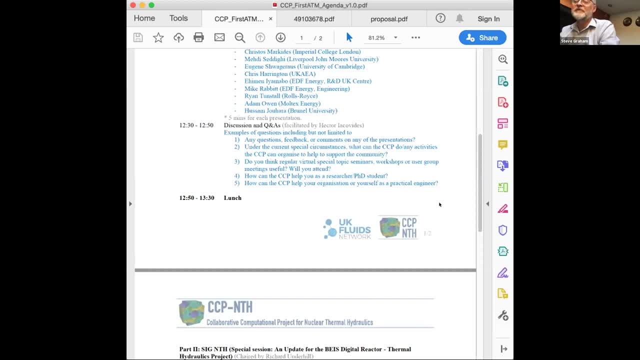 do this now. it may be that we just need do this now. it may be that we just need to be better at defending the position. to be better at defending the position. to be better at defending the position, the technical position in front of the, the technical position in front of the. 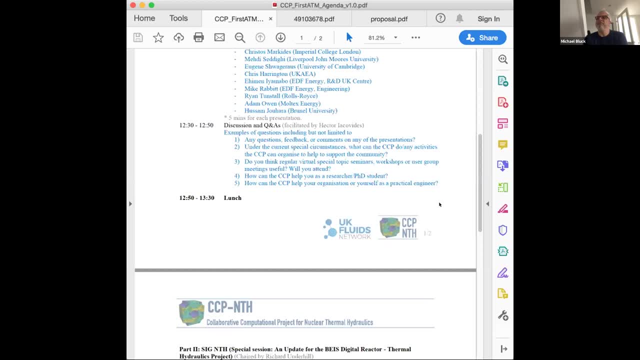 the technical position in front of the regulator, and we just don't seem to be regulator and we just don't seem to be regulator and we just don't seem to be able to give this the sort of you know, able to give this the sort of you know. able to give this the sort of, you know, the input that it that it needs it. may the input that it that it needs it. may the input that it that it needs it may be quite simple at the end of the day, be quite simple at the end of the day. 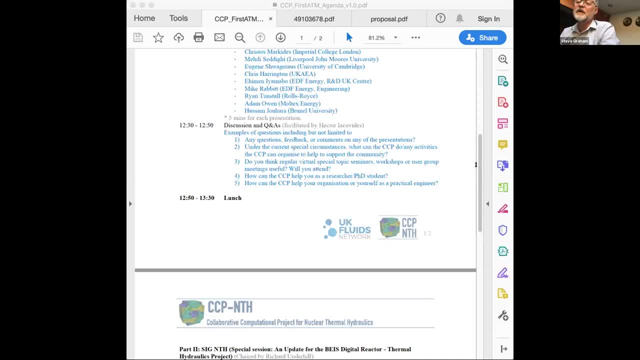 be quite simple at the end of the day, but we perhaps it's the way we tell the but we perhaps it's the way we tell the but we perhaps it's the way we tell the story and the way we bring all these story and the way we bring all these. 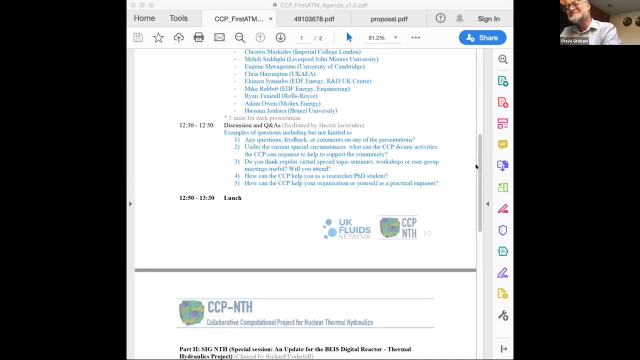 story and the way we bring all these very good concepts together. I don't know very good concepts together. I don't know very good concepts together, I don't know. yeah, I'd agree, I agree as well, Steve I. yeah, I'd agree, I agree as well, Steve I. 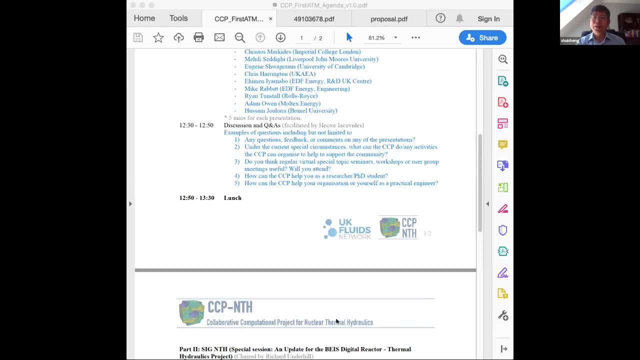 yeah, I'd agree. I agree as well, Steve. I think that's a very important point and think that's a very important point. and think that's a very important point and I wonder whether I wonder whether my. I wonder whether I wonder whether my I wonder whether I wonder whether my coverage is still around online, I know. 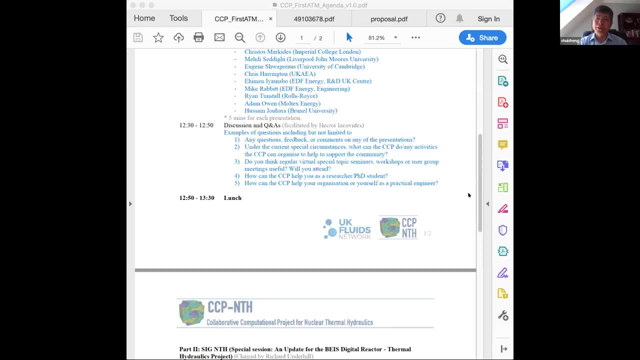 coverage is still around online. I know coverage is still around online. I know that they they try to support at least that they. they try to support at least that they. they try to support at least some of their safety cases with safety, some of their safety cases with safety. 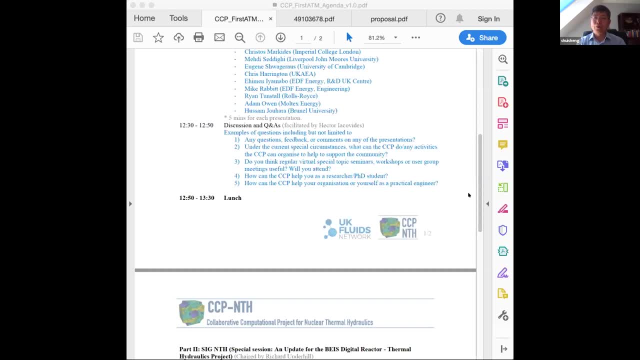 some of their safety cases with safety simulations and I I'm from what well I simulations and I I'm from what well I simulations and I I'm from what well I can see and they had to put a lot of can see and they had to put a lot of. 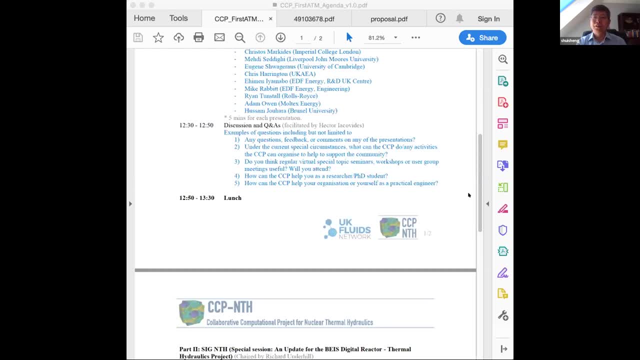 can see, and they had to put a lot of effort to justify their, their, their effort to justify their, their, their effort to justify their, their, their means. you know the method that you use means. you know the method that you use means. you know the method that you use even though, generally speaking, we proceed. 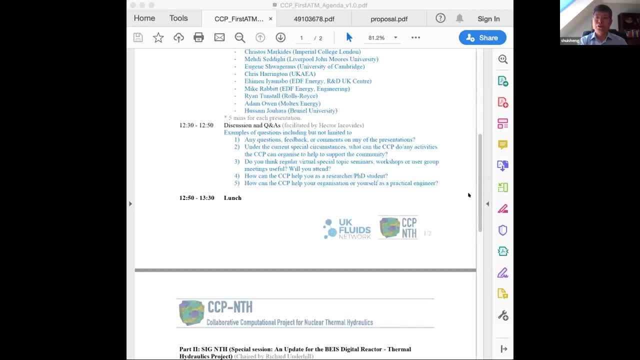 even though, generally speaking, we proceed. even though, generally speaking, we proceed. they are the method they've used. are they are the method they've used? are they are the method they've used, are quite mature and think that you, they be quite mature and think that you, they be. 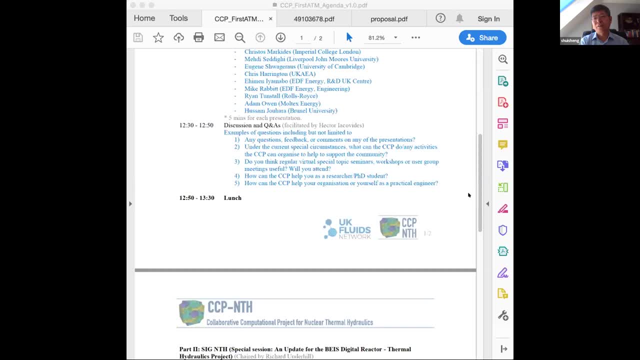 quite mature and think that you, they be a kind of validation, they put together a kind of validation. they put together a kind of validation. they put together seems to be quite sound. but I believe seems to be quite sound, but I believe seems to be quite sound, but I believe that you put a lot of effort, for I mean 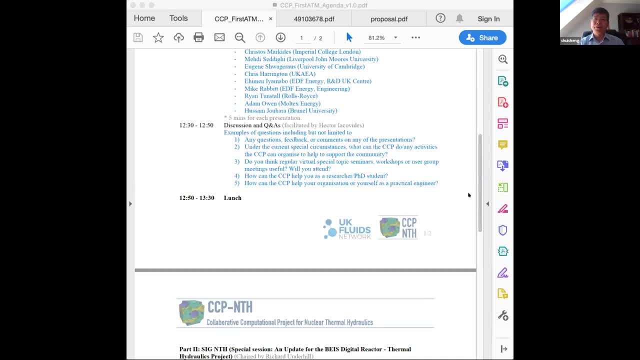 that you put a lot of effort for. I mean that you put a lot of effort for I mean it's basically a case-by-case, rather, it's basically a case-by-case. rather, it's basically a case-by-case, rather than say those are good for indeed. 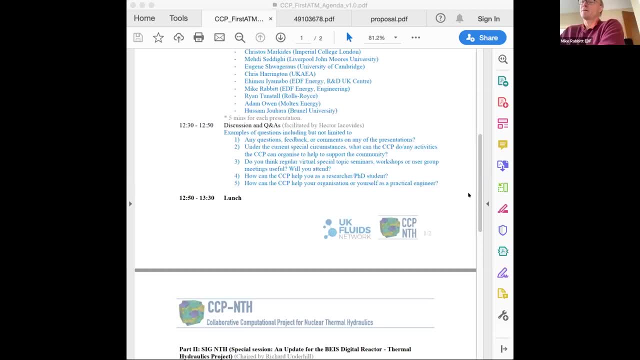 than say those are good for, indeed, than say those are good for, indeed, indeed, yes, I am here. yeah, I think when, indeed, yes, I am here. yeah, I think when, indeed, yes, I am here. yeah, I think, when you're trying to present to the regulator, you're trying to present to the regulator. 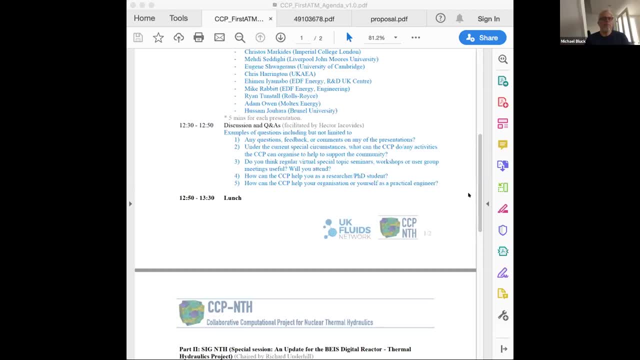 you're trying to present to the regulator. you have to put their hats on yes and you have to put their hats on yes and you have to put their hats on yes and ask the questions they would ask you and ask the questions they would ask you, and. 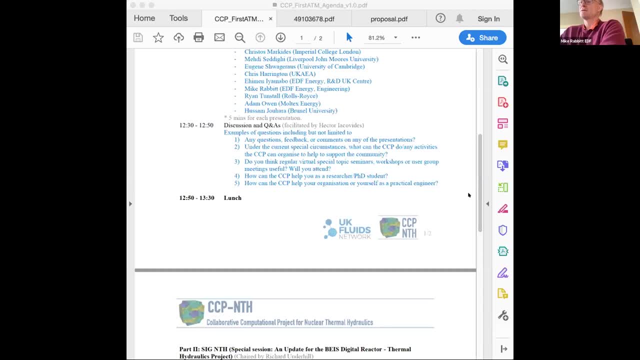 ask the questions they would ask you, and you know because that they're very, you know because that they're very, you know because that they're very reasonable people actually. so it's not reasonable people actually. so it's not reasonable people actually. so it's not good thing to base your safety case on. 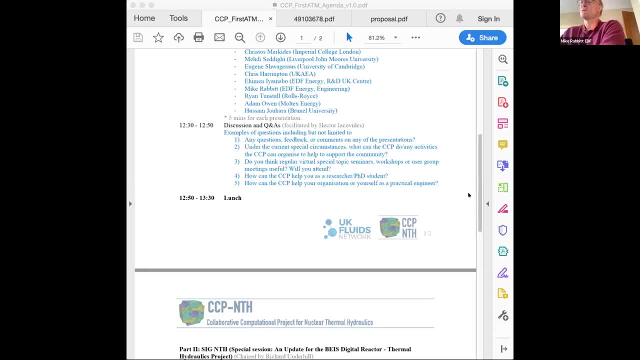 good thing to base your safety case on. good thing to base your safety case on CFD calculation on its own. you have to CFD calculation on its own. you have to CFD calculation on its own. you have to present a safety case which has more. present a safety case which has more. 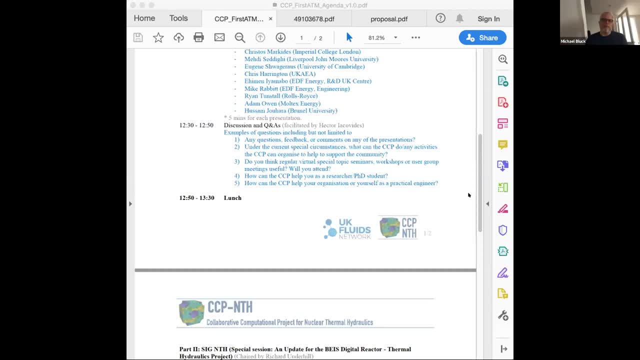 present a safety case which has more than one leg- most definitely yeah, and than one leg most definitely yeah, and than one leg most definitely yeah. and, for example, we've gone to a lot of, for example, we've gone to a lot of, for example, we've gone to a lot of efforts to put thermocouples in reactors. 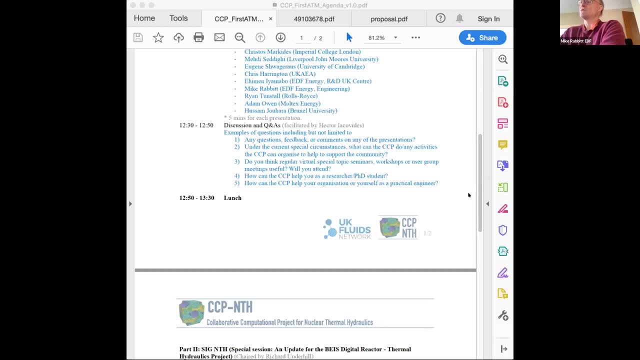 efforts to put thermocouples in reactors, efforts to put thermocouples in reactors, for example. to essentially validate what, for example? to essentially validate what, for example, to essentially validate what you're doing. so it's validation is the you're doing, so it's validation is the. 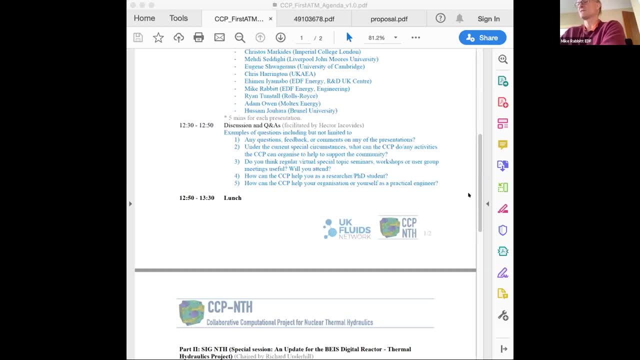 you're doing. so it's validation is the key question that we would answer, we key question that we would answer. we key question that we would answer, we would ask, and that is the question the would ask, and that is the question the would ask and that is the question the regulator asks. so you have to, instead of 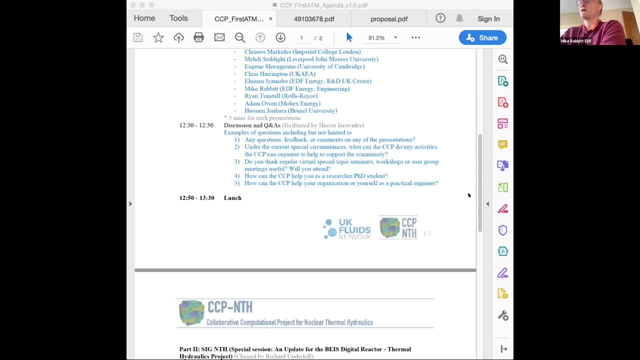 regulator asks, so you have to. instead of regulator asks, so you have to, instead of presenting a safety case. you know it's presenting a safety case. you know it's presenting a safety case. you know it's not going to fly. you have to work hard. not going to fly, you have to work hard. 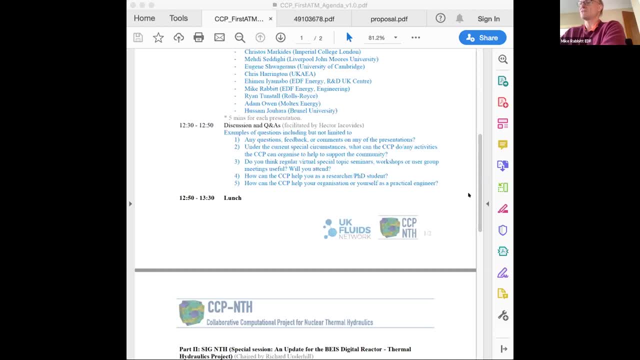 not going to fly. you have to work hard before actually presenting it, and that before actually presenting it, and that before actually presenting it, and that that's the basis of what you have to try. that's the basis of what you have to try. that's the basis of what you have to try to achieve. 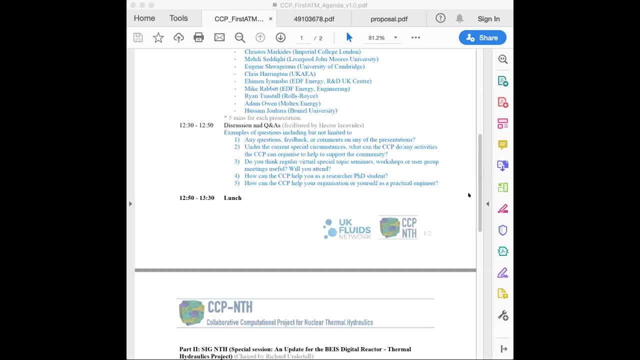 to achieve, to achieve. but mike thermocouples in liquid lead, but mike thermocouples in liquid lead, but mike thermocouples in liquid lead is going to be very hard, is going to be very hard, is going to be very hard. yeah, um yeah, we don't have any of those. 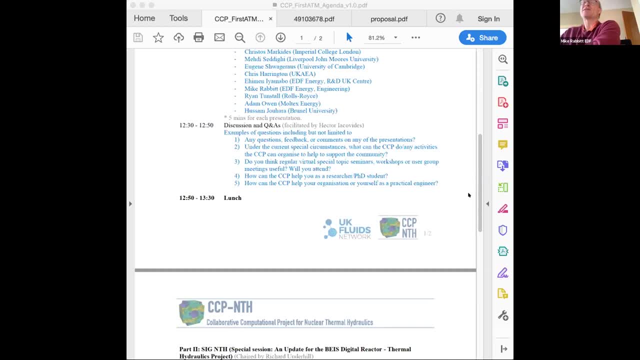 yeah, um yeah, we don't have any of those. yeah, um yeah, we don't have any of those. directors, so directors, so directors. so it's not straightforward either. putting it's not straightforward either. putting it's not straightforward either putting thermocouples in gas. core directors: i. 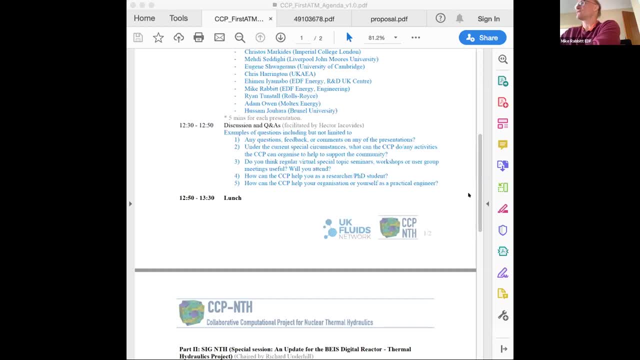 thermocouples in gas core directors. i. thermocouples in gas core directors. i mean they're mean. they're mean they're fairly hot and high pressure. so no, it's fairly hot and high pressure. so no, it's fairly hot and high pressure. so no, it's not straightforward by any means, but so. 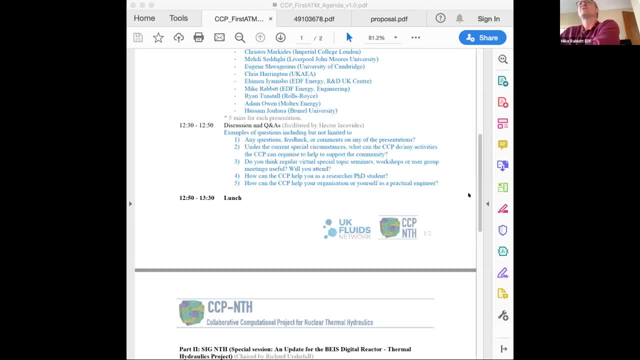 not straightforward by any means. but so not straightforward by any means, but so it comes down to what somebody said. it comes down to what somebody said. it comes down to what somebody said earlier about designing earlier, about designing earlier, about designing before you know designing your reactors, before you know designing your reactors. 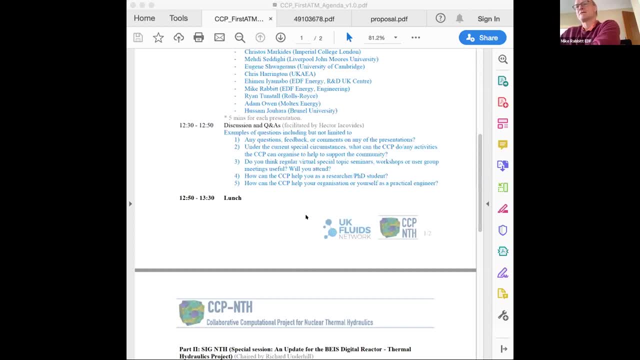 before you know, designing your reactors even up front to to put some good even up front to, to put some good even up front to to put some good information, information, information to get your analysts, but the kinds of to get your analysts, but the kinds of to get your analysts, but the kinds of um challenges that we have on validation. 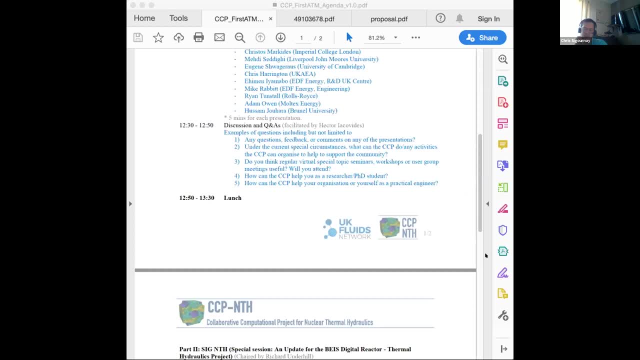 um challenges that we have on validation? um challenges that we have on validation uh associated with the models that we uh associated with the models that we uh associated with the models that we use in our safety cases. they're not use in our safety cases. they're not. 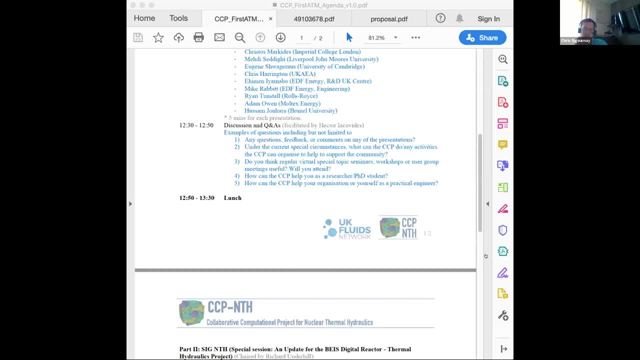 use in our safety cases. they're not the kind kinds of problems generally that, the kind kinds of problems generally that you would be able to underpin by you would be able to underpin by. you would be able to underpin by saying: well, here's a. 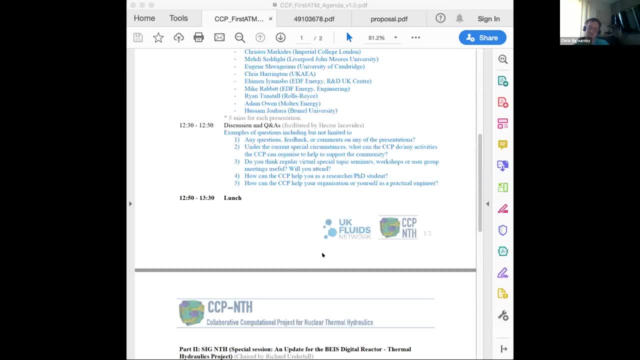 saying: well, here's a saying: well, here's a. here's a dns case of running a reynolds. here's a dns case of running a reynolds. here's a dns case of running a reynolds. number of 5 000 of a. 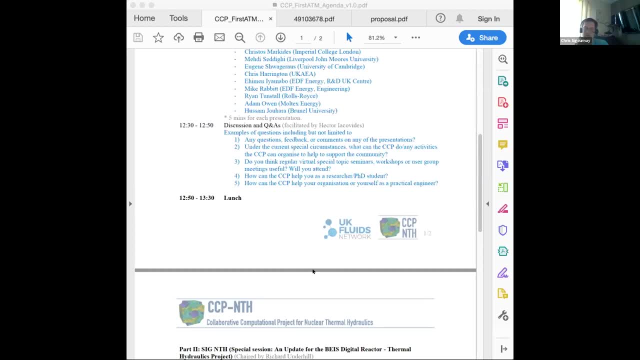 number of 5 000 of a number of 5 000 of a simple channel flow. uh, they're very simple channel flow. uh, they're very simple channel flow. uh, they're very complicated geometries with lots of complicated geometries, with lots of complicated geometries with lots of- um, rather esoteric features, and those are 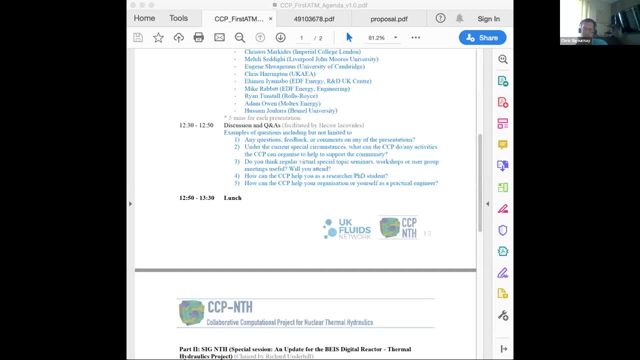 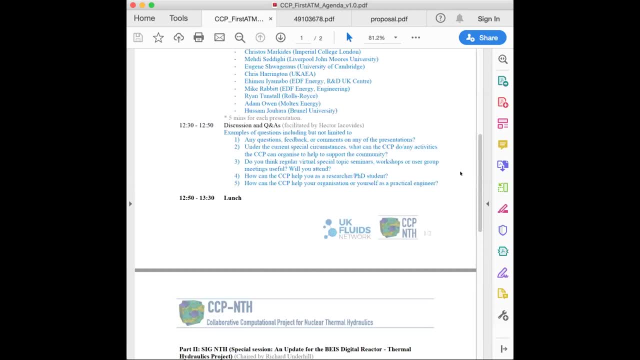 sorry when i said five thousand. that's sorry when i said five thousand. that's a turbulent reynolds number, a turbulent reynolds number, a turbulent reynolds number. okay, based on new star. so that's about. okay, based on new star, so that's about. 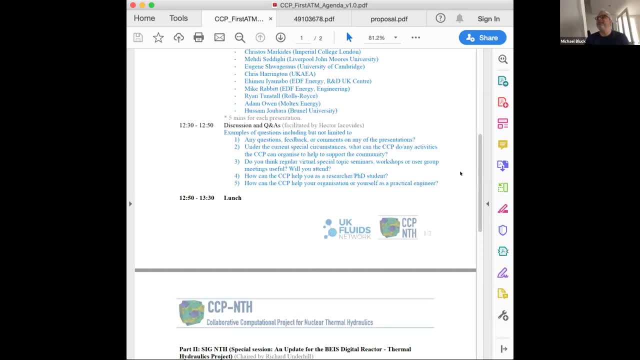 okay, based on new star. so that's about fifty thousand or something. it's still fifty thousand or something. it's still fifty thousand or something, it's still. it's still still okay. um now, i mean that was interesting. okay, um now, i mean that was interesting, okay. um now, i mean that was interesting discussion. obviously we haven't finished. 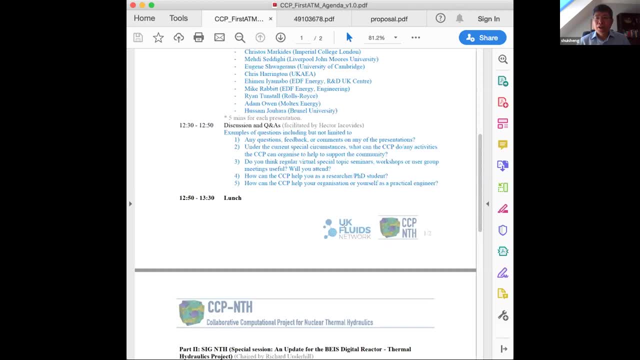 discussion. obviously we haven't finished discussion. obviously we haven't finished. uh, we can't finish this just today. so, uh, we can't finish this just today. so, uh, we can't finish this just today. so, uh, hopefully, uh, ccp would be a, uh a. uh, ccp would be a, uh a. 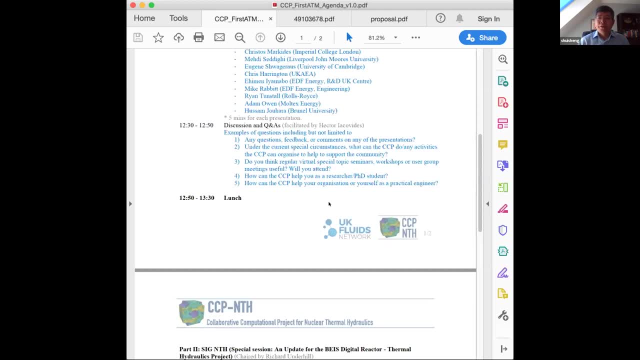 uh, ccp would be a? uh, a forum for for this kind of discussion forum, for for this kind of discussion forum, for for this kind of discussion and, as also said, we will try to use the and, as also said, we will try to use the and, as also said, we will try to use the website. 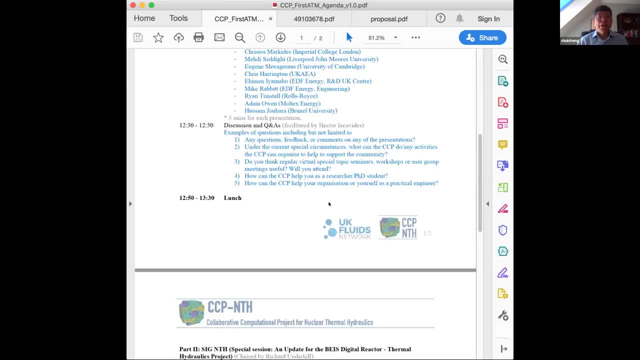 website. website to document, and, and, to document, and, and to document, and, and. so keep some of the progress you know. so keep some of the progress you know, so keep some of the progress you know. joint effort together so that we can. joint effort together so that we can. joint effort together so that we can actually move forward, actually move forward. 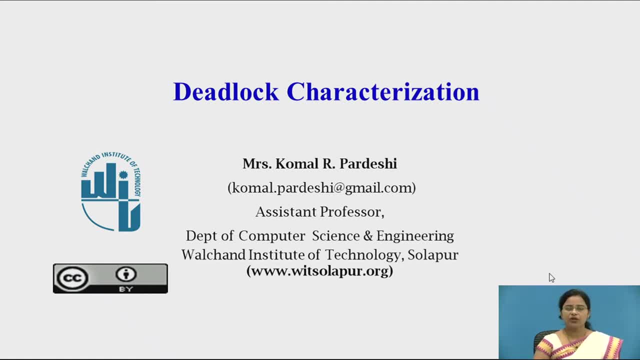 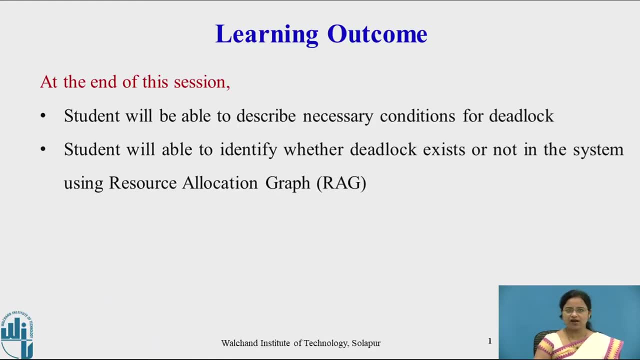 Hello everyone. Now we are going to learn about deadlock characterization, So the learning outcome of this session are: at the end of this session, student will be able to describe necessary conditions for deadlock and student will be able to identify whether deadlock exist or not in the system using resource allocation graph. Now, as in previous video,